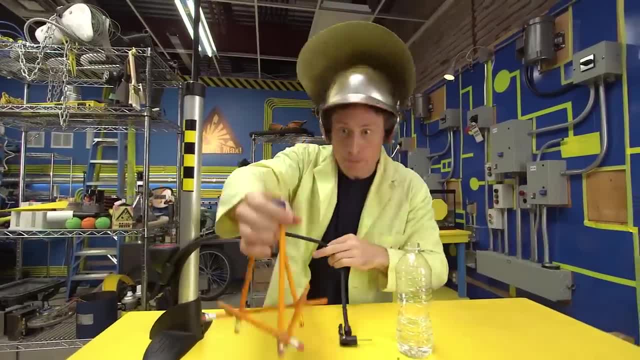 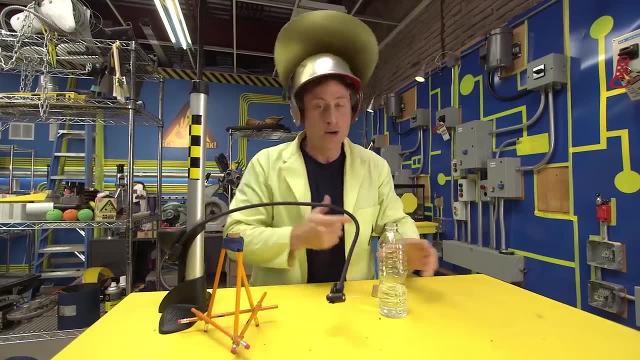 Take your cork and put it in a tripod launcher. You can make this out of pencils or anything you want, as long as it stands up nice and solidly. And then, of course, you want to decorate your bottle so it looks like a rocket. 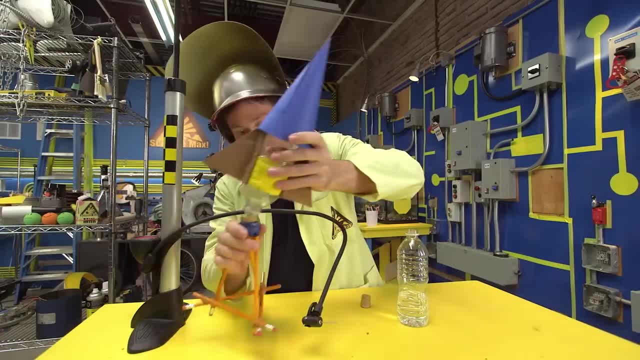 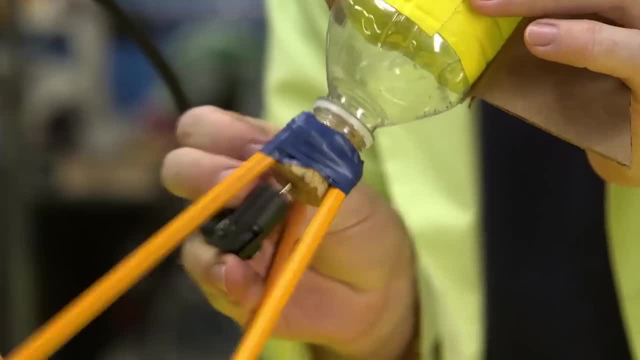 This is my rocket. Pretty good, right. So stick the bottle on the cork like before, like that, and then you stick the pin in the bottom, And what we're going to do is we're going to inflate the bottle with air pressure. 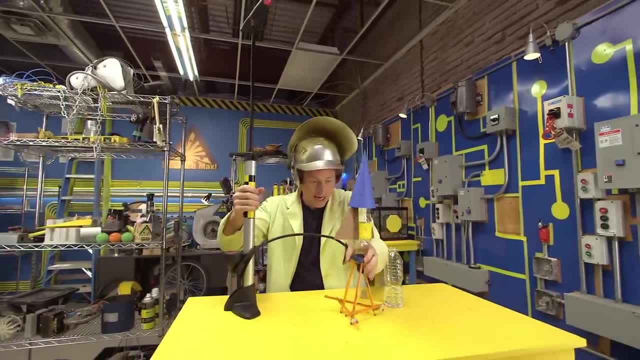 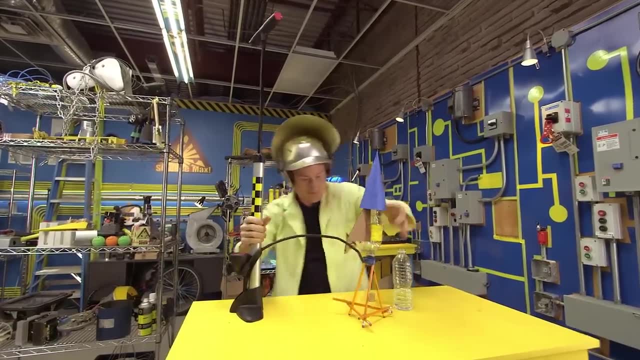 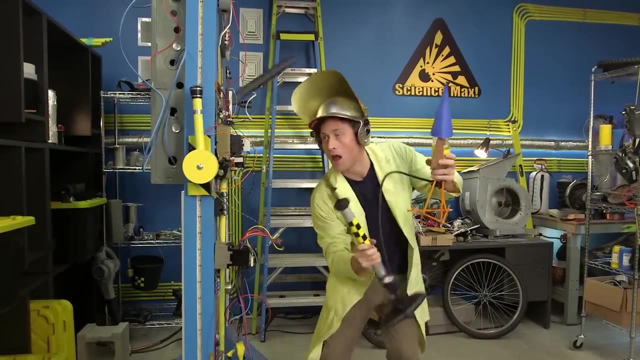 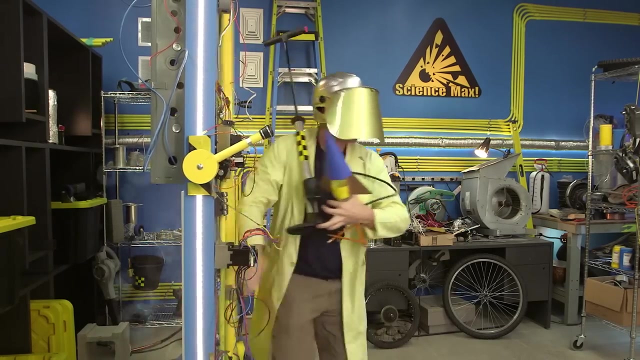 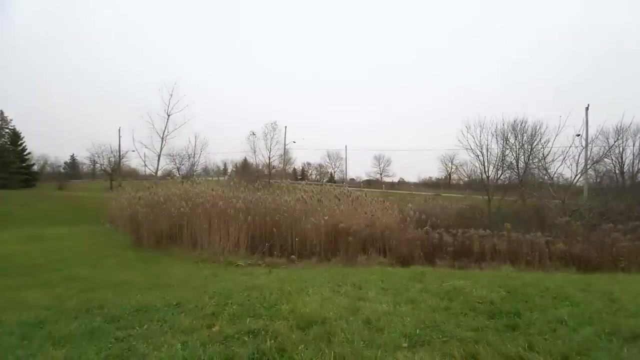 and then it's going to launch: Okay, here we go. You know, rocketry really isn't something you should do indoors. Come on, Hey, this was supposed to be a field. What's going? Why are there? Oh, it's in my shoe. 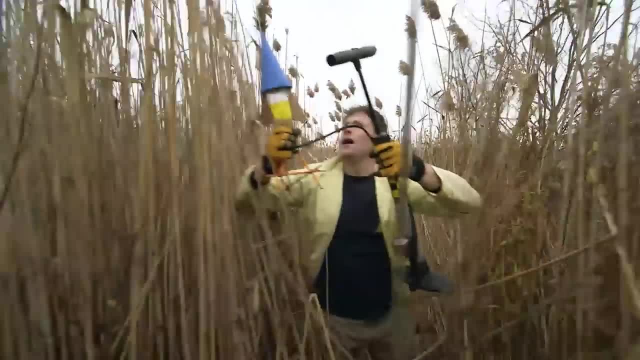 Huh, Oh, Oh, this will do nicely. Now don't forget to do this with an adult and don't forget your safety glasses. Now set up the rocket in a nice big, open area and make sure it's pointed away from you. 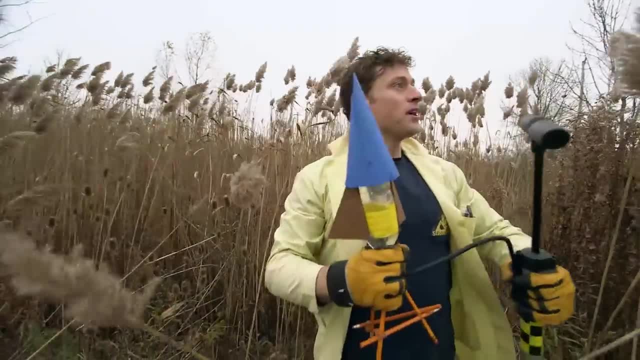 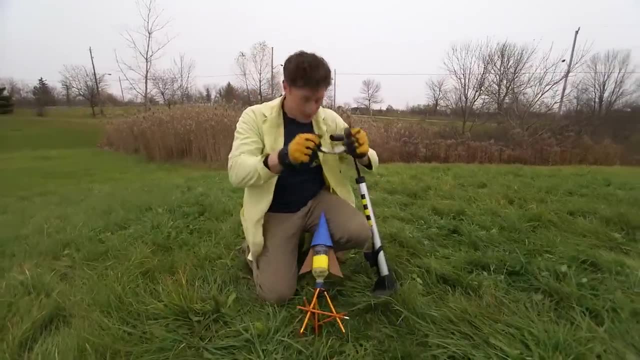 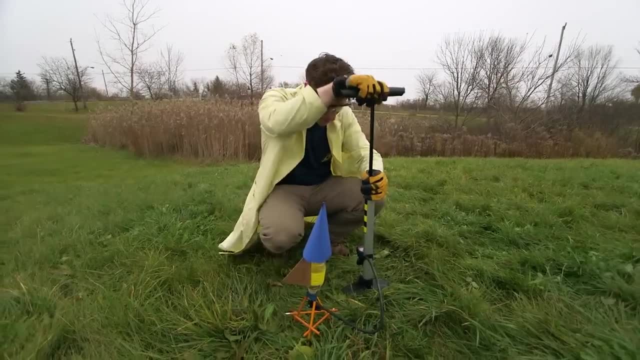 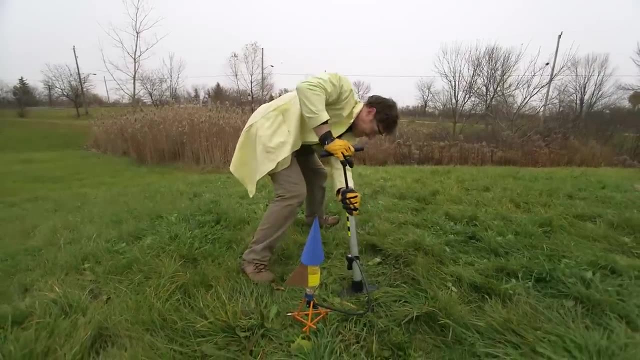 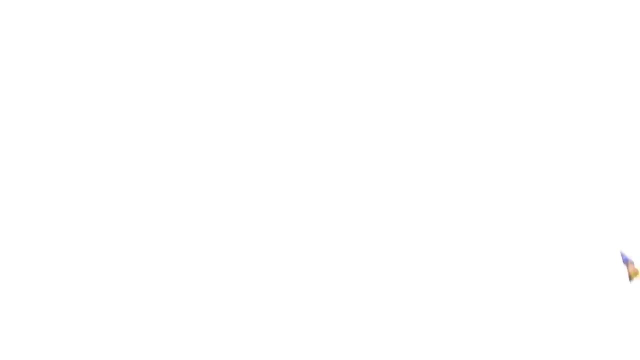 All right, All right. And then what you do is you pump the air pump and it puts air into the rocket which pushes down on the water, which will push down on the cork until eventually. Ha, ha, ha, ha ha. 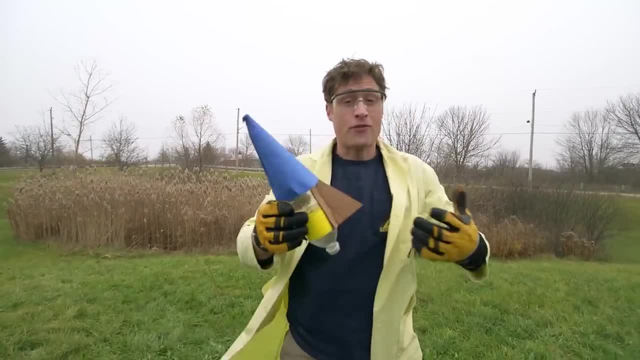 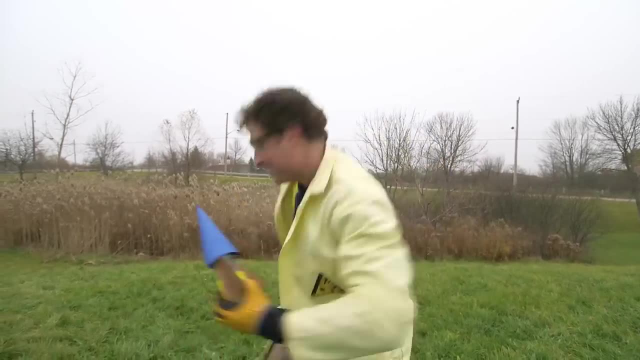 So be science Maximites and come up with your own rocket design. Try different amounts of water, different fins, even a different sized bottle. Try it for yourself and see if you can get one that goes. It goes higher than mine just did. 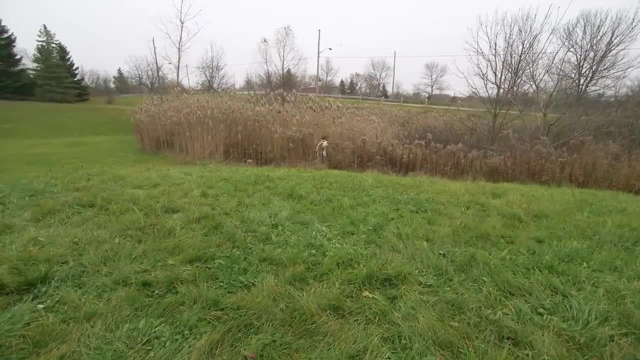 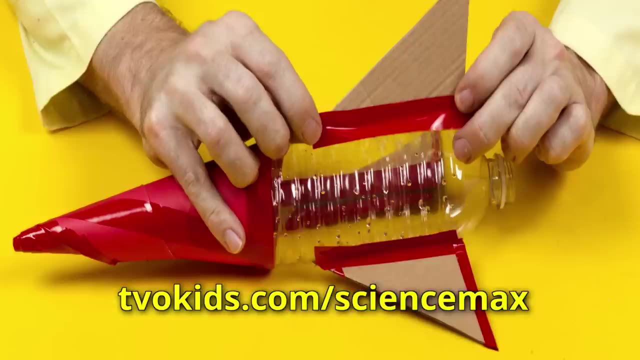 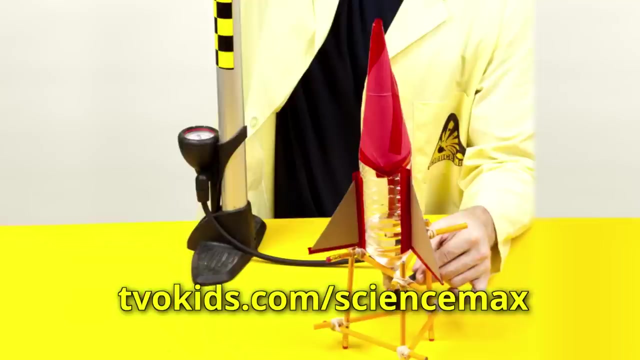 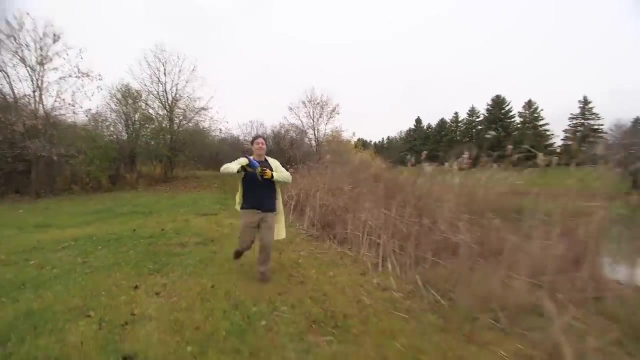 How did I get in? I think it was this way. Do you want step-by-step directions on how to build your own air-powered rocket? Well, don't worry. Everything you need is on our website All right. now it is time to max out. 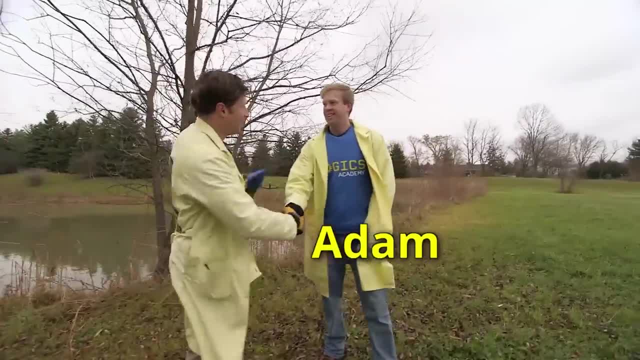 our air-powered rocket. I've got Adam here. Hey Adam, Hey Phil, How you doing Good, how are you Good? Adam's from Logics Academy, Logics Academy And you guys go into schools and talk about science. 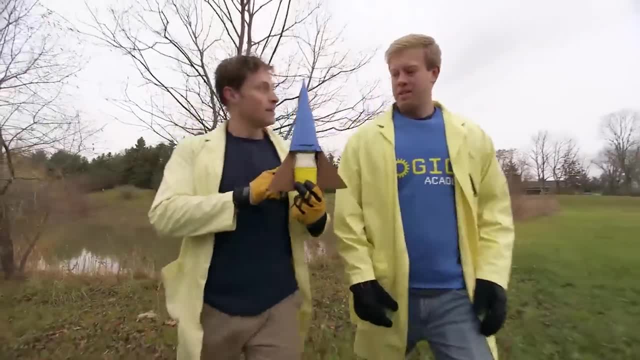 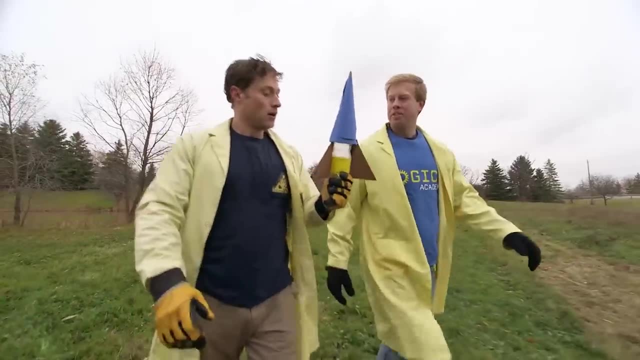 We do Fantastic. Do you guys do a air-powered rocket? Yes, exactly, Does it look like this one Looks exactly like that. Oh, that's great. So how do we max this out? So we want to add more pressure to this bottle. 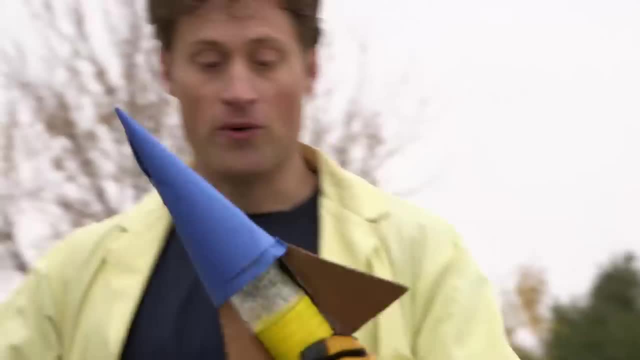 to try to get it to launch a little bit higher. More air, More air, Great. so what do we do? So we're going to use one of these- Ooh, it's an air compressor, Right, which works a lot like the bike pump, right. 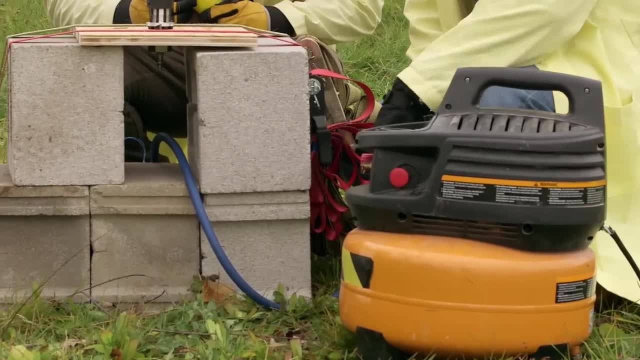 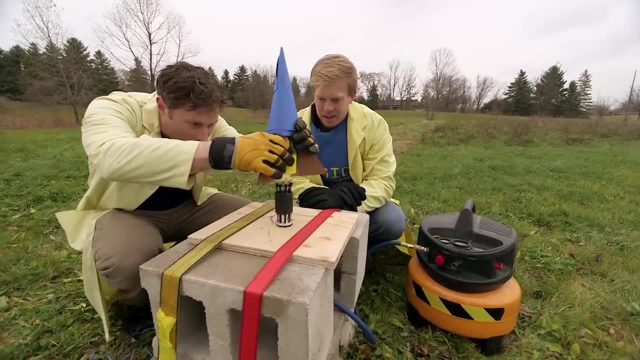 Yeah, exactly So. compressed air coming from here through this tube into underneath here and out that nozzle there And you're going to put your bottle on top And out the nozzle into the bottle like that. Yeah, and now we want to be able to hold it in place. 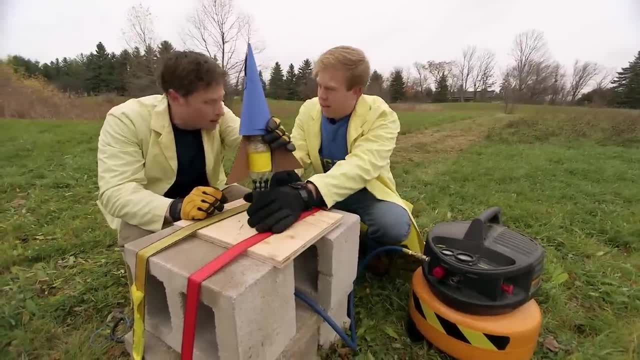 So we're going to have these little fingers here that are actually going to work to hold it until we want to let it go. So we're going to lock it in place. Oh yeah, look at that. Totally locked, Exactly. And then what? 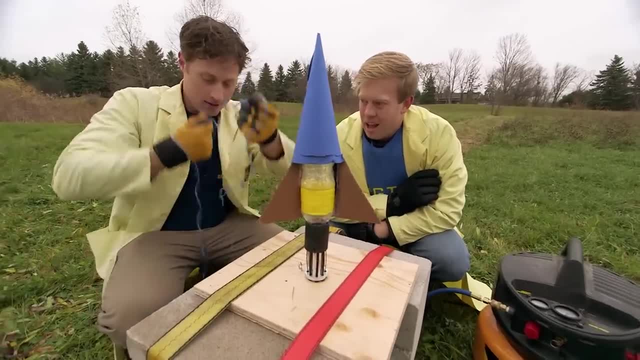 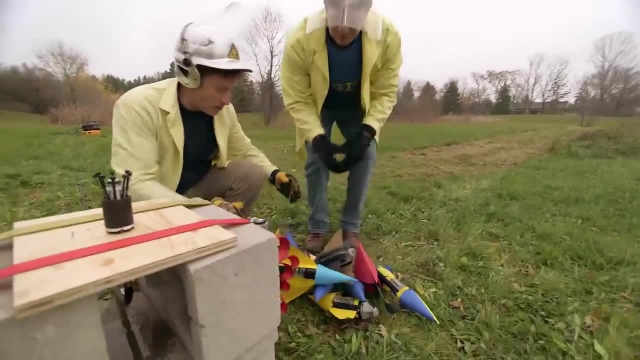 How do we launch it Now? you're going to take this cord and go a safe distance away And we are going to pull it, And then we would pull it. Which one do you want to start with? I think we should use this one here. 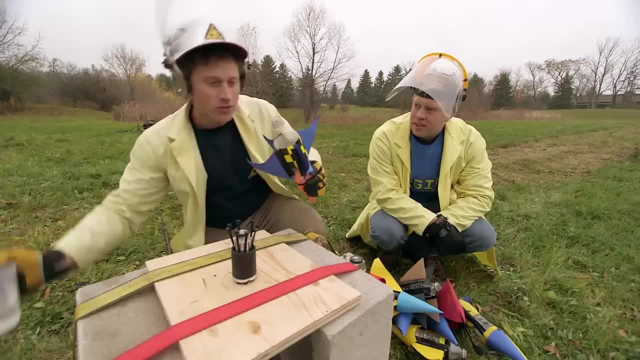 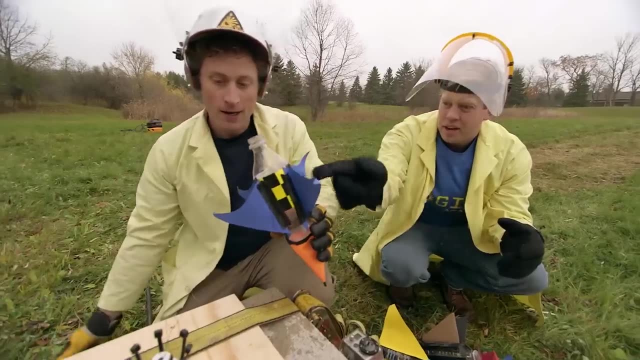 OK, great, Now we put water in it, right? Yep, you're going to put water in there. Why do we use water? So the water is going to act to push the rocket up into the air. The compressed air in here is going. 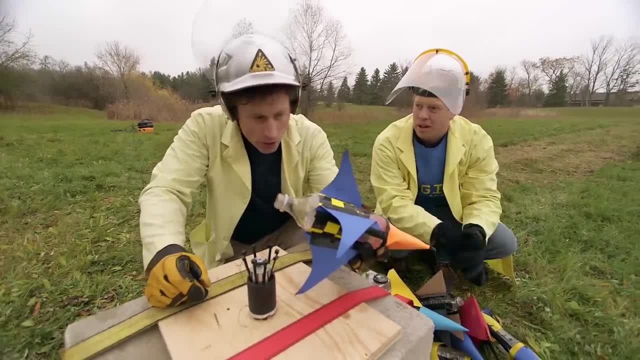 to shoot the water out the back, And the water is going to push on the rocket and make it launch. It's just to give it a little extra push. How do I get it on there without spilling any water? So just rest it next to the launcher there. 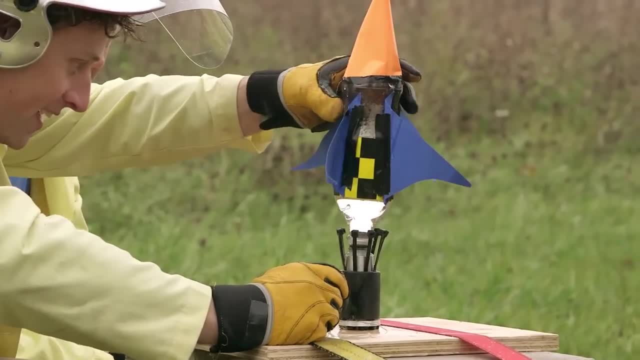 Just go fast. Yeah, just go really fast. Ooh, There you go, There we go. Just a little bit, Ha ha, And then Lock it in place. Locking it in place, There's no air pressure in the hose yet, right? 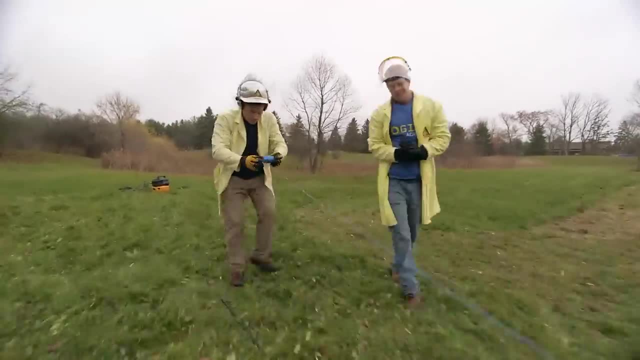 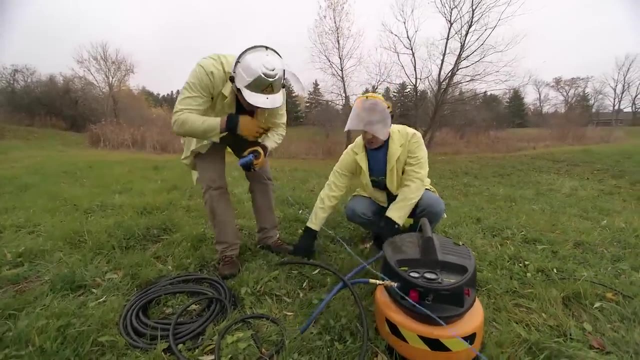 Not yet. no, First we have to spool out the launch cord, So the air compressor has the compressed air in it. It's ready to go? Yep, it's all ready to go. We just need to connect the hoses. 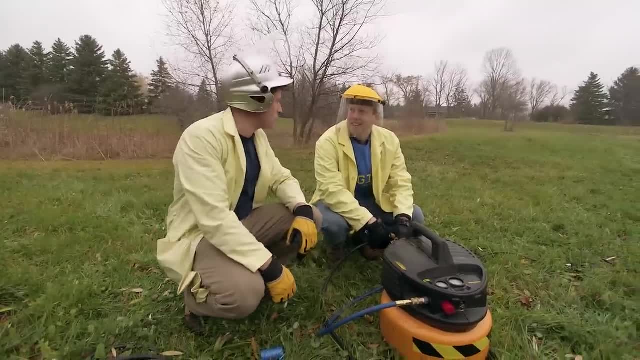 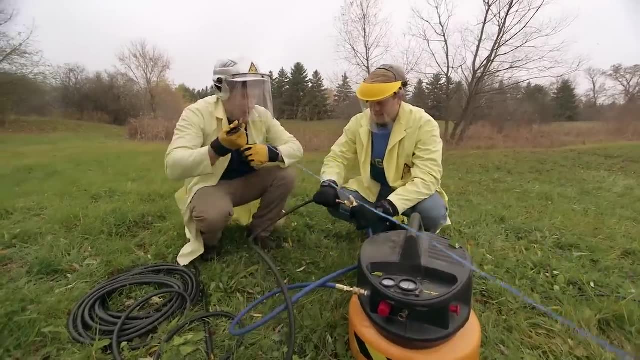 Adam, I've noticed it's snowing a little bit. Do you think that's any reason why we should stop? I don't think so. No, the science must go on. Blast shields down Connecting hoses. When we connect the air hose, the pressure 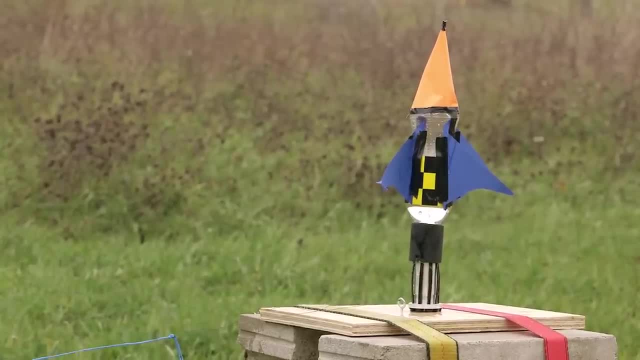 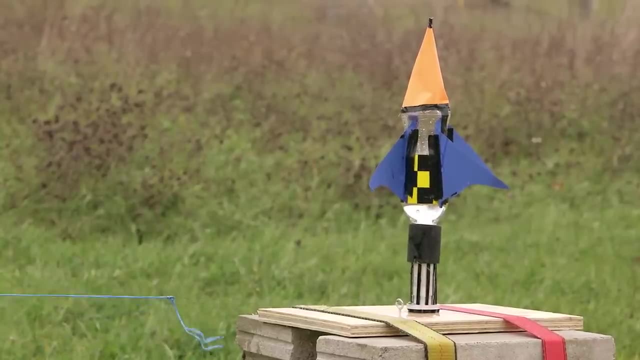 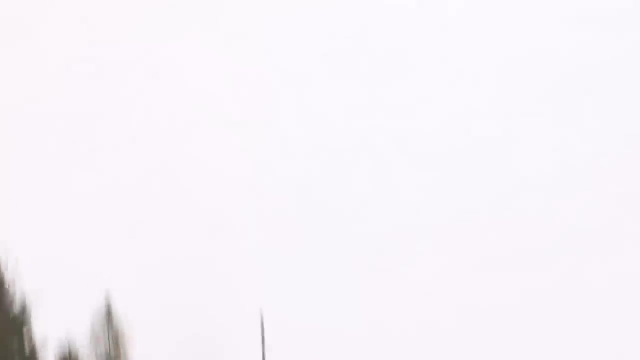 from the compressor travels down the line and into the bottle. You can see the bubbles of air going in. Those bubbles are carrying more air into the bottle, giving it more pressure. Here we go: 3,, 2,, 1.. All right. 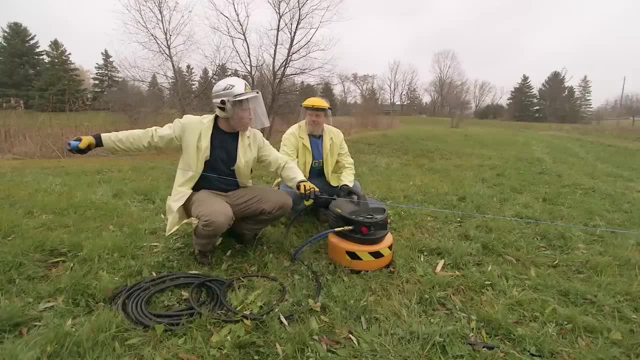 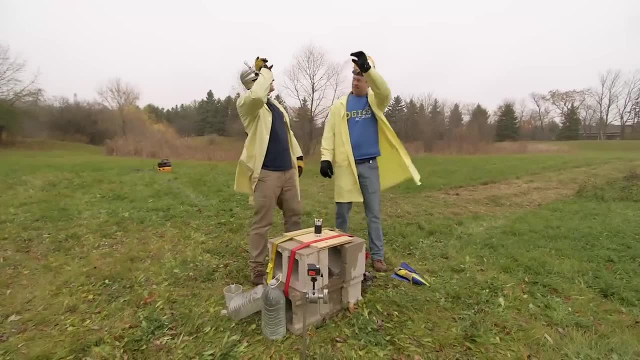 Another rocket. Let's do it again. Launch it, Get 3,, 2,, 1.. Woo, Ha, ha, ha, ha, ha ha. Nice, Success, Success, Nice. So small bottle worked really well. How do we make it bigger? 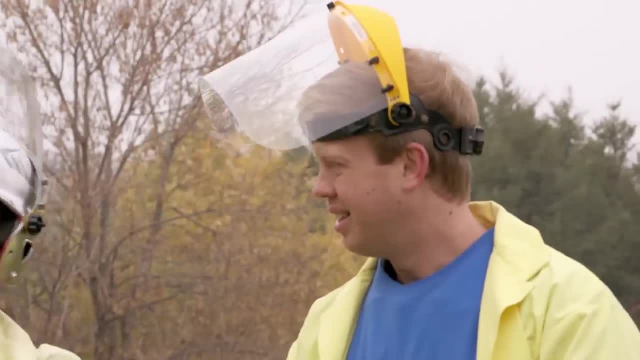 I know Bigger nose cone, I think a bigger bottle, Oh, a bigger bottle. Yeah, of course That's easy. How about this empty water bottle that we have now? That might work, except that the top here is too big. 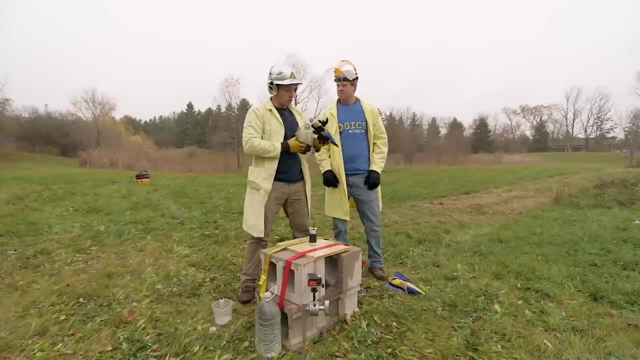 and I don't think it'll fit on our launcher. Oh yeah, So what should we use? A 2-litre pop bottle might work a bit better because it'll be about the same size. Oh, that's right. 2-litre pop bottles have the same opening. 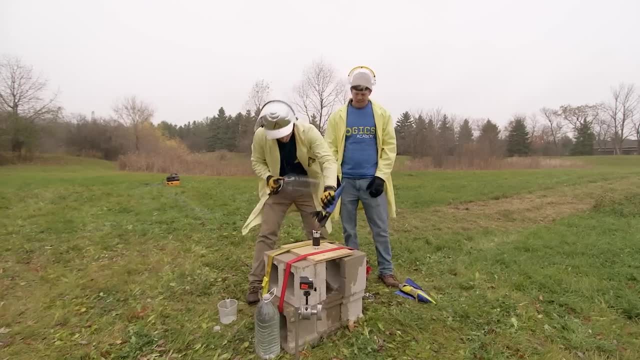 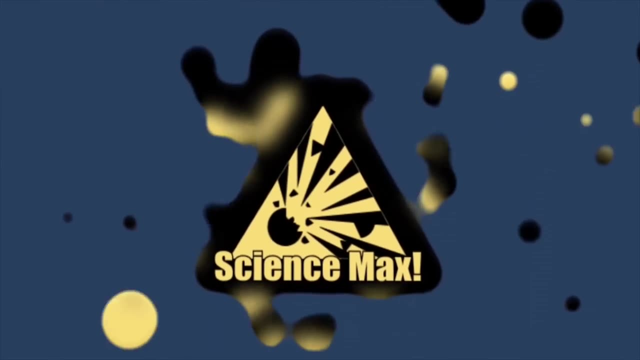 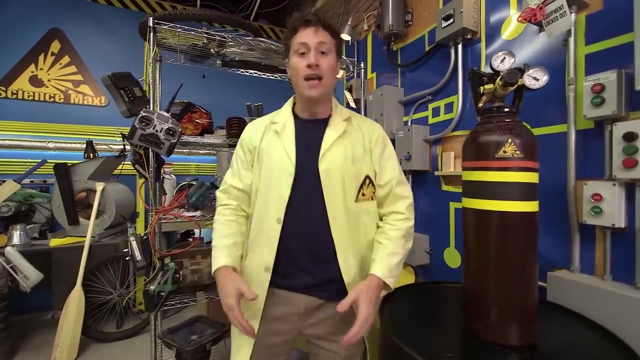 as these small water bottles, Exactly. That's great. All right, let's make a couple of rockets out of 2-litre pop bottles. Awesome Pressure happens when you squeeze something or compress it. Solids do not compress very well. 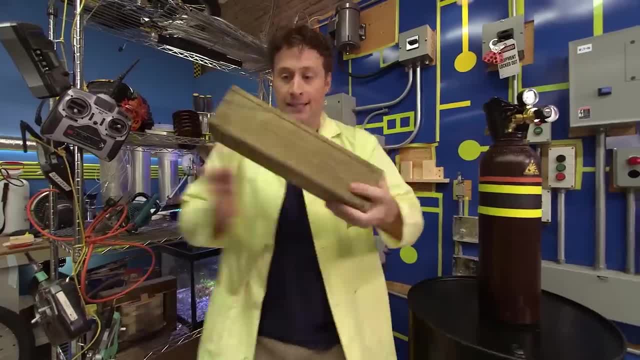 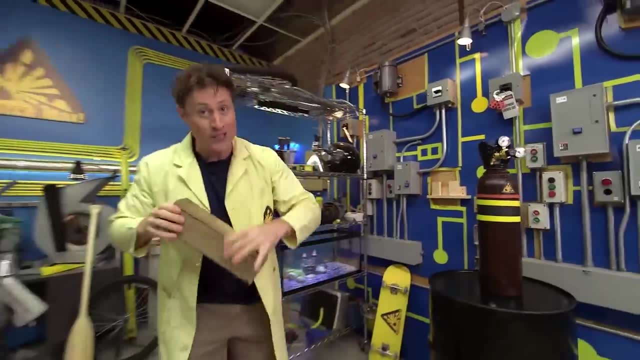 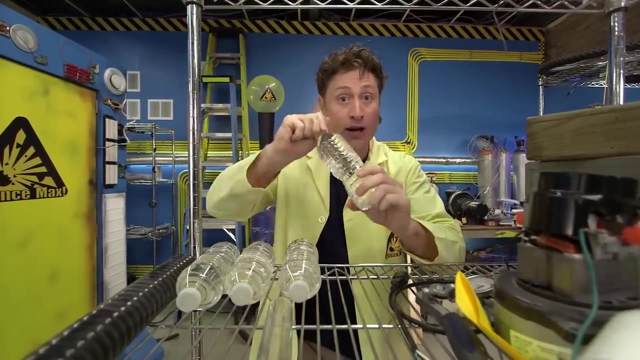 I will demonstrate. Um, solid, Is it compressing? No, okay, Liquids don't compress very well either. You can demonstrate this for yourself by getting a plastic water bottle and filling it right to the very bottom with water and putting on the cap. 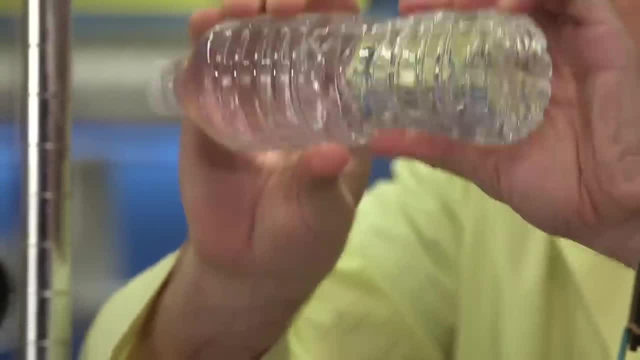 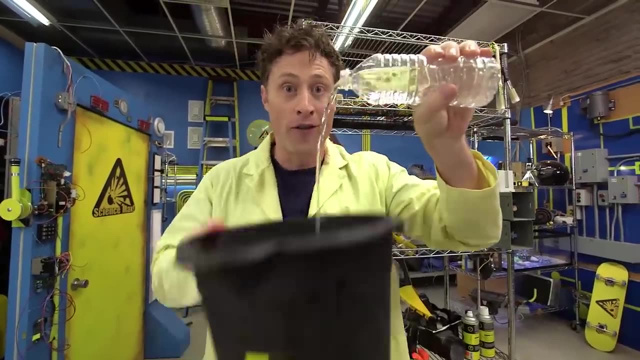 and squeezing, You'll find that you can't really squeeze the bottle very much. But if you empty out half of the water, no, don't pour it on the floor and then put the cap back on the bottle and try to squeeze it. 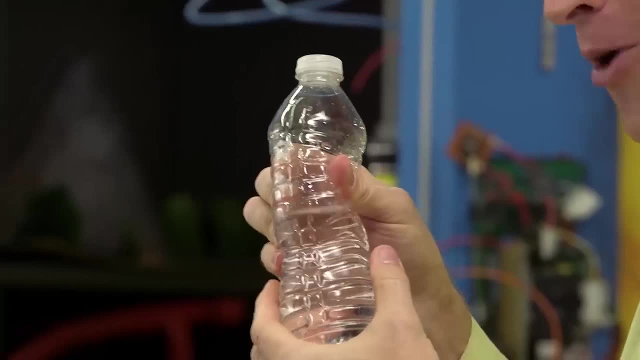 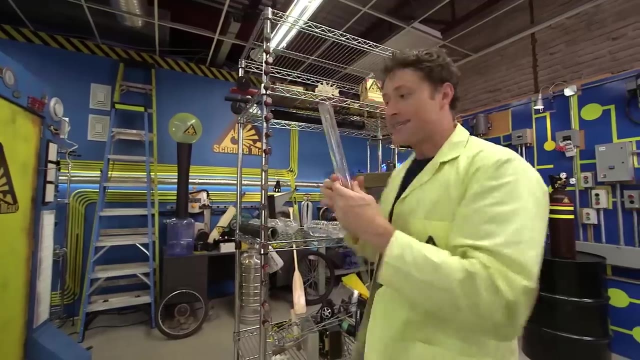 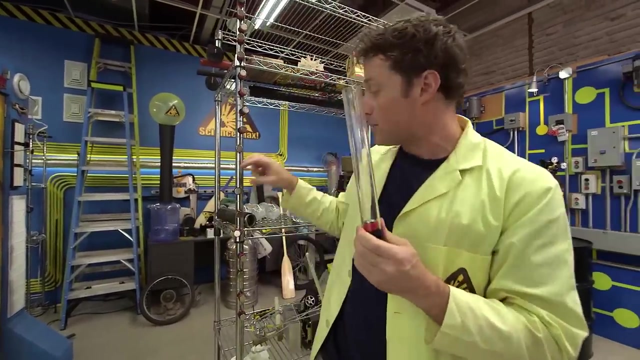 you'll find that you can squeeze it a lot more. That's because gases compress much easier than solids or liquids. Here's what's going on. Say, this container is well, any any container, And these magnets are air molecules. Now I'm gonna put the magnets in pole to pole. 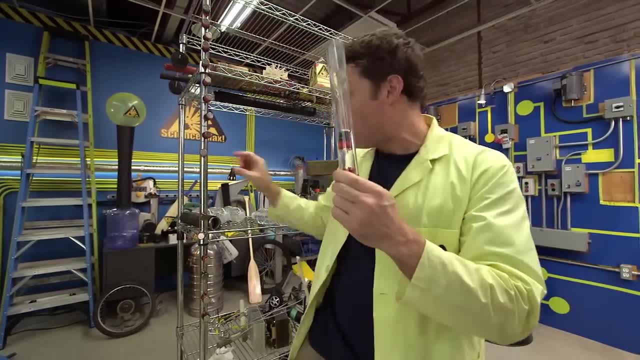 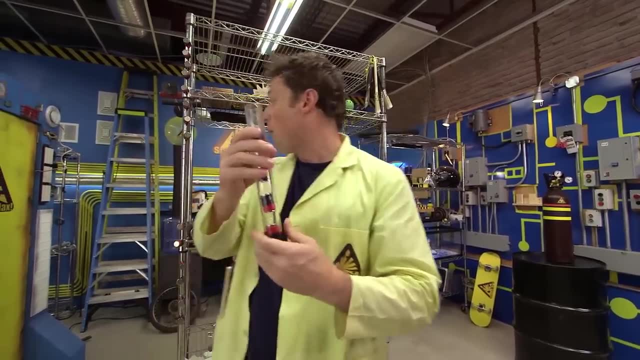 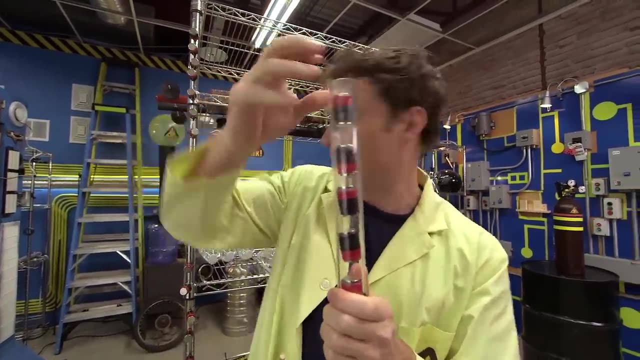 so they repel each other and want to stay a certain distance apart, just like air molecules do. There we go, A container at normal gas pressure. Now watch what happens when I add more gas molecules. They start to get squeezed together. And if I add more, 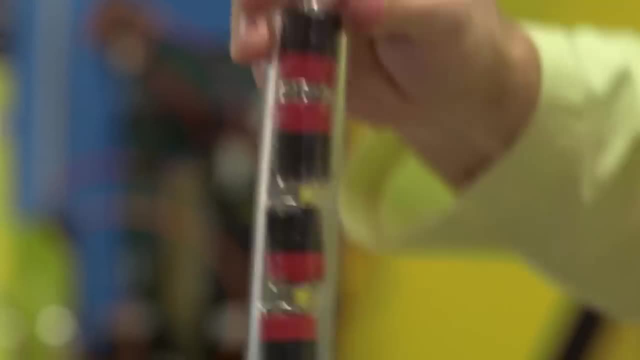 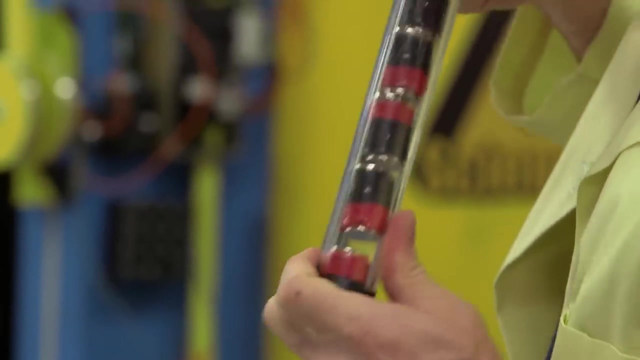 the amount of space that each one gets is less and less. Now this container is under a lot of pressure. These molecules really want to escape through the top of the container, but they can't because I'm holding them down. If I took something like this plunger. 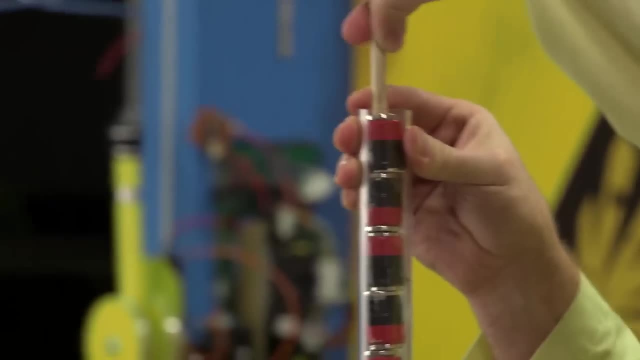 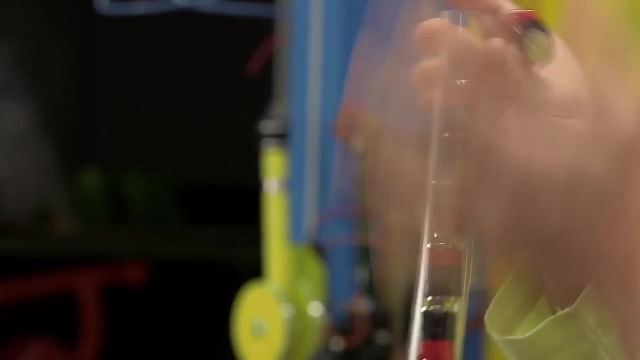 and I pushed them down even more. now they're really under pressure. They want to get out, but they can't because I'm holding them in. Now watch what happens when I let them go: They all pop out the top and the container has returned. 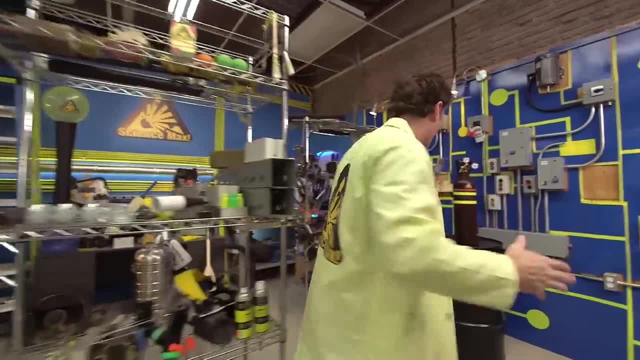 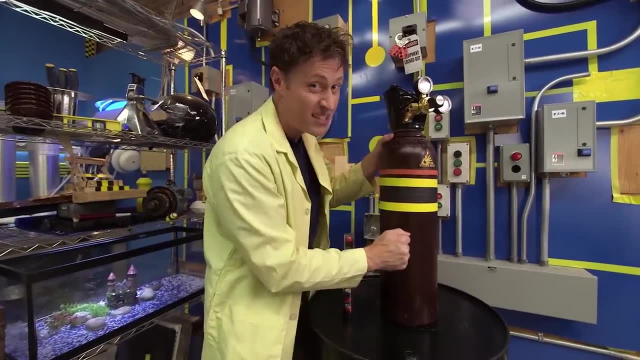 to normal gas pressure. That's what happens when we put gas in a container like this one. These containers that hold compressed gas are made out of solid steel because you need something really strong or it might explode if you put too much gas pressure in it. 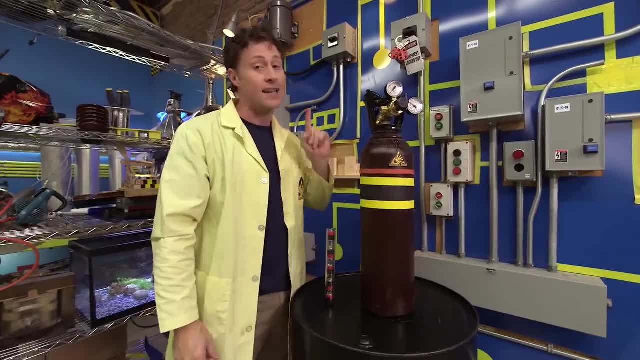 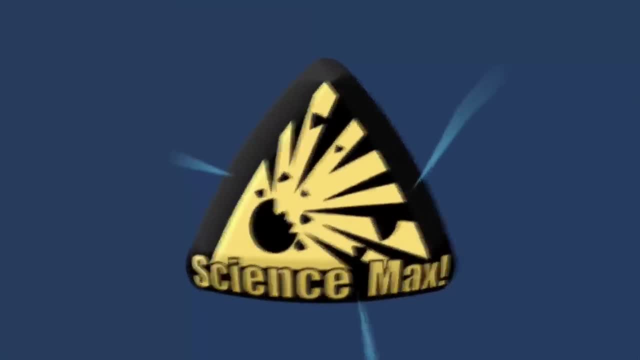 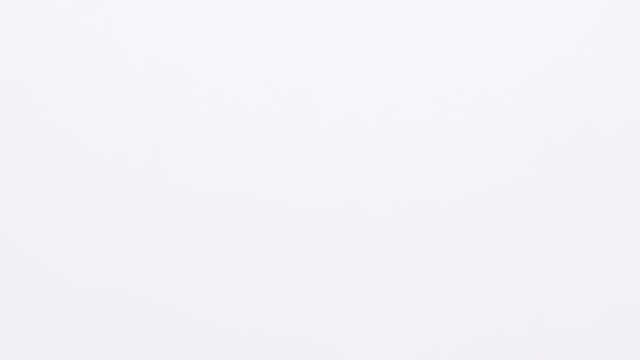 That's why these are only filled up by professionals who know exactly how much pressure it can take. That is the power of pressure. Our air-powered rocket was working pretty well. It was working, But there's always room to max it out In order to do that. 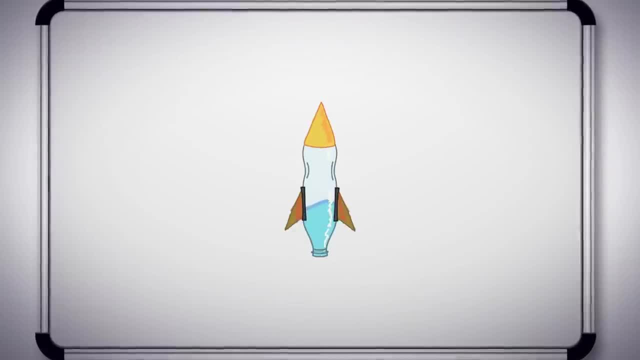 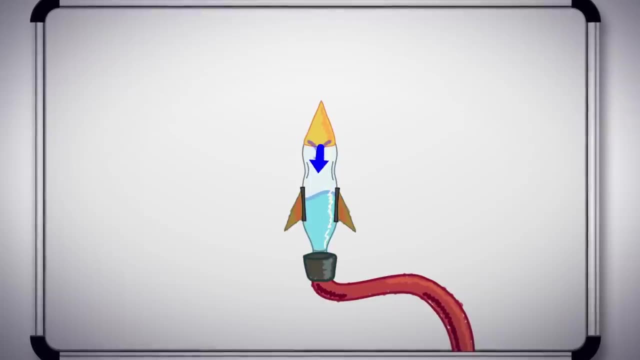 we need to understand how it works. First we fill the bottle almost halfway with water. then we add air to the bottle. The air pressure builds up and the air presses down on the water. The rocket takes off when we pull on the release valve. 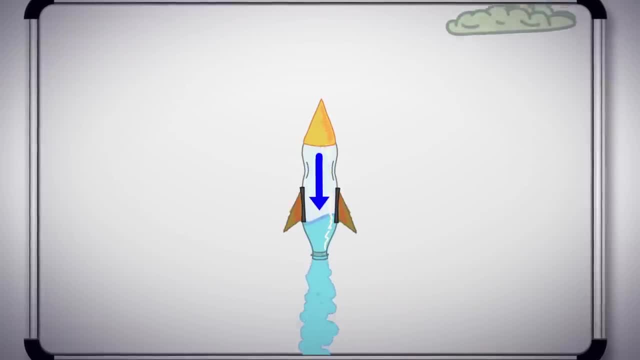 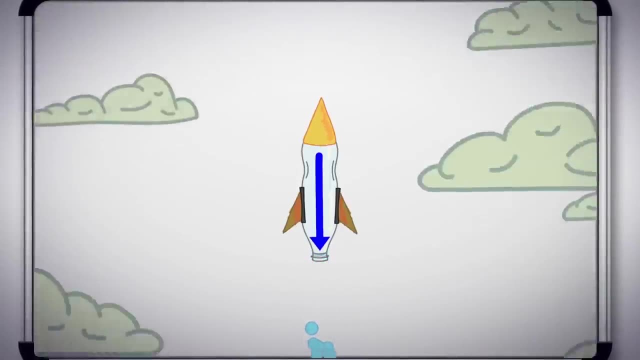 which was blocking the opening of the bottle. Once that happens, the air pushes out the water. It's the water that gives us our thrust, so the water is very important. Once all the water is gone, the air escapes and the bottle returns to normal air pressure. 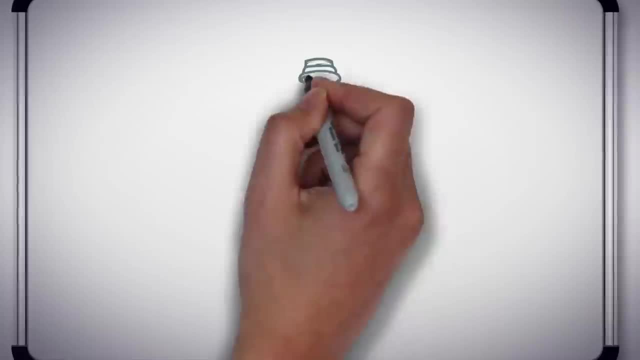 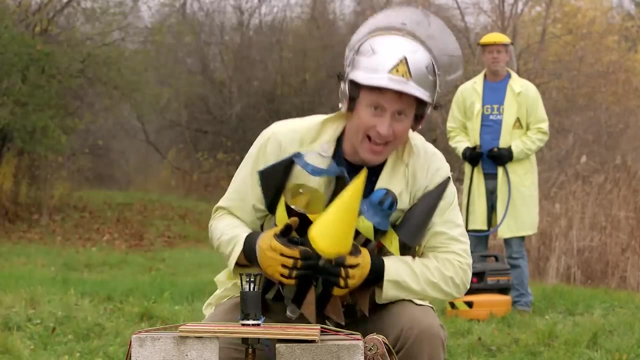 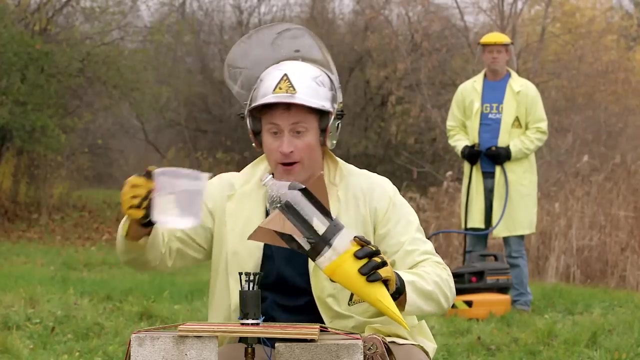 But by that time it's high in the sky. Now the plan is to use two-litre bottles instead of regular water bottles to see if they work better. Now we've made a few more rockets out of two-litre bottles and I'm going to fill this one up with water. 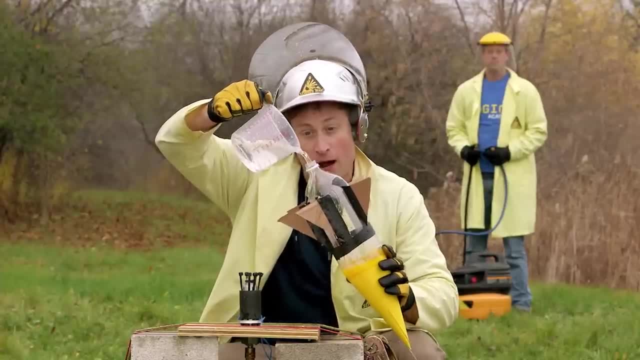 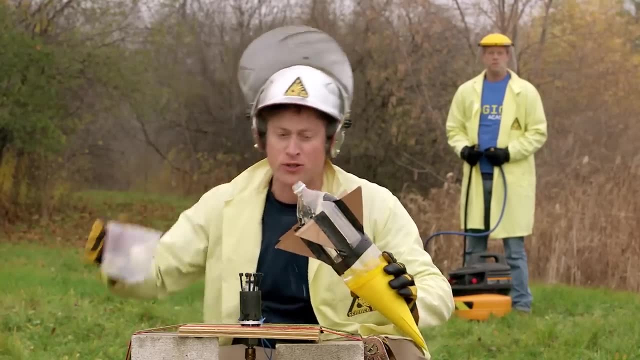 and we're going to fire it again and see what happens. Now. the idea is that these will work better because they have more volume, and more volume means we could possibly put more air pressure in. It's hard to know until you try it, of course. 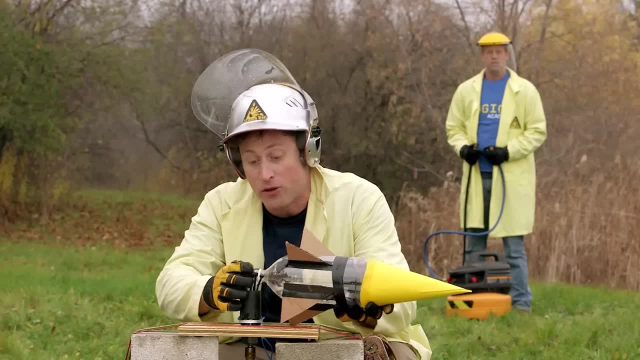 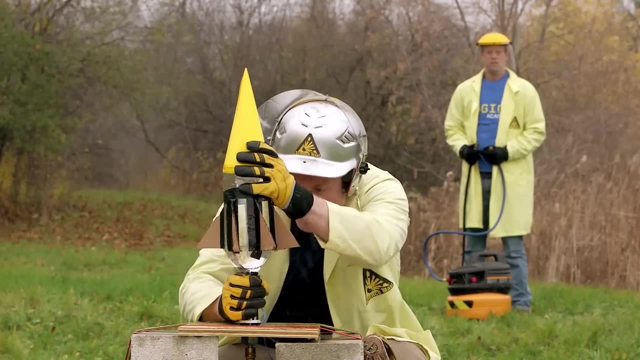 But the other reason why it might work better is two-litre bottles generally hold carbonated beverages, which means they already have to be made a little stronger than regular water bottles because they have to hold in the carbonation, which is just like air pressure. 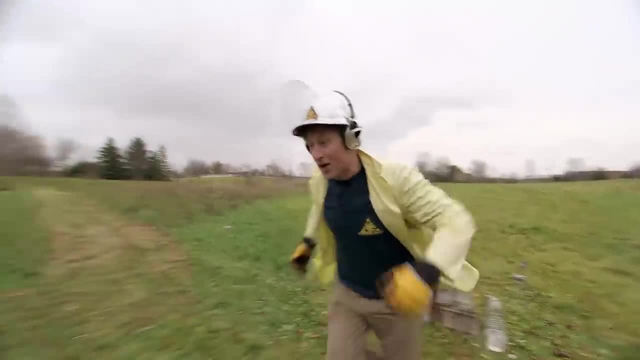 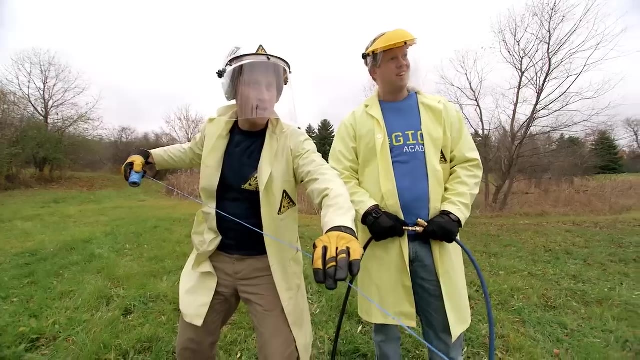 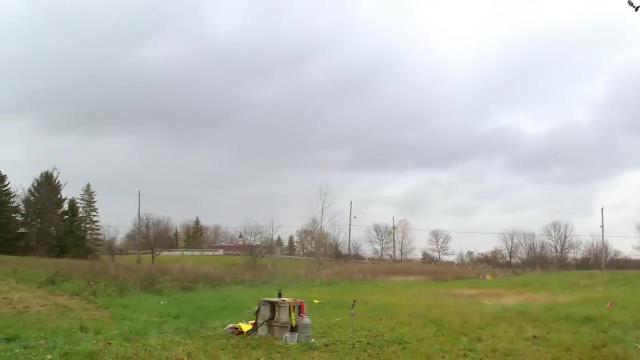 All right, ready to go? Okay, here we go. You ready, Adam? Yep, Okay, All right, let's get the blast shield down. Pressurize Three, two, one. Let's do another one. And three, two, one. 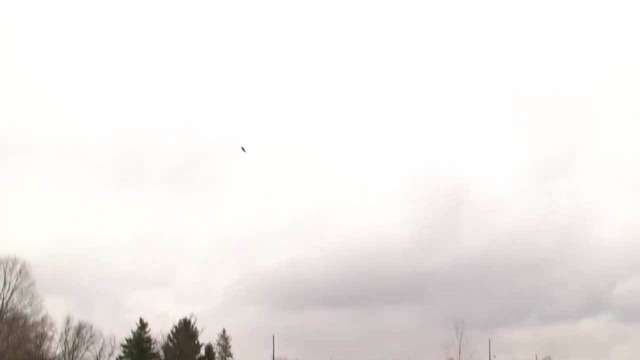 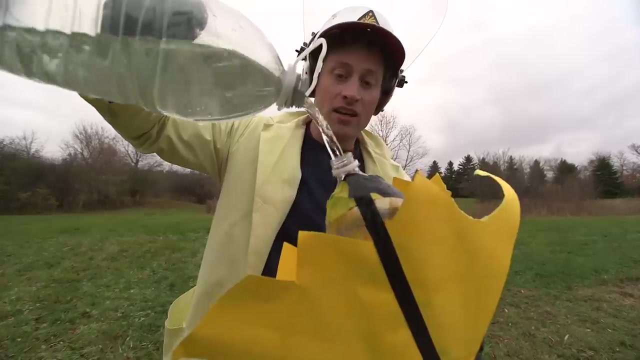 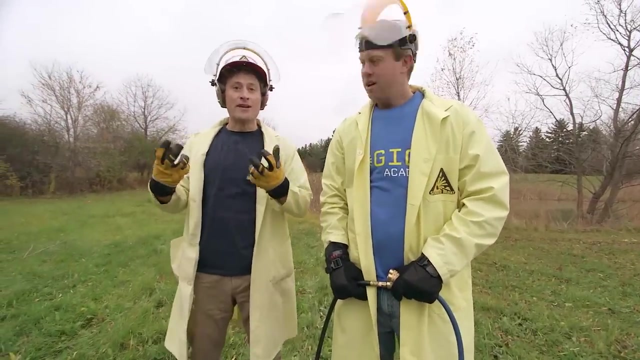 Whoa, Wow. This is the superhero design rocket, which I'm very excited about. All right, Adam, You're doing really well, But before we fire this next one, how can we make it bigger, better and more awesome? Getting more pressure, More pressure. How do we do that? Well, we're firing at about 90 psi right now. Psi pounds per square inch of pressure. right Yeah, So we could increase it. We could increase it. So how? we're at 90 now. 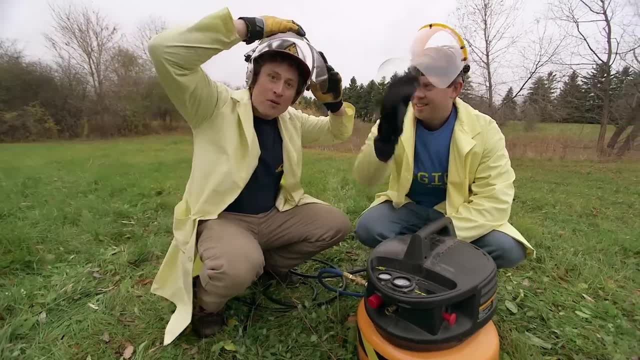 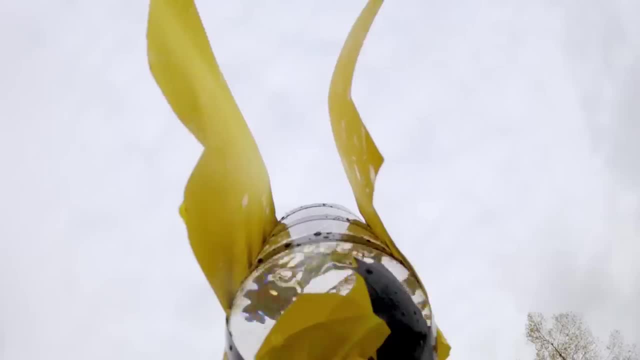 How high does the tank go? Go to about 120.. 120 psi. Let's see what happens. All right, let's do it. Okay, here we go: 90.. 110.. 120.. Should we fire it? 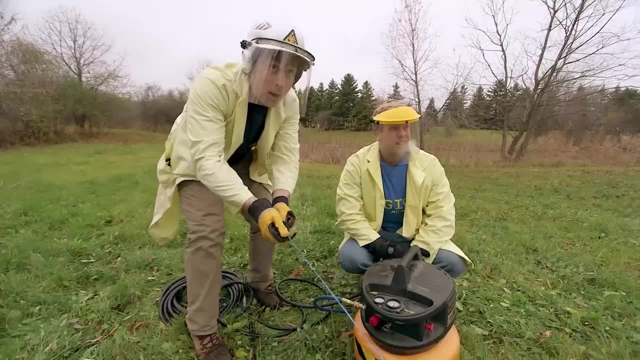 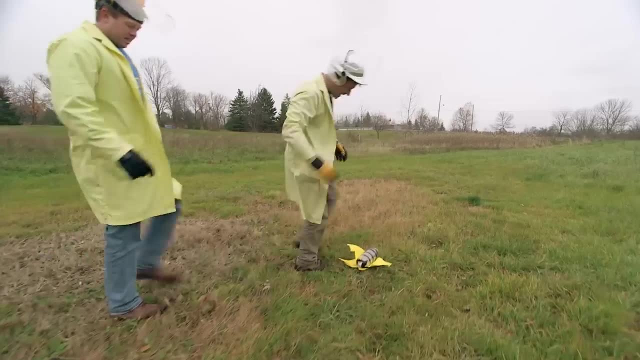 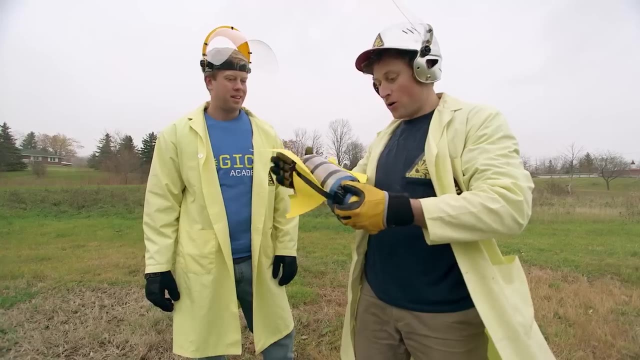 Let's fire it. Let's fire it. Here we go. Three, two, one, All right. Hey, actually it worked. okay, There's just a piece missing here, but I think the bottle is still okay. Yeah, So two-liter bottle full pressure. 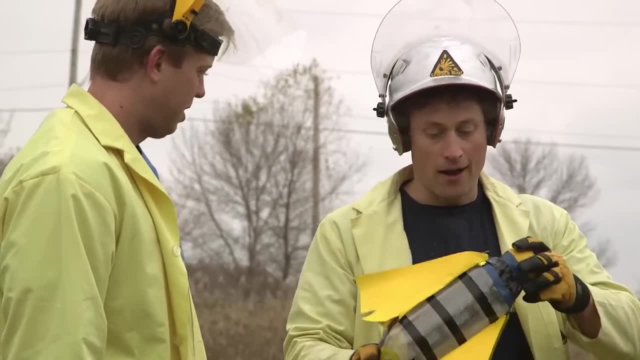 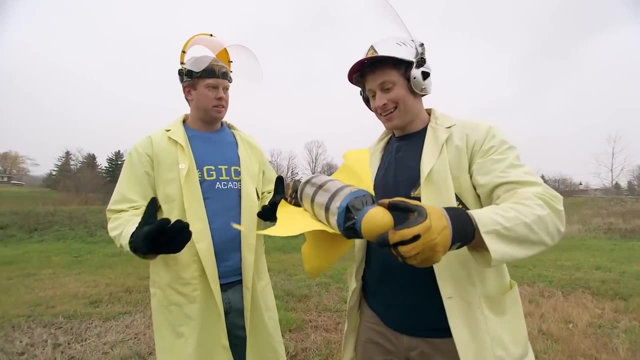 I think we can still make something even better, even more maxed out. What if we used an even bigger bottle? You know the five-liter ones that you see on a water cooler? Yeah, You think we can use one of those. Definitely, I think we could use that. 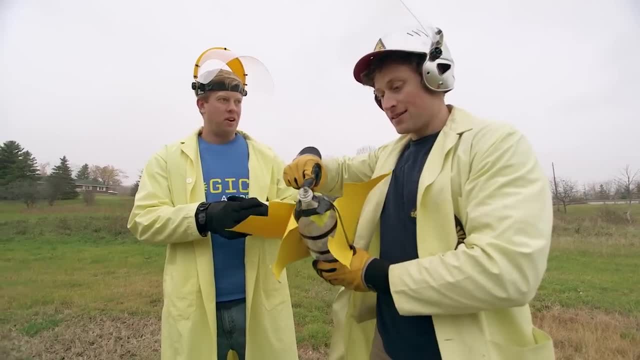 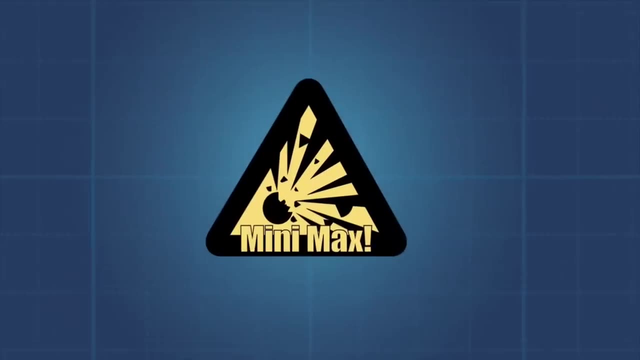 We need to change the mouthpiece size- Oh right, Yes- To fit our launchers. Well, let's do it. Let's do it. Mini Max, Help. I'm being crushed by all this pressure. A whole kilogram is being pushed down. 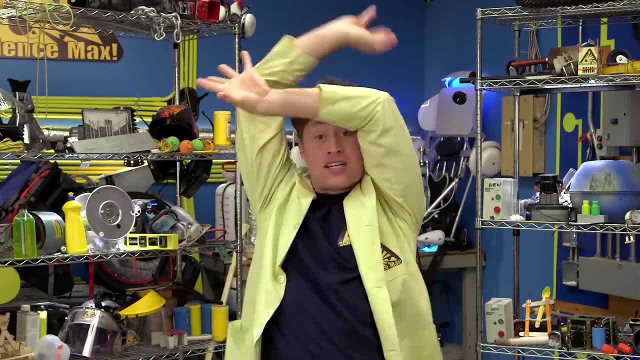 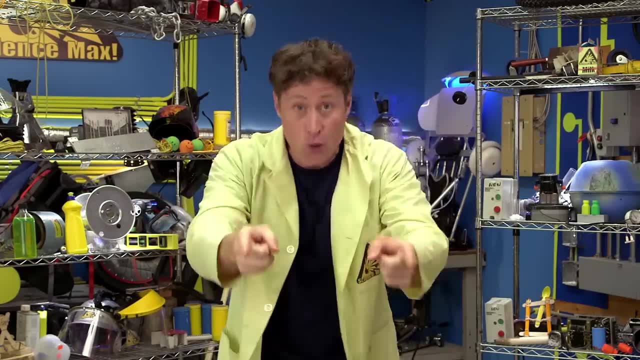 on every square centimeter of my body: 103 kilopascals. 103 kilopascals- Actually one kilogram for every square centimeter on your body- is the exact kind of pressure that you and I are under at all times every day. 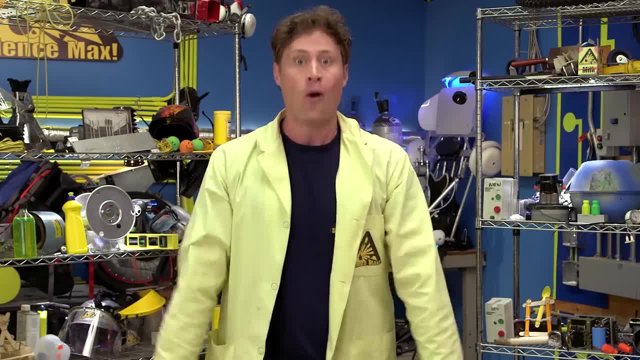 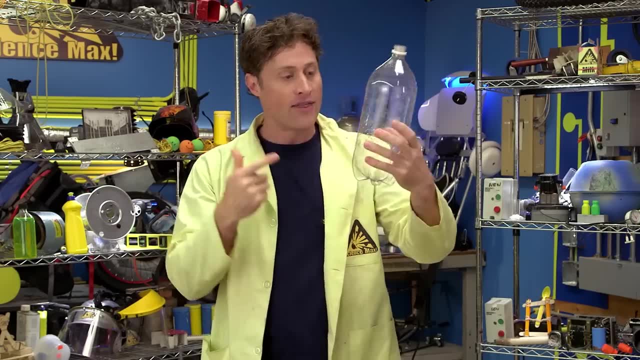 We don't notice it because we're used to it, but it sounds like a lot, doesn't it? Well, it is. Here's an experiment you can do with a plastic bottle. Say, at room temperature, there are 10 million air molecules in here. 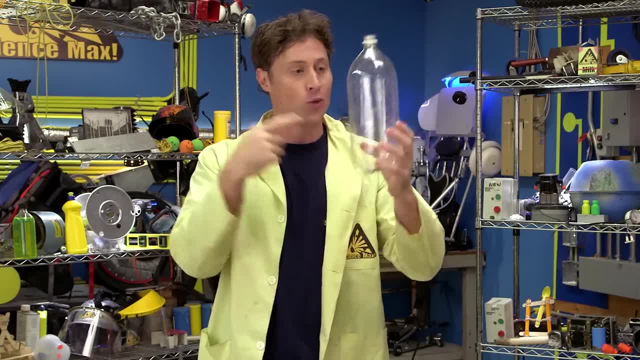 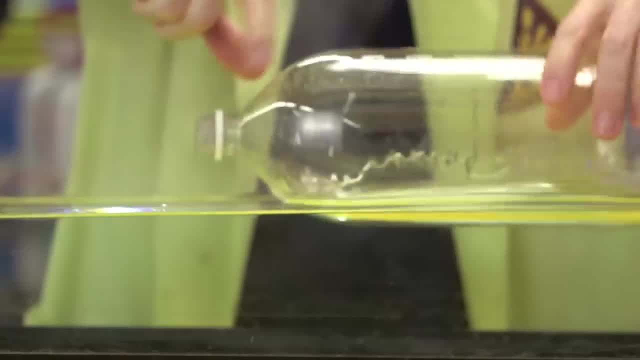 Doesn't really matter how many, but we'll say there's 10 million at normal room temperature. What happens if I heat up the air inside this bottle? This is warm water. What I'm trying to do is heat up the air inside the bottle. 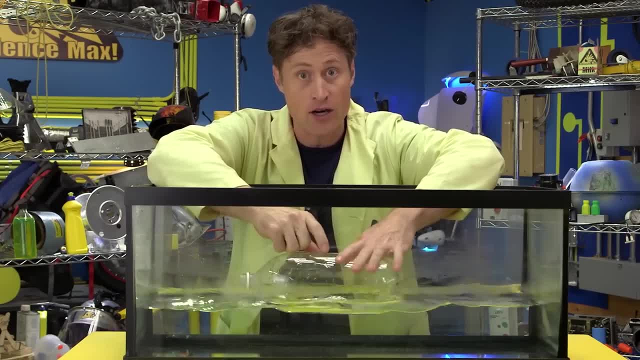 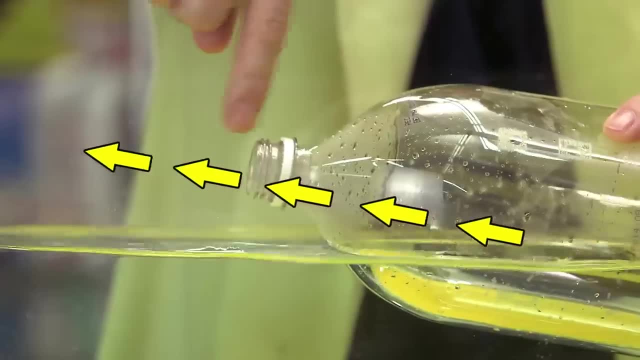 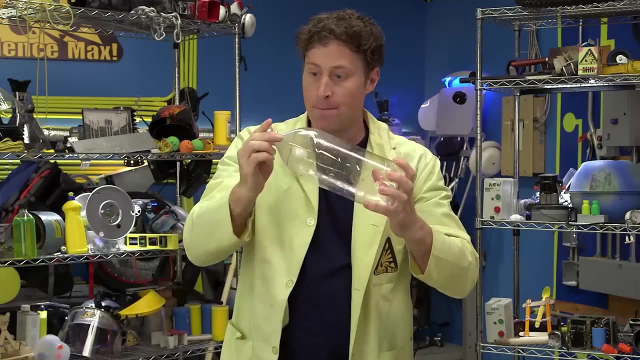 because the air molecules, when they get hotter, move faster and need more room. So the 10 million air molecules are starting to escape out the mouth of the bottle and reducing the number of air molecules inside. And now I take the bottle out and cap it. 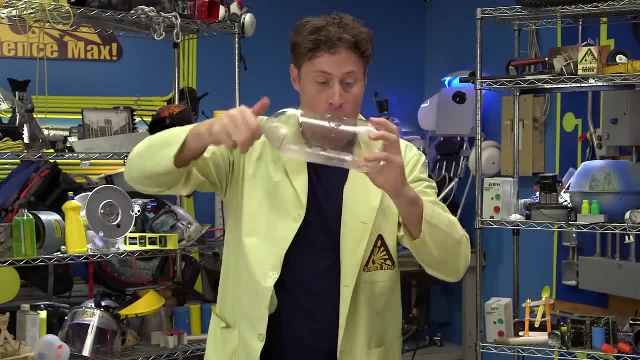 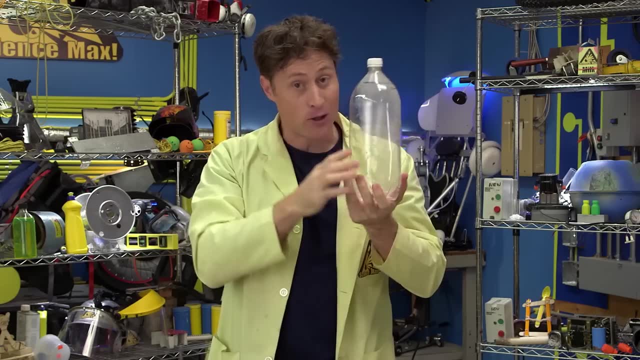 Because the air molecules heated up and speeded up. they needed more room. Now there's less of them in the bottle. There's about 4 million air molecules inside this bottle, but they're all hot air molecules and they have a higher pressure. 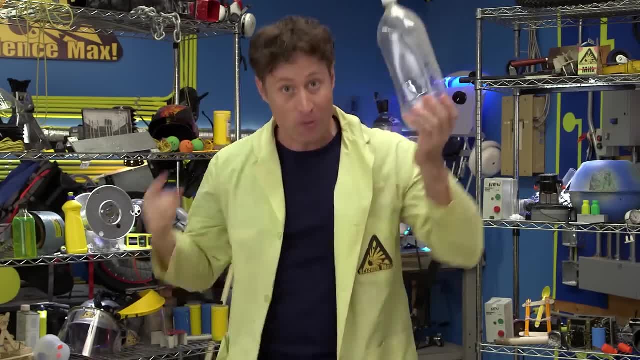 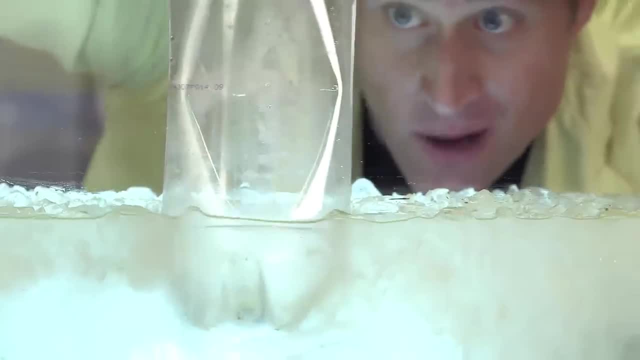 and you don't notice it, because the air out here isn't crushing the bottle. But watch what happens if I cool the air inside the bottle. This is ice water. So what's happening now is the molecules are slowing down and they need less space. 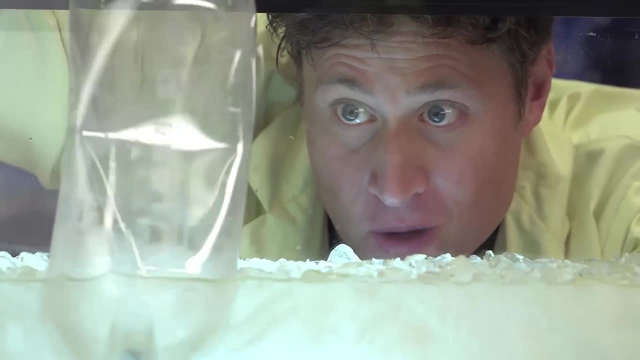 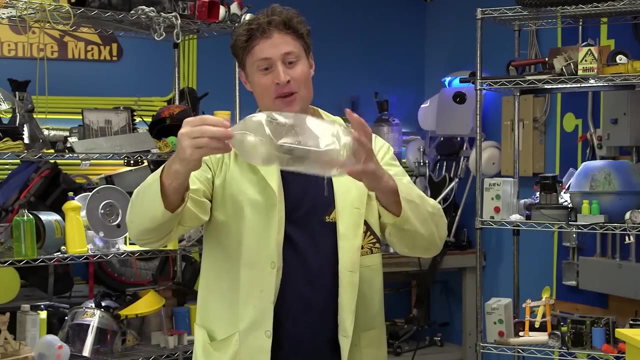 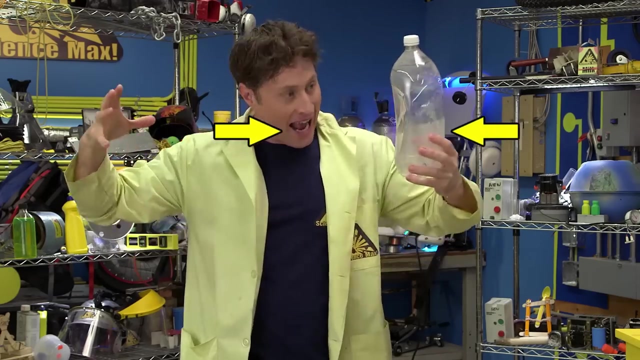 So they need less room and they're being crushed by the pressure on the outside of the bottle. It has been crushed because the colder air molecules don't need the same kind of room as the hot air molecules. The room temperature air has crushed the bottle. 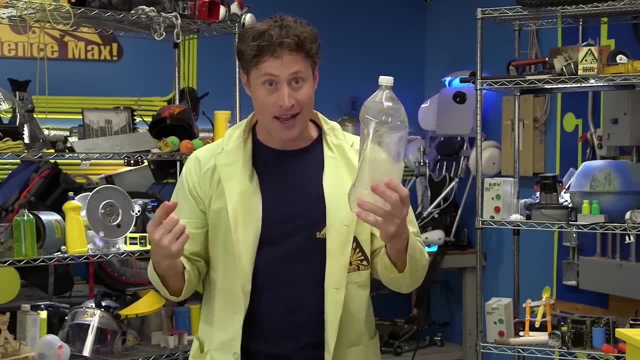 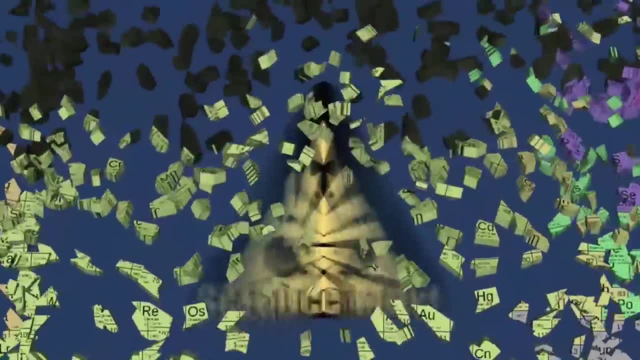 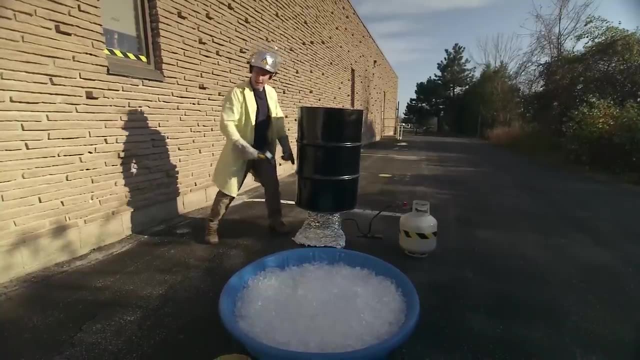 The air inside has a lower pressure than the air outside. Pretty amazing. Even more amazing when we max it out. This is a steel drum. What we've done is we've put some water in it and we're heating it up to boiling, so there's nothing but hot air inside the drum. 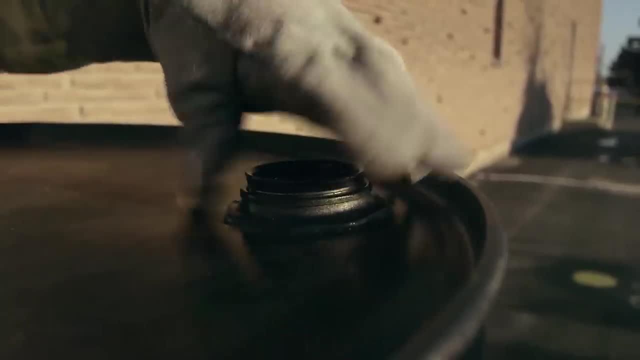 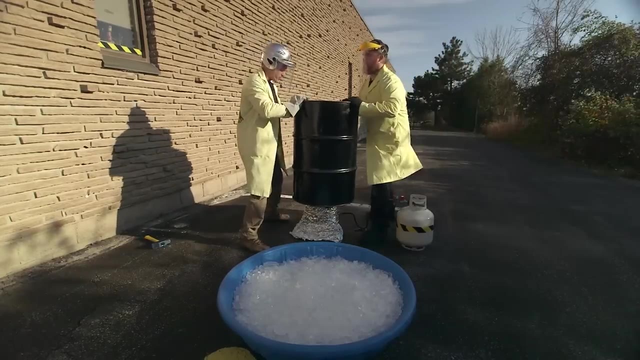 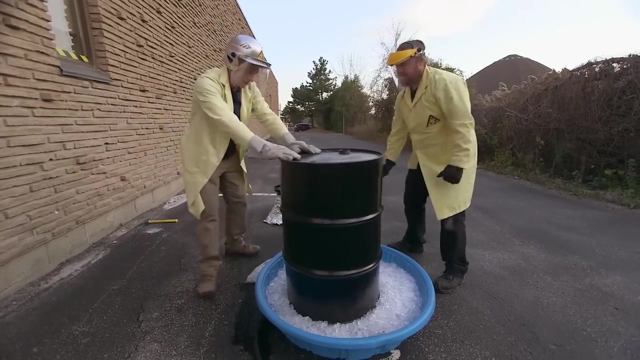 This is an airtight cap which we use to seal the drum And now we cool the drum off. Hey, Trevor, give me a hand Ready. One, two, three you lift. That's good, This pool is filled with ice. 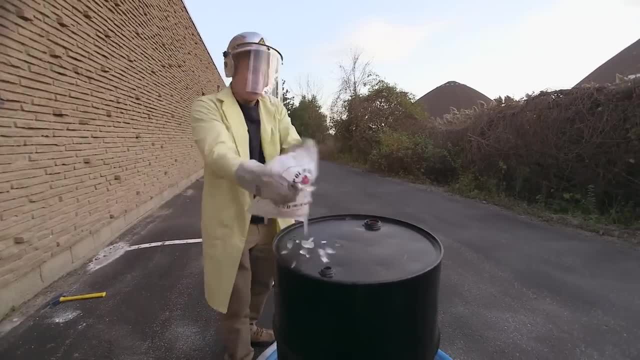 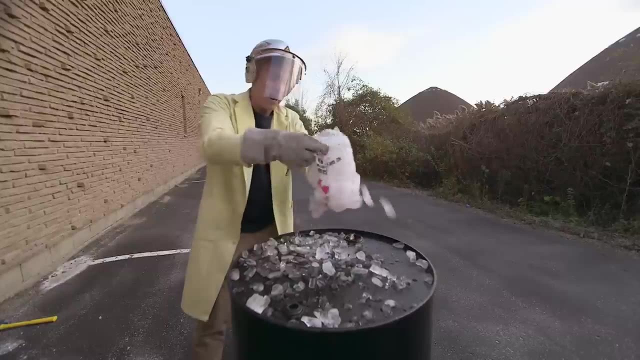 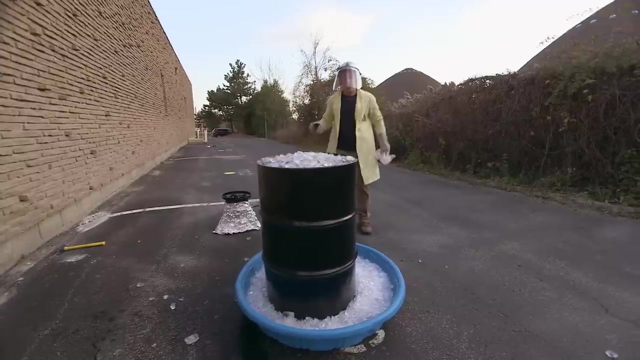 What we're doing now is cooling off the steel drum, which will cool off the air inside it, Which means eventually, the air inside the steel drum will be a much lower pressure than the air outside the steel drum, Because this steel drum has a lot more volume. 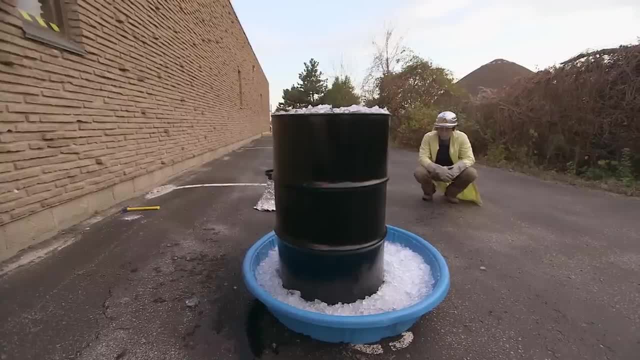 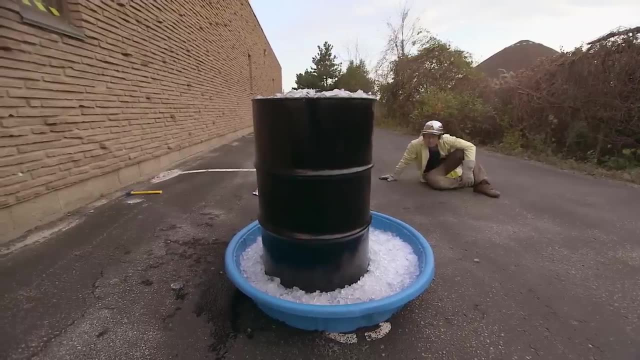 than a two-litre pop bottle. it takes a lot longer for the air to cool down. The other thing to think about is that it's a steel drum. I could stand on it and it wouldn't even dent, But sure enough, after a few minutes. 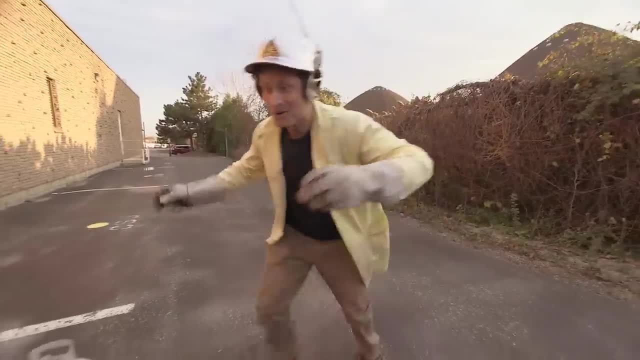 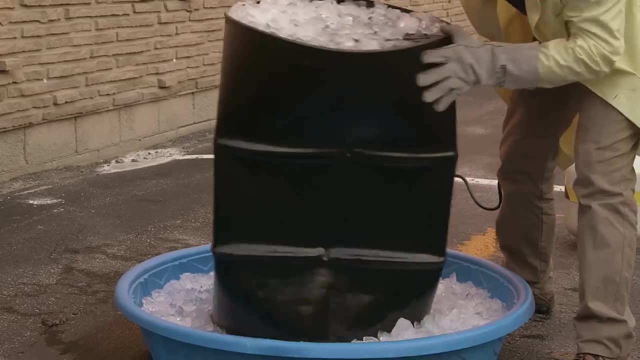 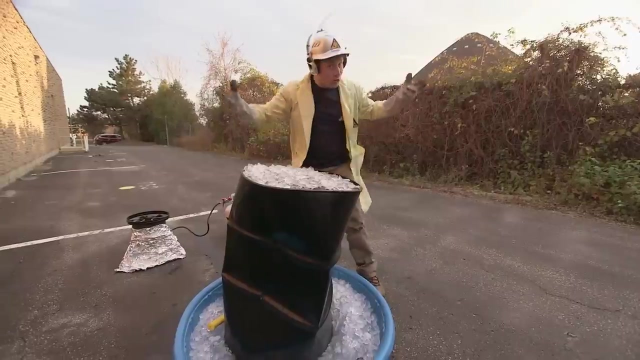 Whoa-ho-ho-ho, Check it out. The barrel has totally crushed. The low-pressure air inside the barrel wasn't enough to withstand the force of the regular air pressure that you and I walk through every day, The air pressure all around us. 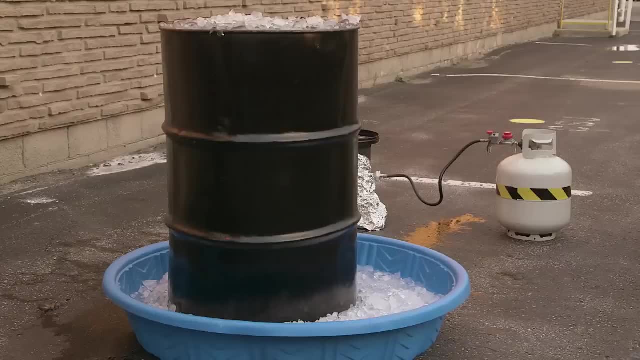 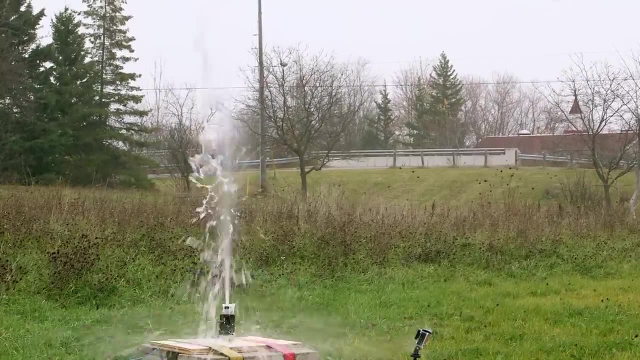 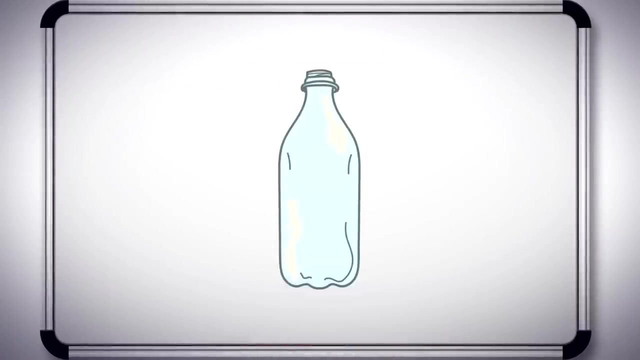 is enough to crush a steel drum. How cool is that Our air-powered rockets have been working really well, But we still want to go further. Since the two-litre bottle worked better than the water bottle, we think increasing the size again might make it more awesome. 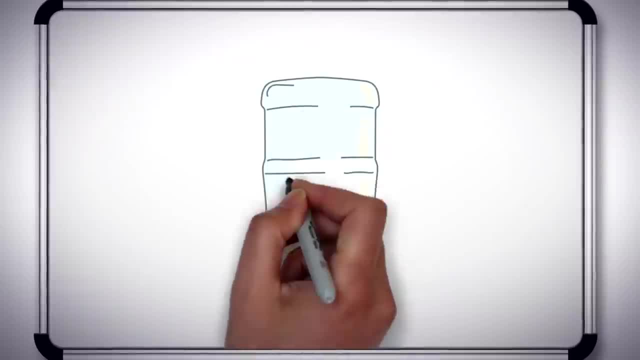 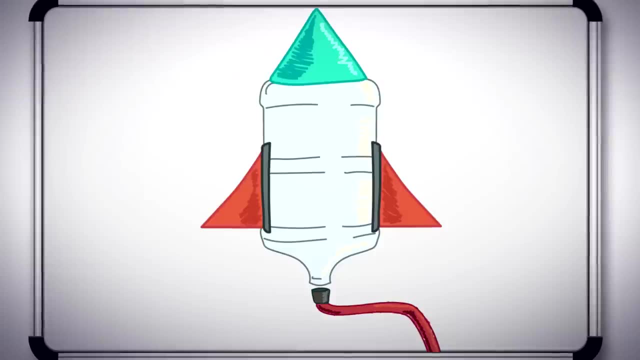 So now the plan is to switch our two-litre bottle with a 20-litre water cooler jug and make a rocket out of that, Because the launcher nozzle, which holds the bottle in place till we're ready to launch it, isn't going to fit the opening of this bigger jug. 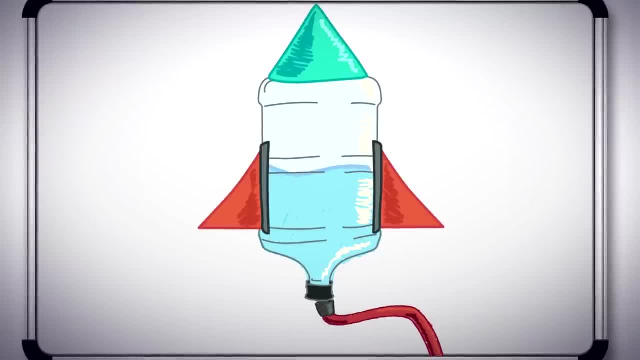 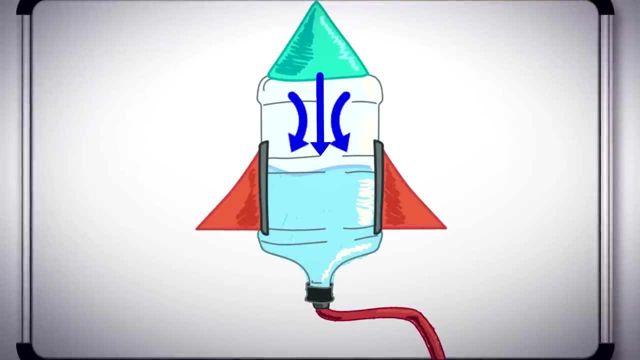 we've decided to use the cap that came with the jug. If we screw the cap on, it'll work sort of like the cork: The air pressure will press down on the water and keep pushing against the cap until the cap has a catastrophic failure. 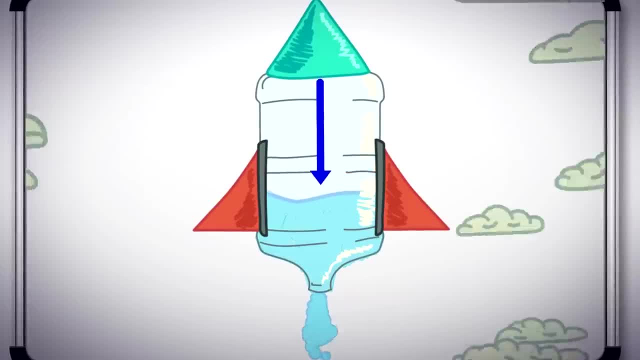 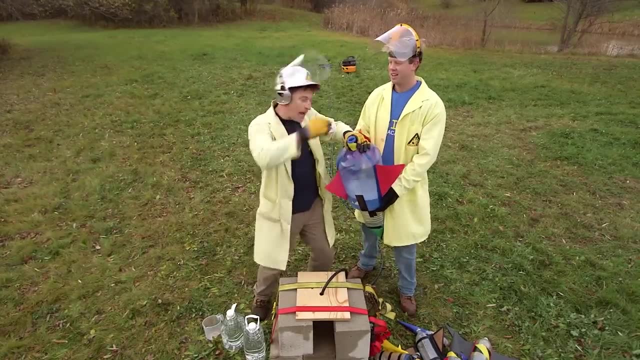 which is a very cool way of saying that eventually the cap will break and the bottle will shoot into the sky. 20-litre water cooler jug filled with some water- This is the cap that'll work, sort of like the cork We put the air pressure in there. 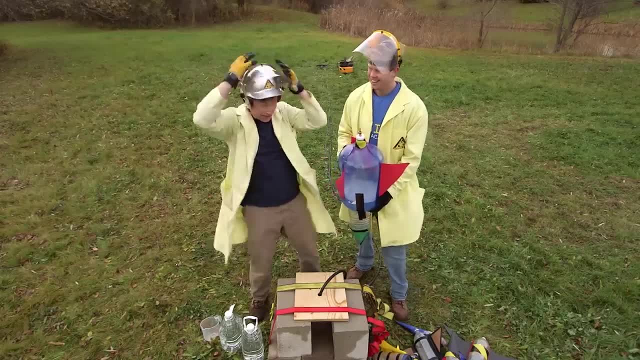 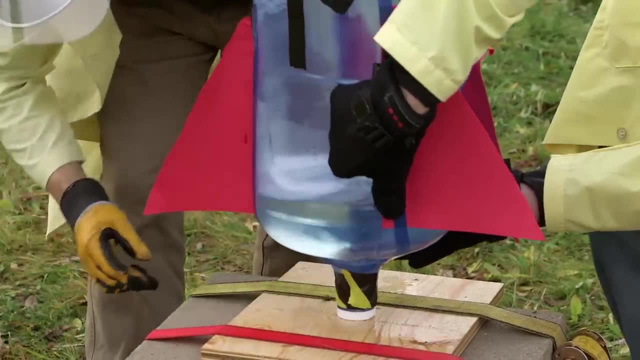 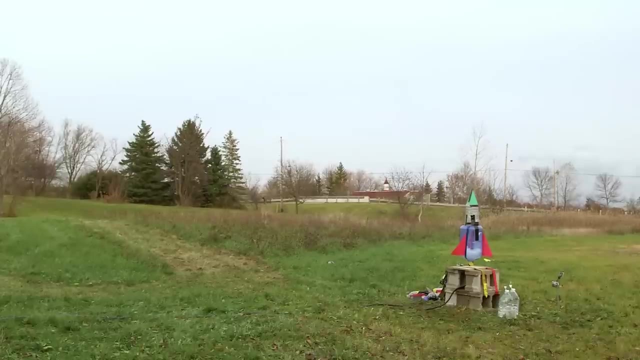 the cap can't take it anymore, pops off and the thing flies. hopefully Let's find out. Okay, that looks good There. Let's do this, Go for pressure. Uh-oh, Uh-oh, Oh no. 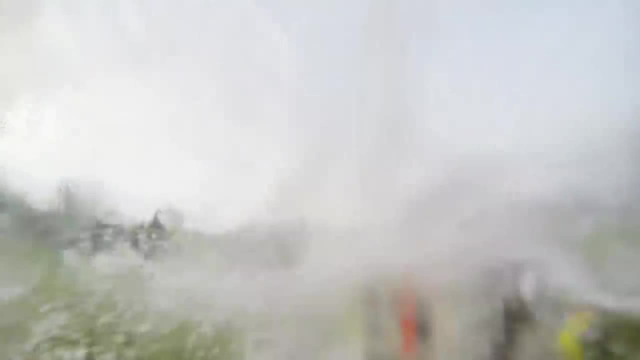 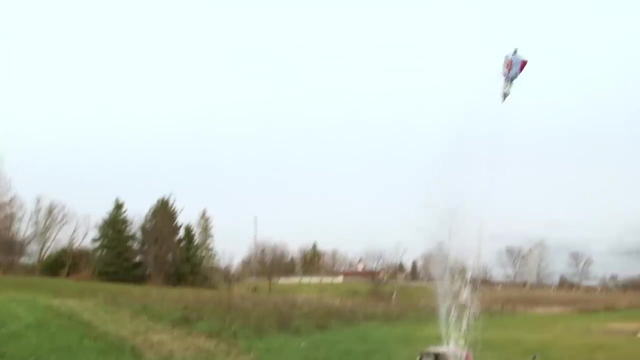 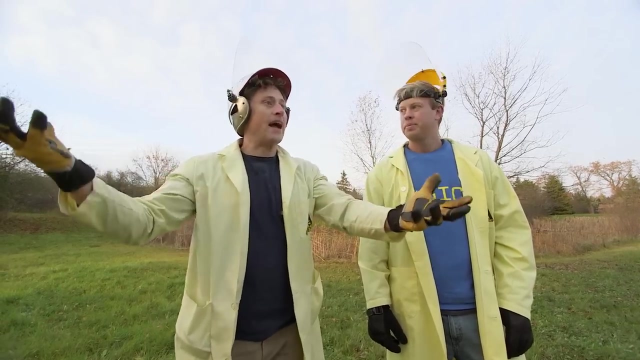 Whoa Hilarious. That worked pretty well. It sort of does that. I wonder if it's aerodynamic? No, No, So how do we? What else can we do? What else can we do to make it even more maxed out? 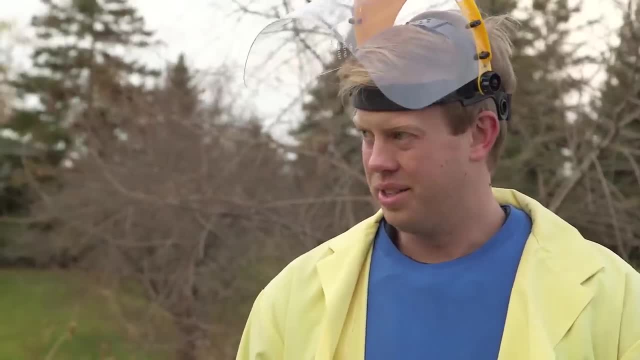 I think we can use the 2-litre bottles. They work really well. The 2-litre bottles are the best right, I think so. So what do we do? We can probably stack them. We stack them on top of each other. 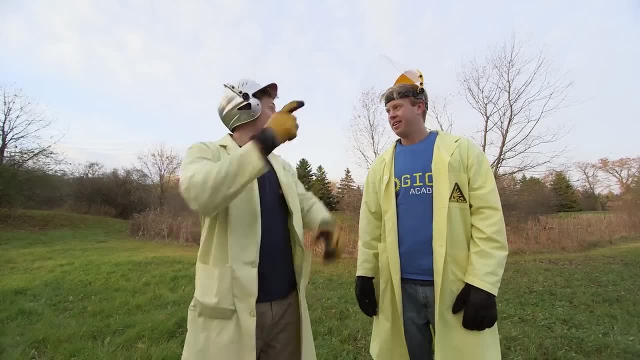 Yeah, That'd work, I like that. So we put a whole bunch of them together. Yeah, Tell you what I'll do you one better. Why don't we use three stacks? Awesome, We'll use three stacks, three launchers, three times the thrust. 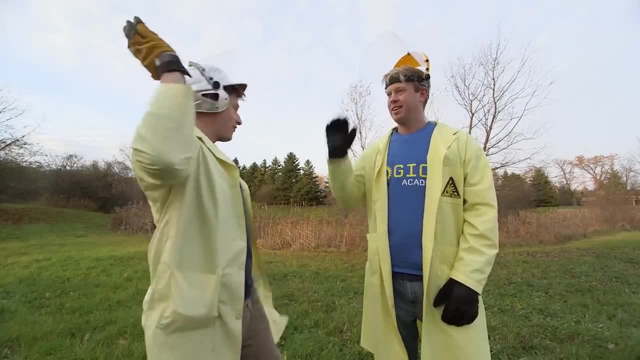 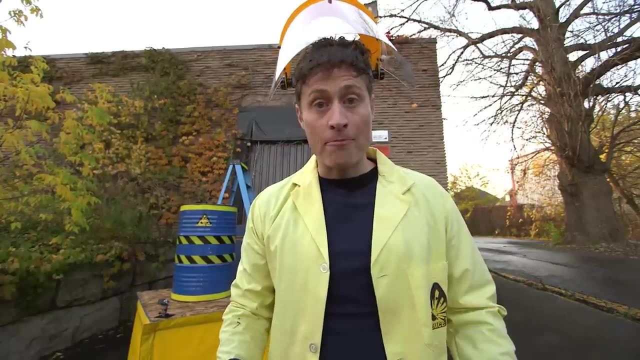 and we'll make a giant rocket out of a 2-litre bottle. Yeah, great idea. High fives, Here we go. Gas molecules get further apart when you warm them up and closer together when you cool them down. So what happens if you keep cooling them down? 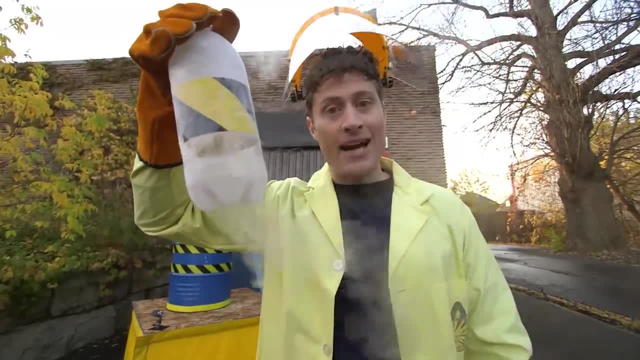 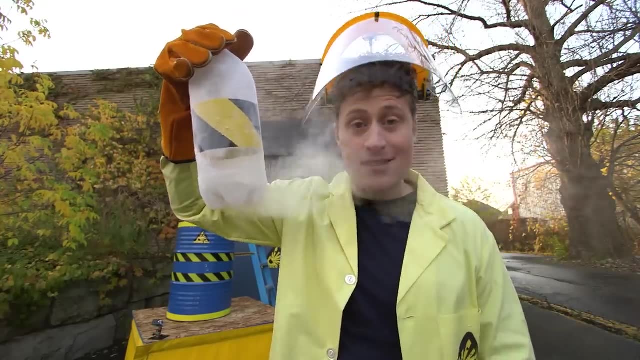 Well, they turn into this. This is liquid nitrogen. Nitrogen makes up 78% of the air we breathe, but when you cool it down to minus 196 degrees Celsius, it turns into a liquid. It's boiling right now because at room temperature. 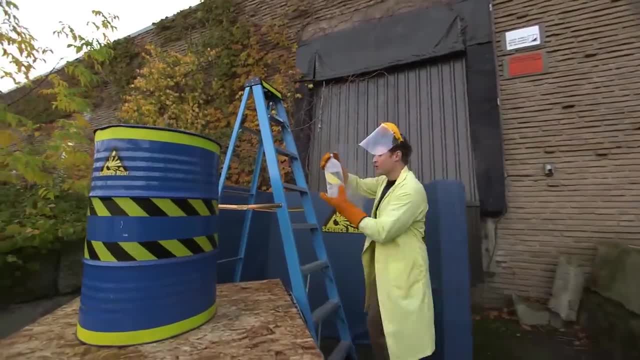 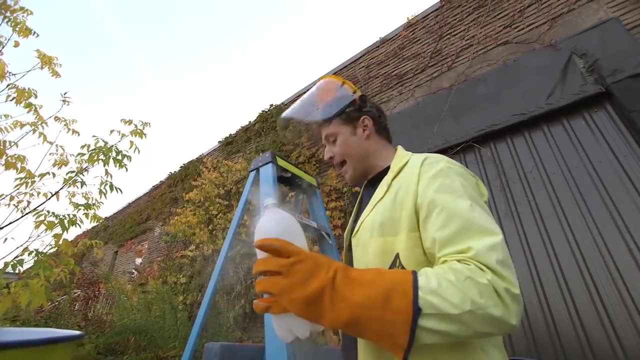 nitrogen wants to be a gas. So the liquid nitrogen is turning into gaseous nitrogen and all of the extra molecules are escaping through the top of the bottle. So what happens when you cool them down? So what happens if I put a cap on the bottle? 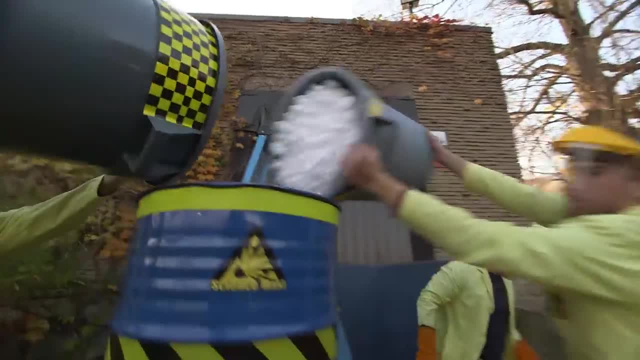 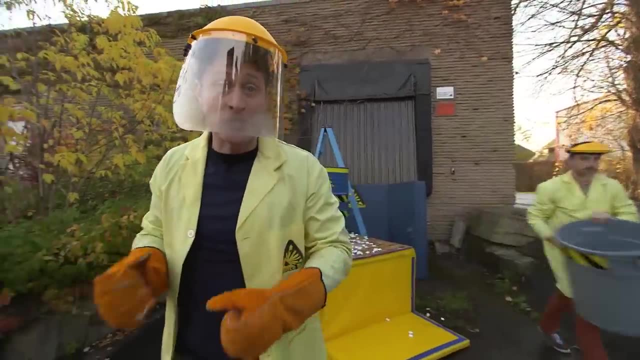 Right now the liquid nitrogen is turning back into a gas, but because there's a cap on the bottle, the gas has nowhere to go, So the pressure is just going to keep building and building until the plastic bottle can't contain it anymore. 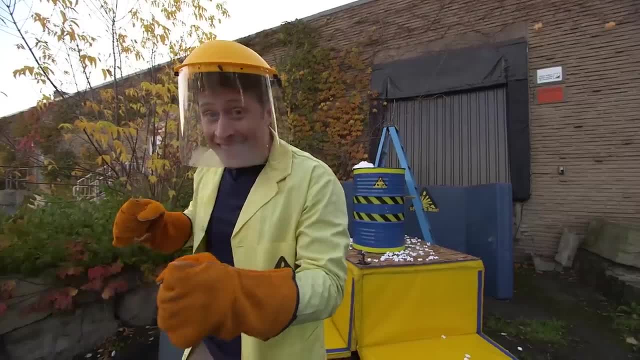 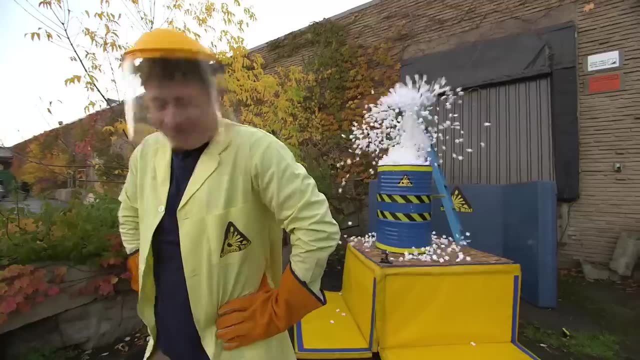 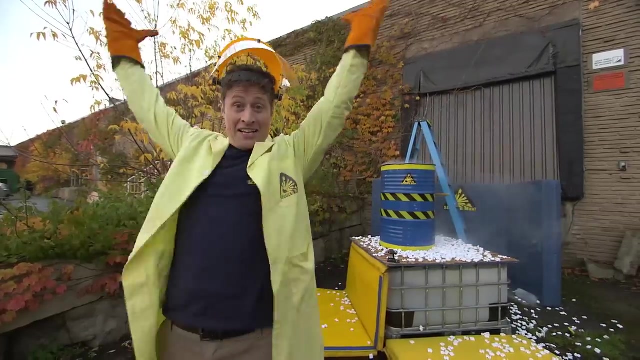 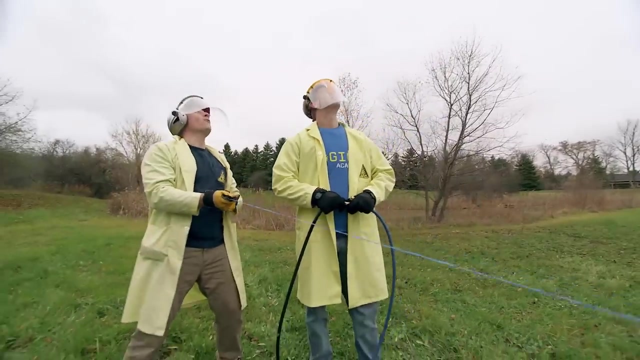 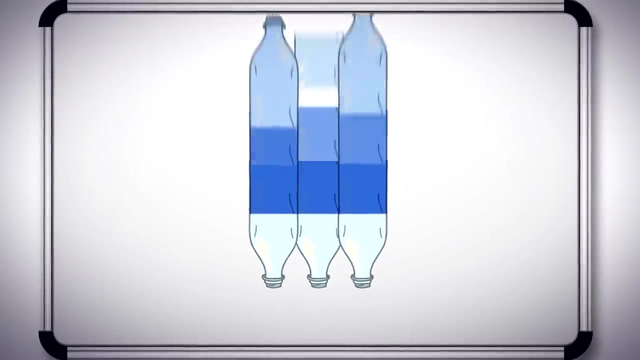 and, and, and, and. It pops like a balloon. Science 丽 Miyا вопросы. Our rockets have gone from small to bigger, to even bigger. Now the plan is to use three 2 litre bottles and create columns of them. 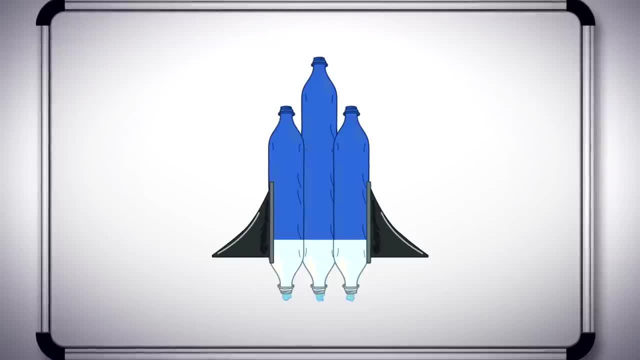 into a giant rocket. We pressurize them just like we did before, but with more thrust it might work even better. all over the place, I can make a giant rocket with this. all over the place, I can make a giant rocket with this. 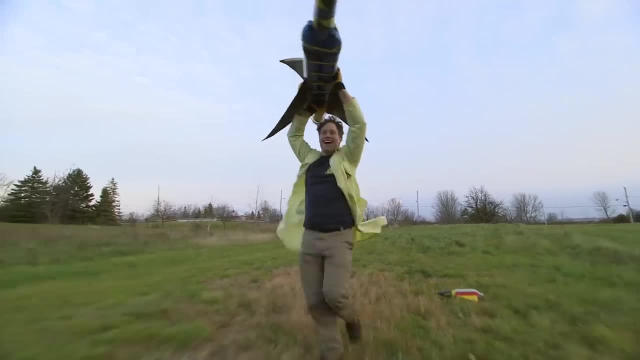 over more filters and lines and it might work even better all around the spaceship. Even if it doesn't work better, I'm pretty excited about this new plan, Giant rocket. 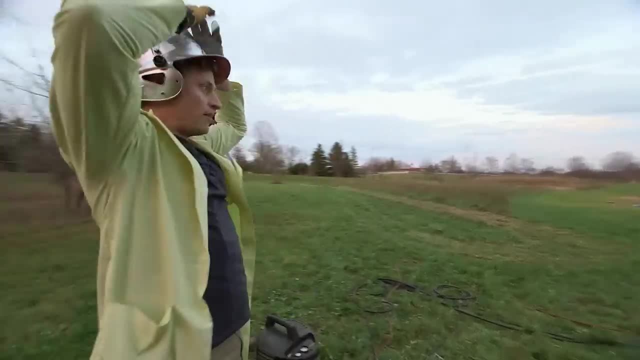 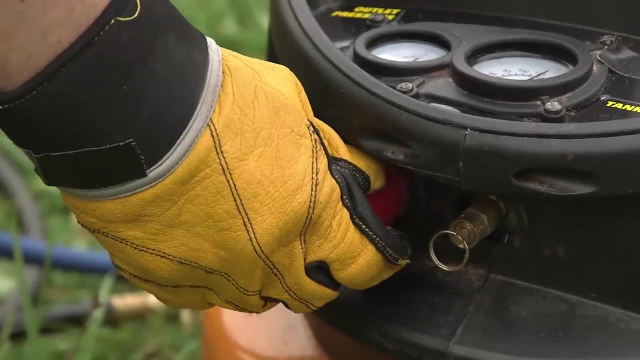 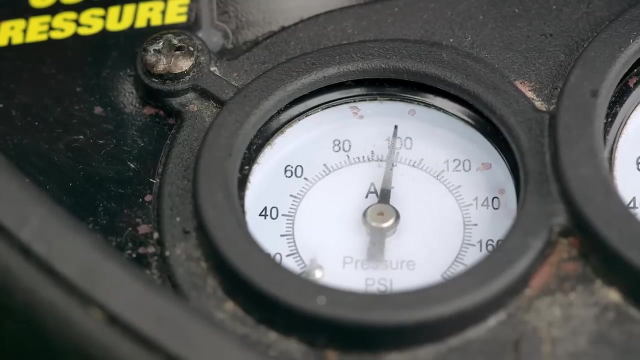 Giant rocket. You ready, I'm ready. Okay, blast shield's down. Connecting hose. Dialing up pressure Pressure is rising. It's bubbling, Bubbling, 100 PSI. Okay, stand by to fire. Three, two, one. 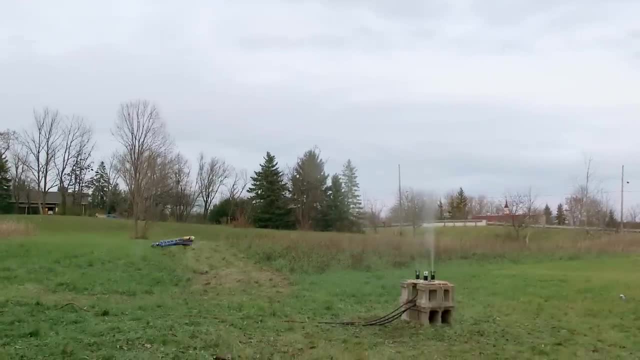 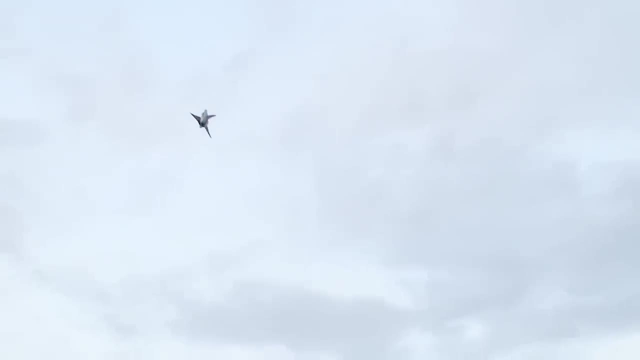 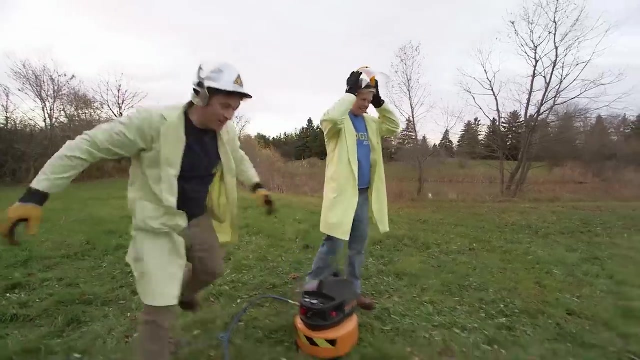 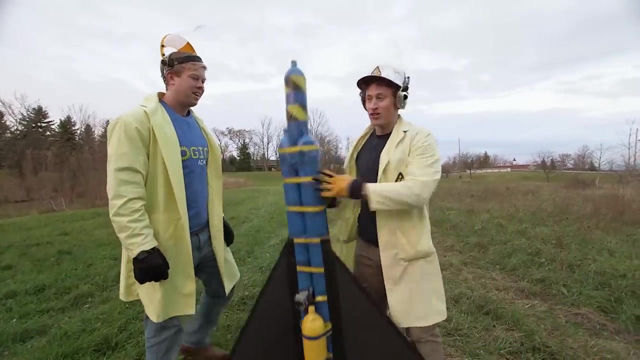 Whoa Woo-hoo-hoo, Whoa Woo-hoo-hoo. Awesome, Yeah, let's go check it out. Well, there you have it. Rocket Science, Max Experiments at Large. Well done, Nicely, nicely done. 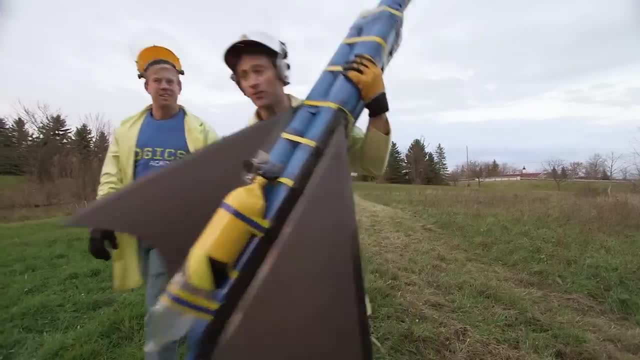 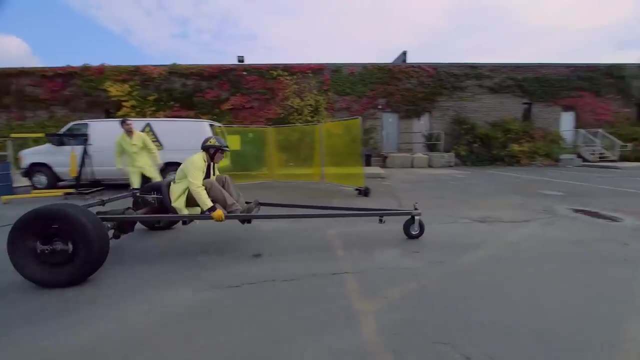 Do you think we can fire it again? Yeah, it looks like it needs some repairs. though Put on your helmets. for this episode of Science Max, We try to build a human-sized cart powered by inertia Plus Newton's laws, from a caveman to crockery. 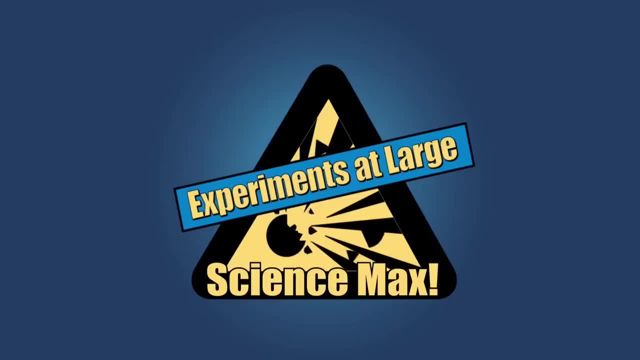 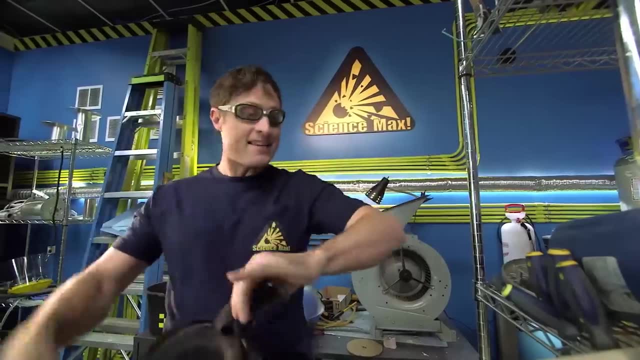 Inertia on Science Max Experiments at Large. Greetings race fans and Science Maximites. I am Phil McCordick and this is Science Max Experiments at Large. Today, we're going to be experimenting with the Drag Racer. 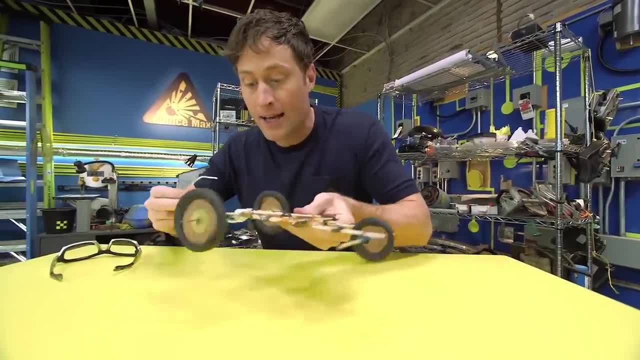 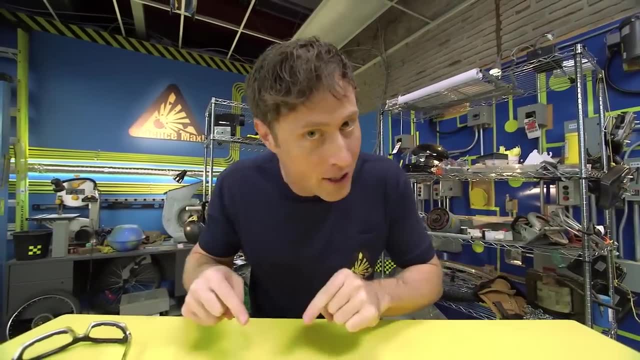 Huh, Pretty cool. It works like this: You pull the string and get the wheels going really fast, and then you let it go and it just drives away on its own. The interesting thing is, I don't have to push it. 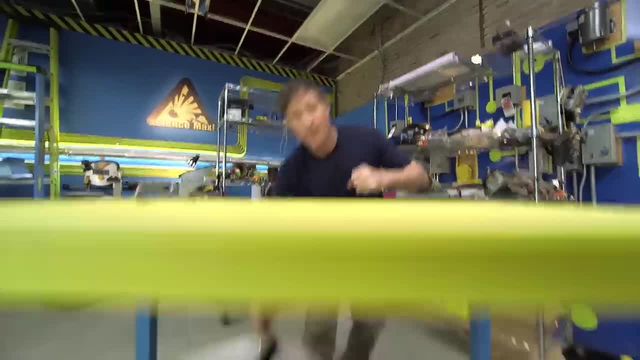 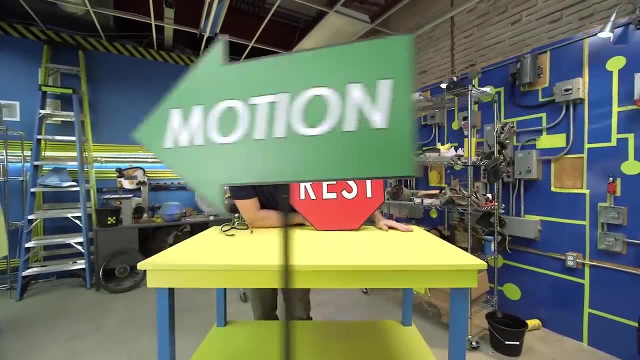 It goes by itself. It all has to do with Newton's first law of motion, which is An object at rest. An object at rest tends to stay at rest, and an object in motion tends to stay in motion. Uh yeah. 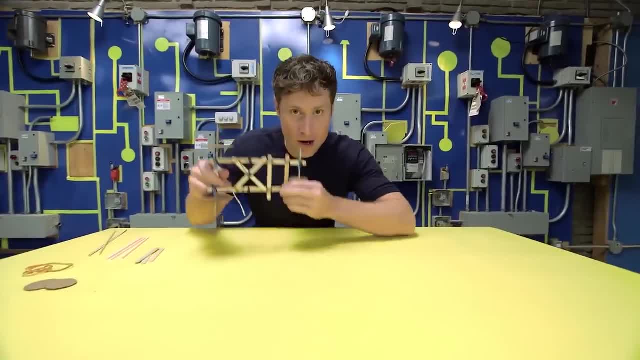 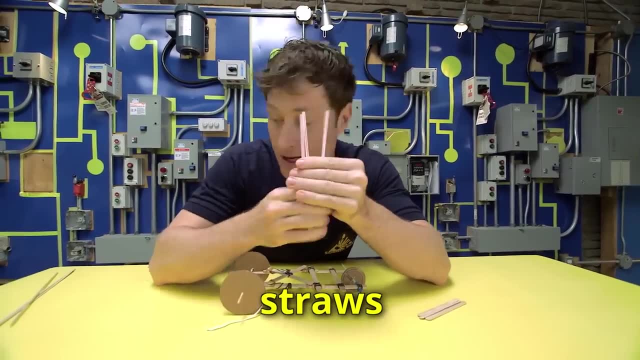 Let's get building. Here is everything you need to build your very own dragster. You need some popsicle sticks, some straws and some shish kebab skewers. I love these. You can get these at the grocery store. 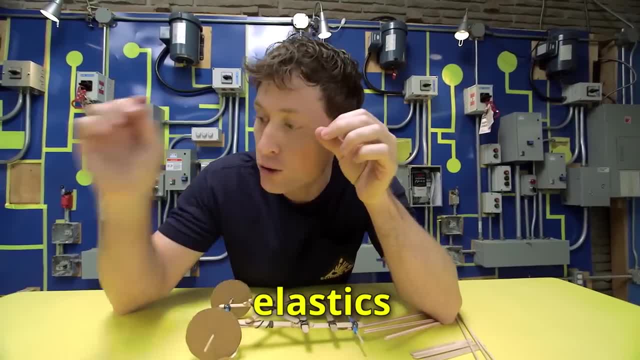 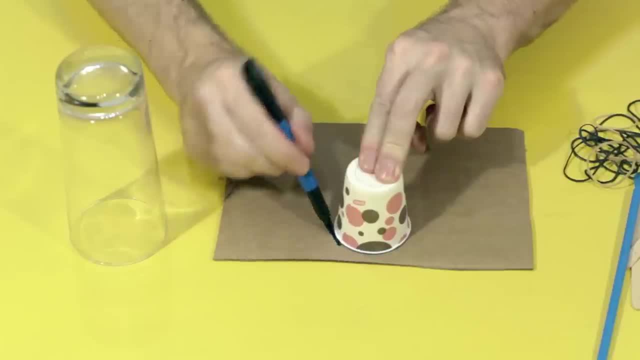 Let's see Some elastics. and of course you want wheels, and I just cut my wheels out Out of cardboard. So here's a quick explanation of how to build your dragster. First, use anything round to trace three circles out on your piece of cardboard. 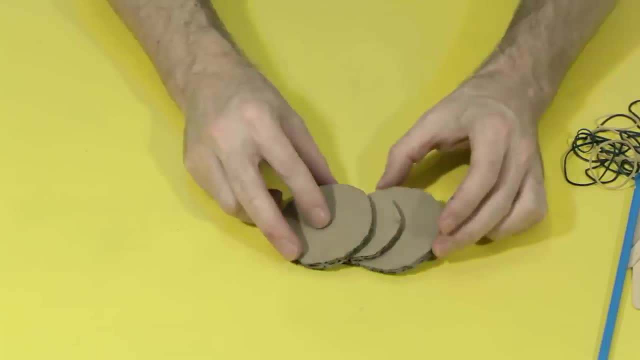 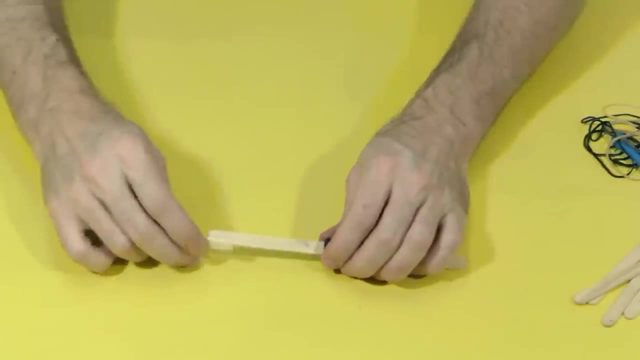 Remember you want two big and one small circle. Then cut out your wheels. Then it's time to make the frame of the dragster using popsicle sticks and elastics. Just put two popsicle sticks together, then wrap the elastic band around them to keep. 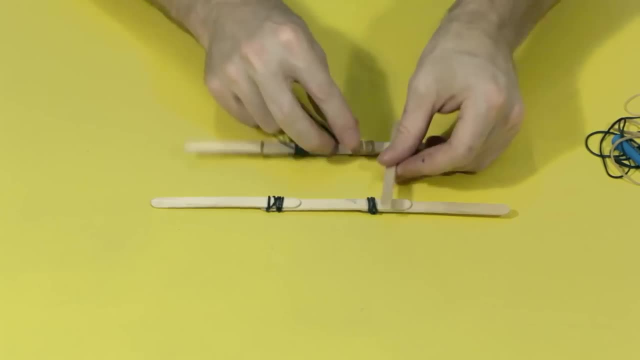 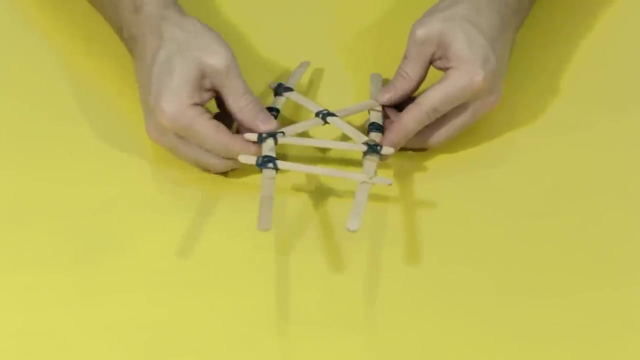 them together. First you build one side, then the other side, Then add some pieces across the middle to give it support. Remember not to put everything together. Remember not to put any popsicle sticks too near the ends, because they'll get in the. 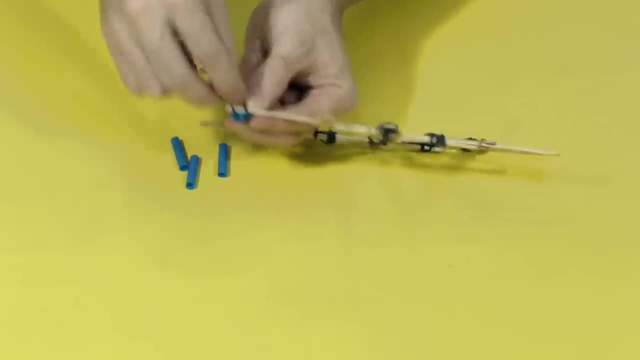 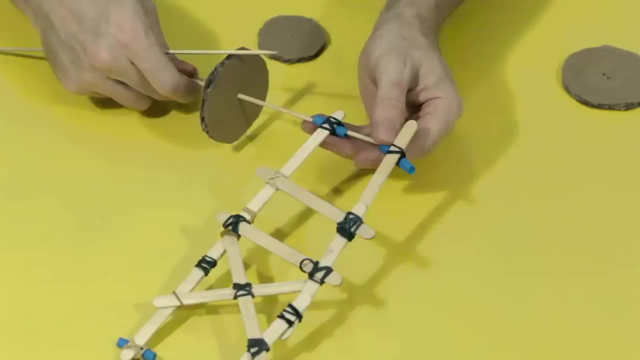 way of your wheels. Next, cut the straws into small pieces and use an elastic band to tie them to the ends of the popsicle sticks. Then it's just a matter of sticking the shish kebab skewer in a wheel, passing it through. 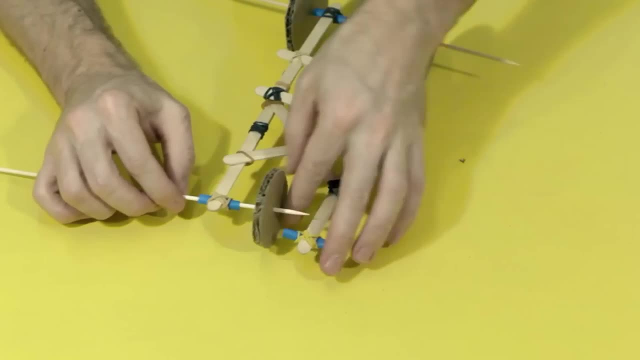 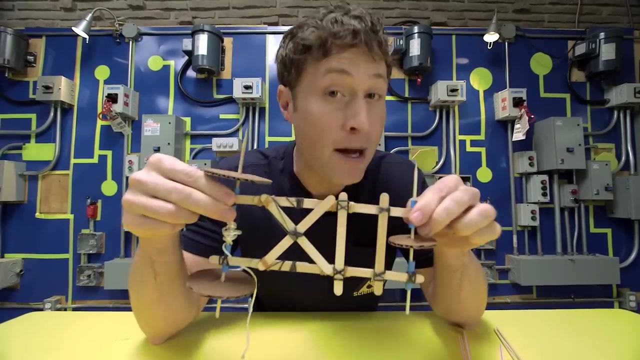 the straws and sticking on the other wheel. Don't forget that the small wheel goes in the middle, at the front. You can trim the skewers afterward by just breaking it off short. If you want step-by-step directions on exactly how to do this, you can go to our website. 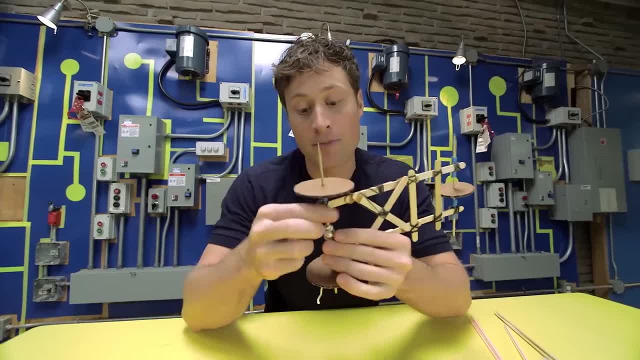 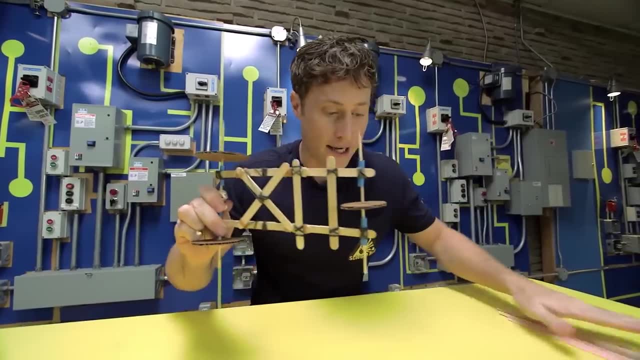 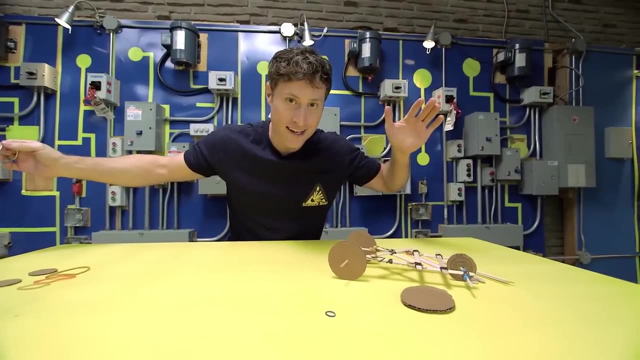 I'll see you next time. It's all right there. Now the last part is wrap some string around the back axle so you can pull and the wheels will spin. Let's check it out and see how it works. Didn't work that well, did it? 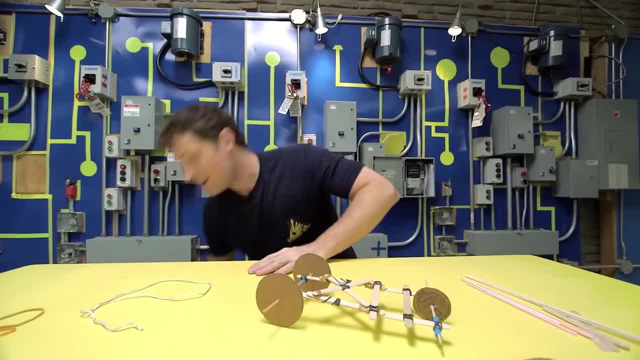 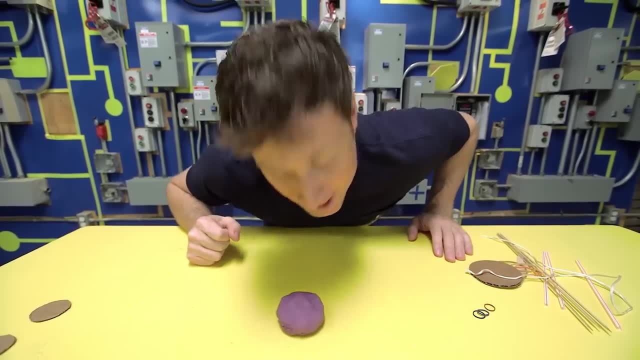 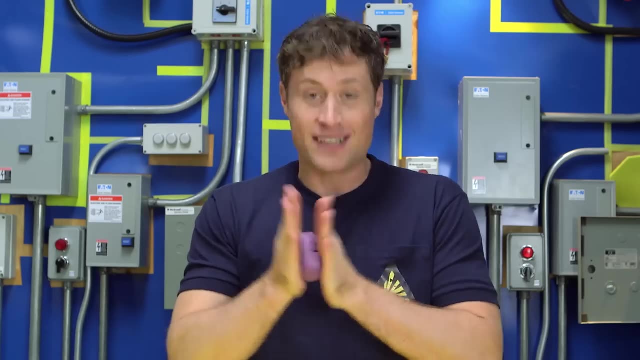 That's because we haven't added the secret ingredient Plasticine, the perfect secret ingredient for all of your dragster needs, And also sculpting, Because that's what it's for. Remember how I said: an object at rest tends to stay at rest and an object in motion tends. 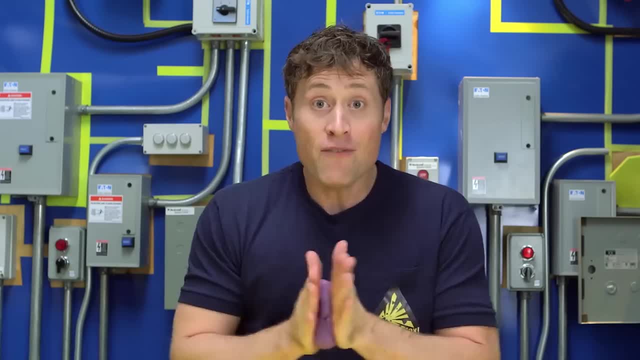 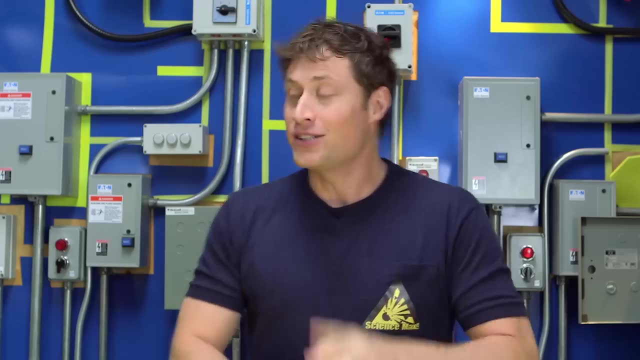 to stay in motion. Well, the heavier something is, the more force you need to change its direction, either get it moving or make it stop. That is called inertia. It's the tendency for an object to resist the change in motion, either getting it going. 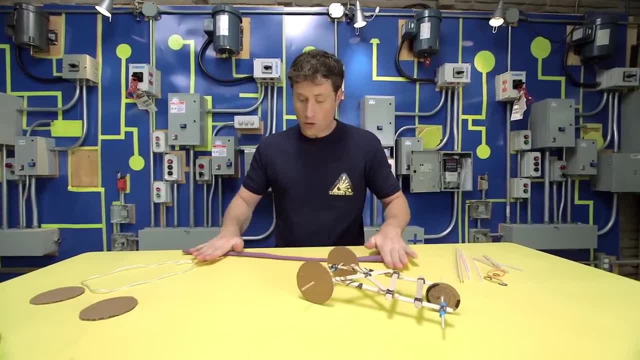 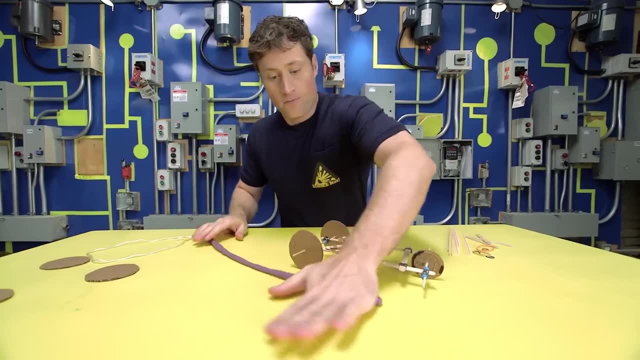 or making it stop. So the heavier we make the wheels of our dragster, the more they will resist Or they will resist a change in motion. So what I've done is I've stretched out my plasticine and then you roll the wheels of. 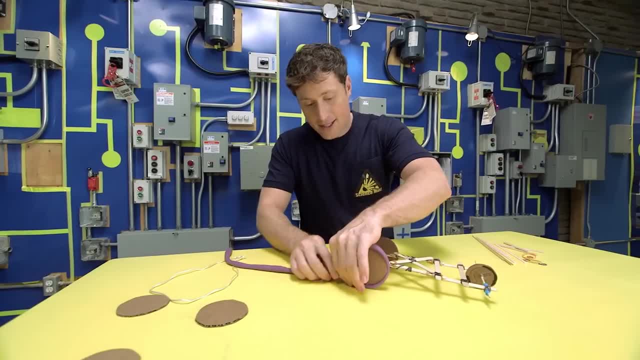 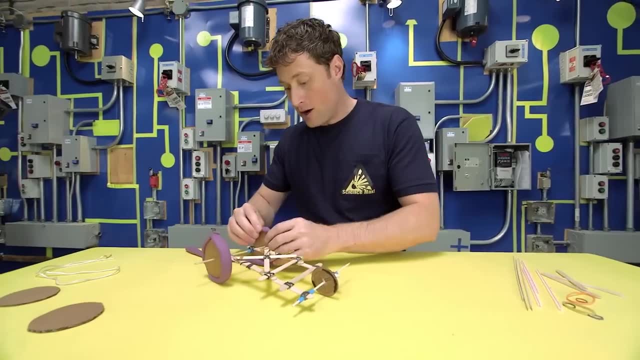 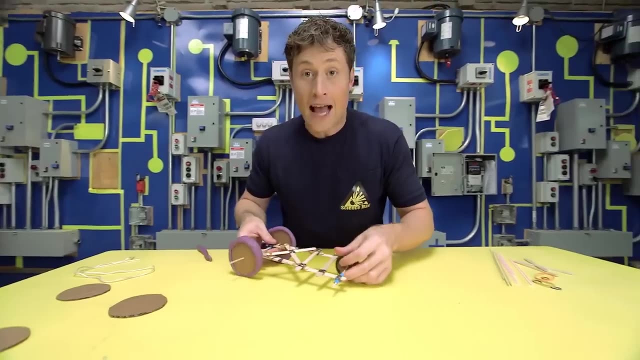 the dragster around in the plasticine and this will make each wheel way heavier than just the cardboard by itself And it will make it much better in terms of keeping the dragster going, because if the wheel has more weight it will have more inertia. 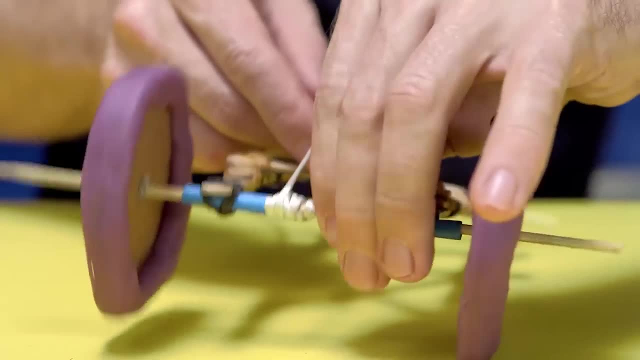 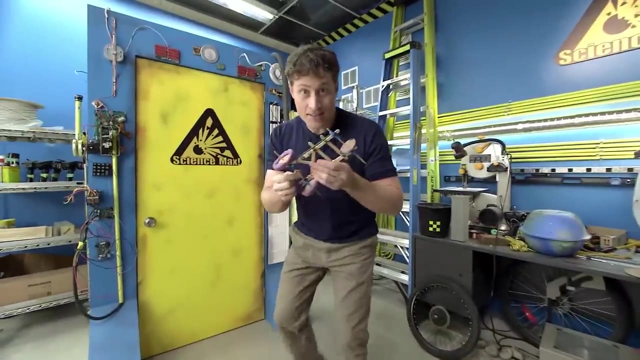 Now I have to wrap the string around the back axle, just like that, And there we go. All right, Let's try it out. All right, Let's give it a shot and see how it works. Pull on the string, get the wheels going real fast and there it goes. 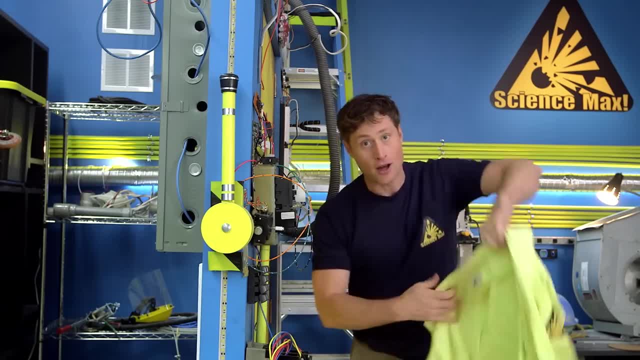 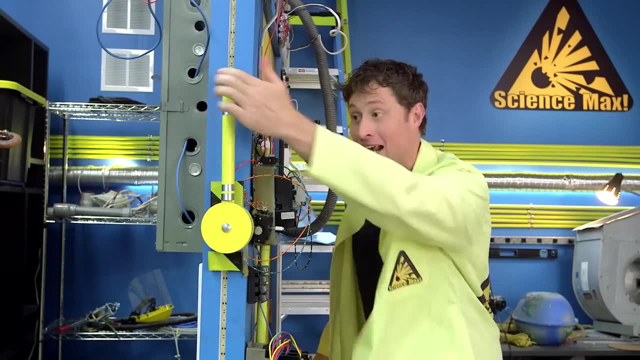 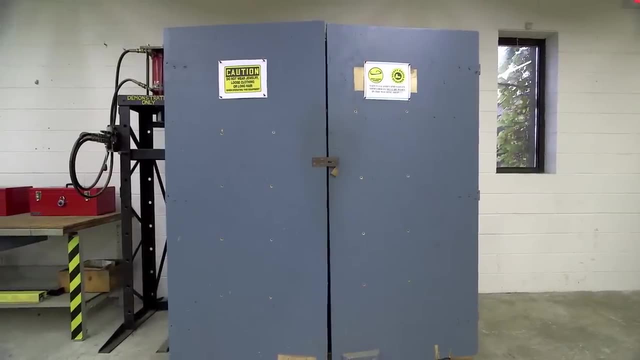 Now, of course, this is Science, Max, Experiments at Large, and we are going to do it again, and we're going to do it much, much bigger. That's why I'm going to the Center for Skills Development and Training. I thought it was bigger. 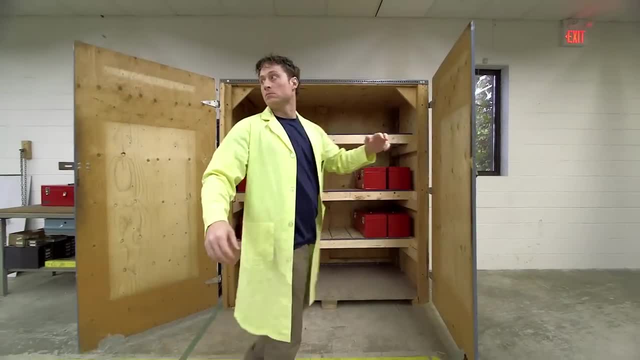 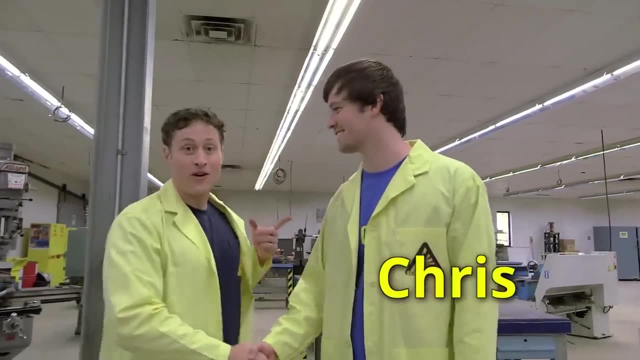 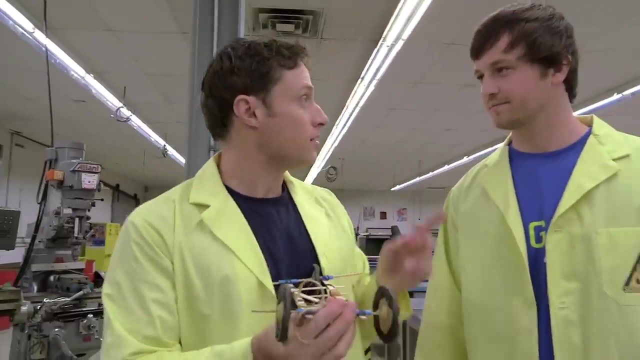 Oh right, Hey Chris, Hey Phil, How you doing? Chris is from Logics Academy, Logics Academy, And he is going to help me max out our dragster Now. you guys at Logics Academy go into schools and build all kinds of cool stuff with the 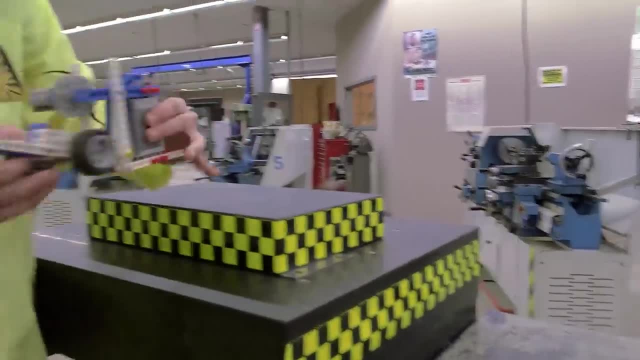 students. right, That's absolutely right. This is our dragster over here, actually, And this one has an electric motor. Oh yeah, It's kind of fun And these gears touch, Ooh, Wheels get going. I like that. 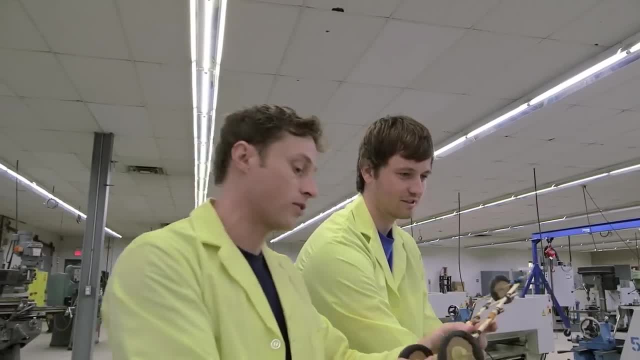 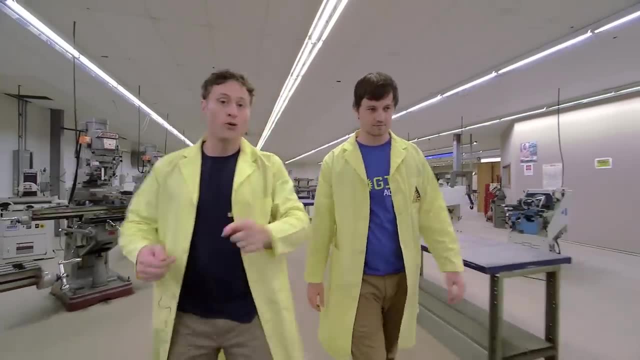 And All right. See, our dragster works on good old human power. You pull the string and there it goes. Now you have a physics degree, right, I do, Which means you know Newton's first law of motion. 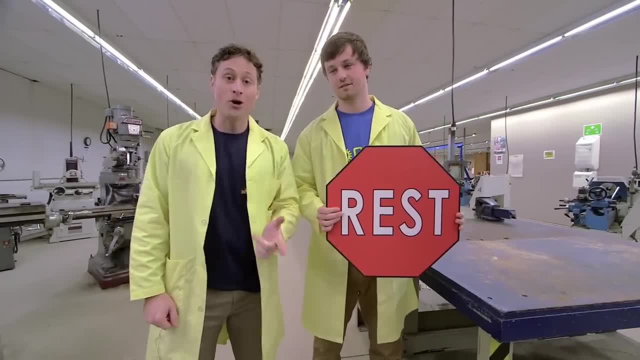 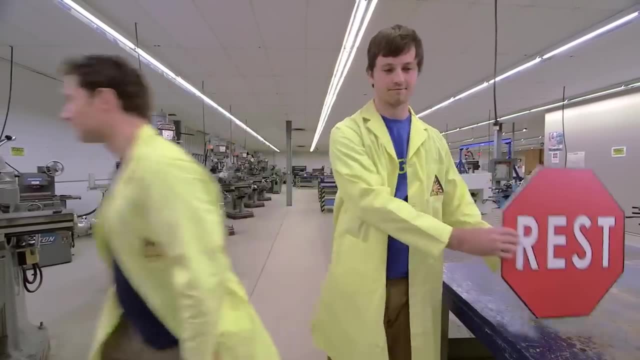 Of course, An object at rest tends to stay at rest And an object in motion tends to stay in motion. I thought it was going to come from over there. Yeah, Come on. All right, Chris, I want to make a dragster big enough that we can ride. 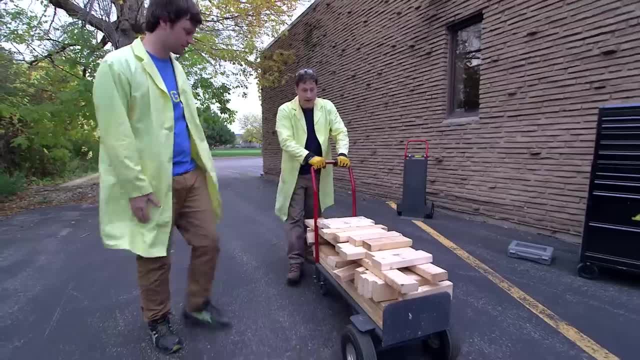 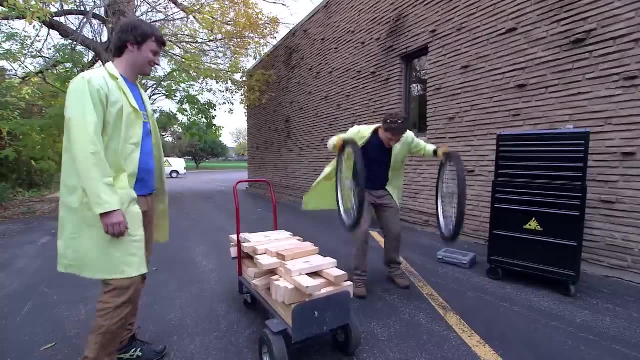 Whoa, Okay. Well, it's going to have to be pretty big. Yeah, I think we have enough wood, though, right? Yeah, Looks like it. Oh, look, I've got some wheels. Perfect, These are bike tires. 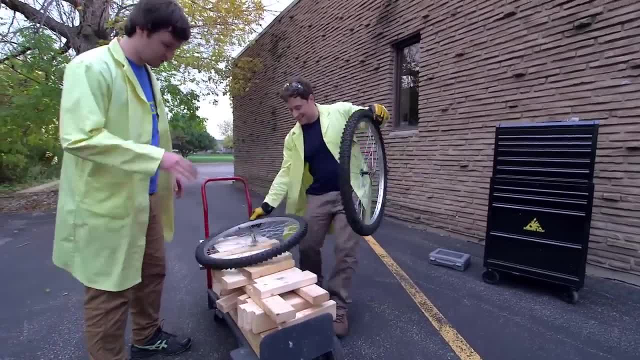 And I filled them full of air, so they're bouncy. Check it out. Excellent, Whoa, Okay. So, yeah, We build our frame out of wood. Yeah, Attach the tires on and then find a way to get them spinning. 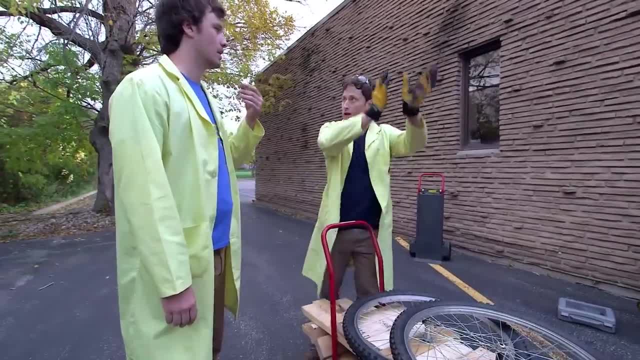 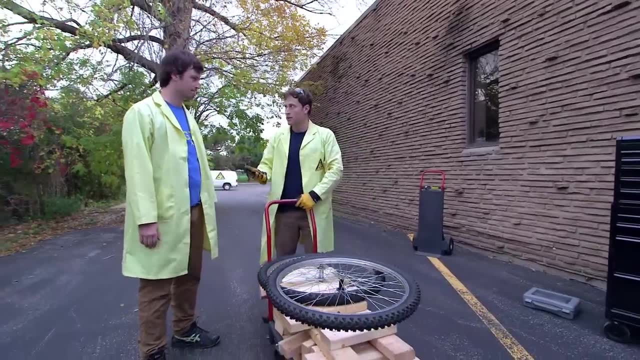 And if the tires are spinning, Yeah, we don't actually have to push the cart because it'll just go on its own. That's the idea. The inertia should carry, and the wheels should carry us down the track. So in this case, the object in motion is the wheels. 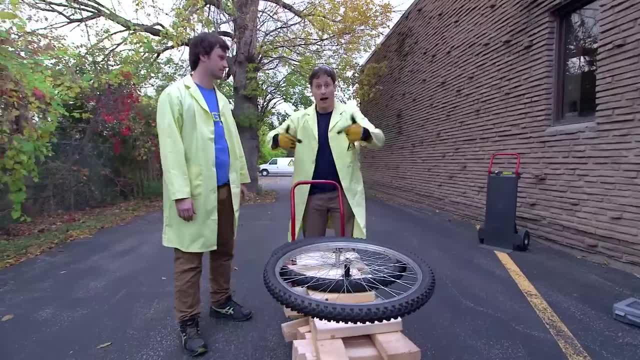 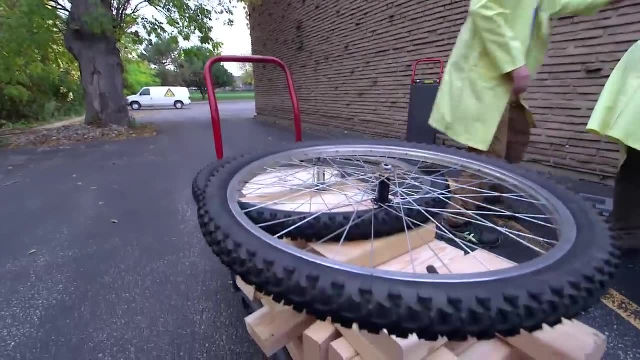 That's right. And it wants to stay in motion, which means that when it hits the ground, it'll push the cart, And hopefully us too, And hopefully us too. All right, Let's get building, Let's do it. 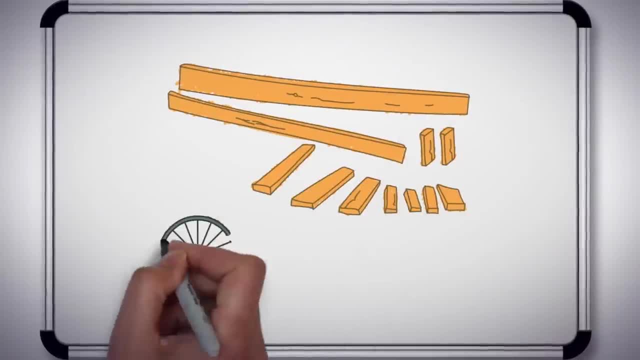 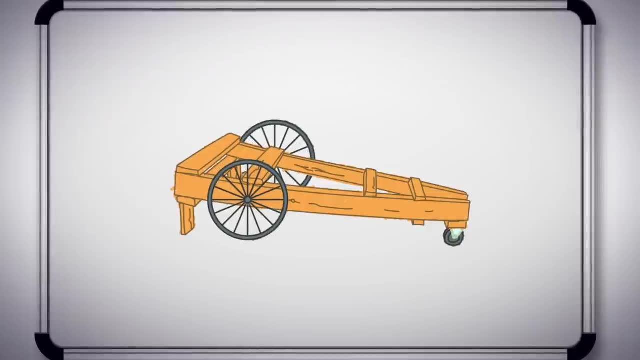 So Chris and I get to work building the dragster. Our maxed-out version is going to look just like the popsicle stick version: a triangular frame with two large wheels at the back and a small one at the front. What's more. 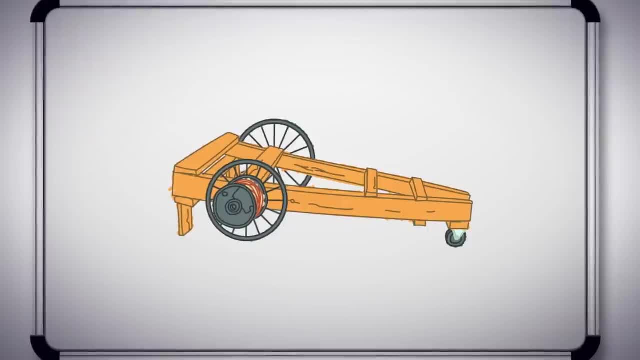 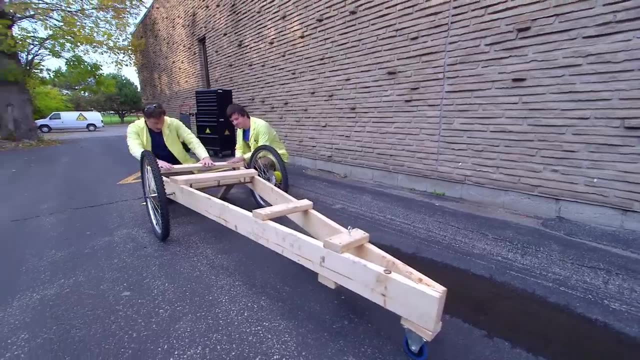 We're going to do the same thing. to get the wheels spinning, We're going to attach a rope and give it a pull When we drop it down. the inertia of the wheels should make the dragster take off. All right, Here we have our dragster. 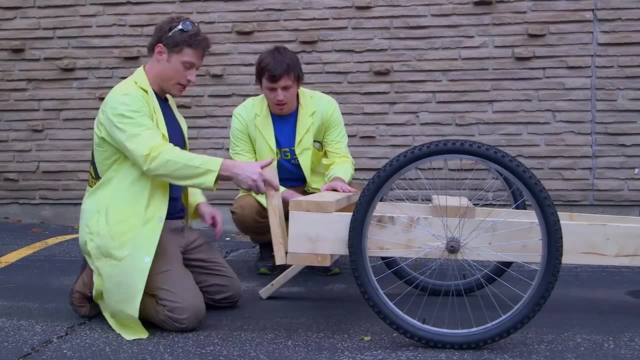 This is nice, Chris. Yeah, it looks good. So the only thing I don't understand is: what are these for, Right? So these are going to help us lift the wheels off the ground, like this. Oh, okay, Pull it back. 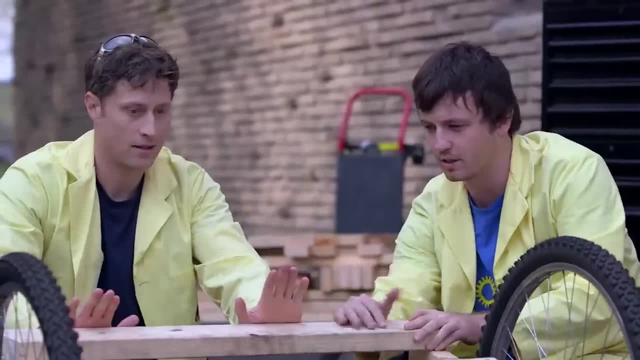 And what's going to happen is we're going to run real fast with that string and we're going to give it a little kick and hopefully it'll take off. Yeah, All right, I like it, All right. So I'm going to just run backwards as fast as I can. 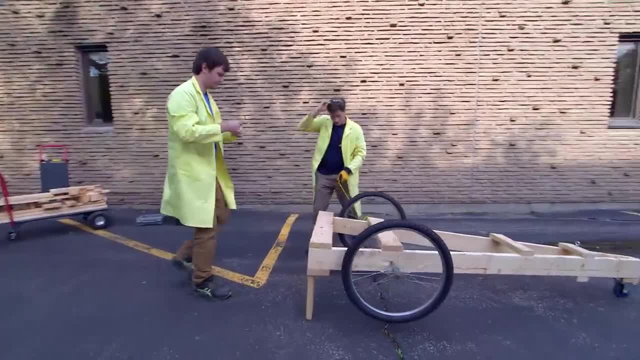 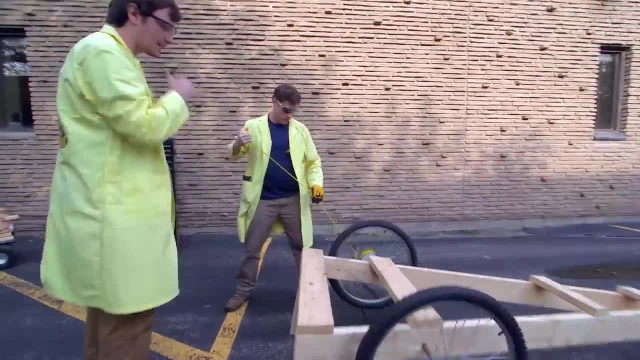 As fast as you can. All right, Here we go. Ready, Yep, Ready. Okay, Safety glasses on. And Oh wait, Did you want to sit on it? or? Oh right, Let's wait until we see it working, and then we can. 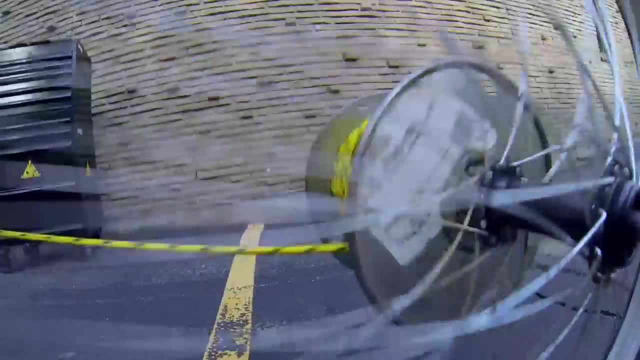 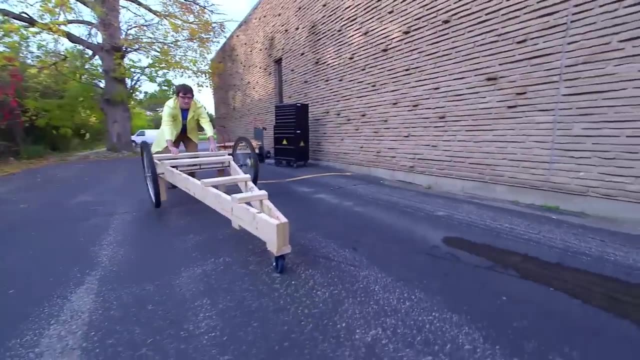 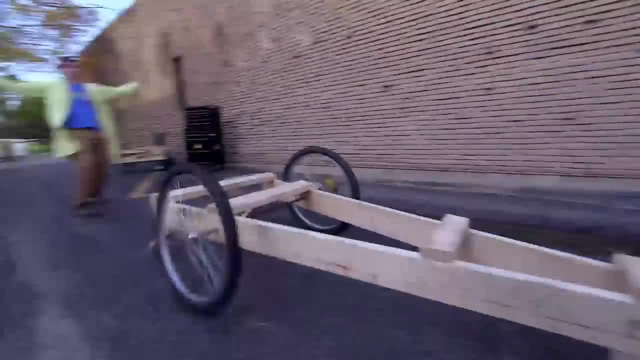 It was able to drive away from a stop using the inertia it got from its spinning wheels and a little bit from Chris's kick. That worked pretty well. That was awesome. Yeah, I think we can make it go even better. You think so? 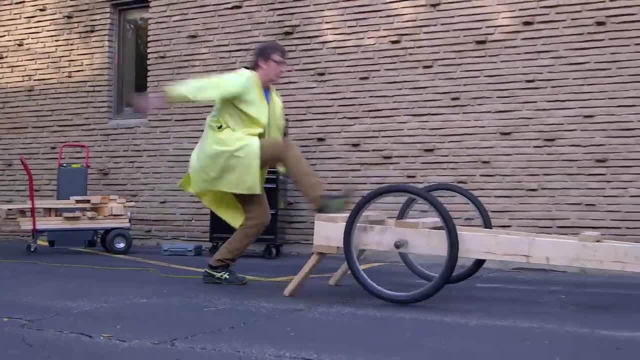 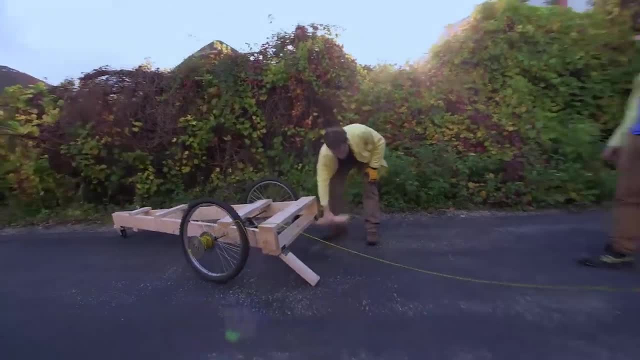 I just think we need a bit more speed. Yeah, All right, Well, let's pull it back to the start, Okay, So what? We just The wheels weren't going fast enough. Yeah, I think. so I think that you running, I mean, was great, but 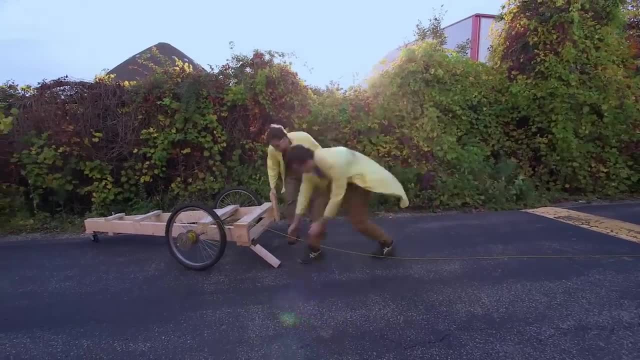 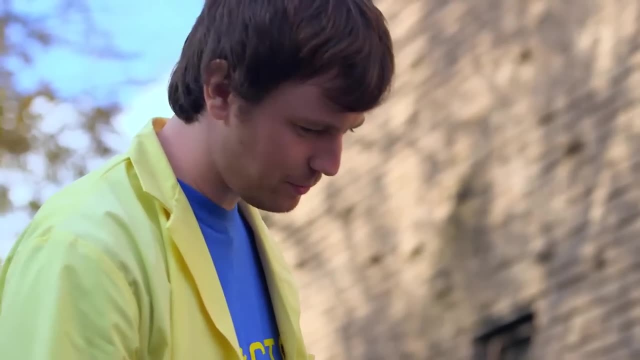 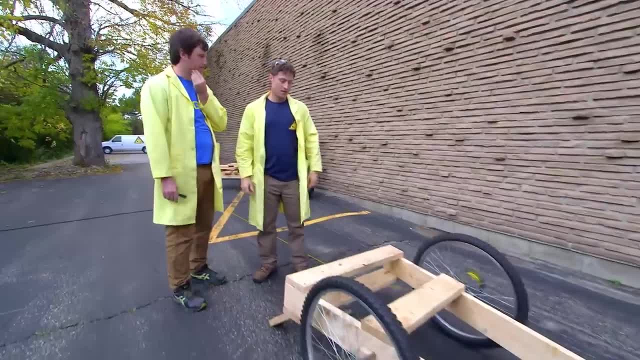 Maybe, Oh, just to get the wheels spinning fast. Yes, that's right. But what do we? I don't know how that would work. Well, I was thinking: a power drill, A power drill. Yeah, I don't get it. 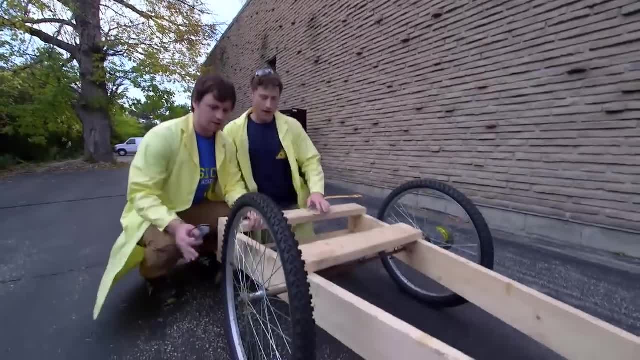 Okay, How do we use a drill? Let me explain. So we'll take a drill Right and we'll attach it right under this axle here, and that'll get the wheel spinning a lot faster than we had it before. 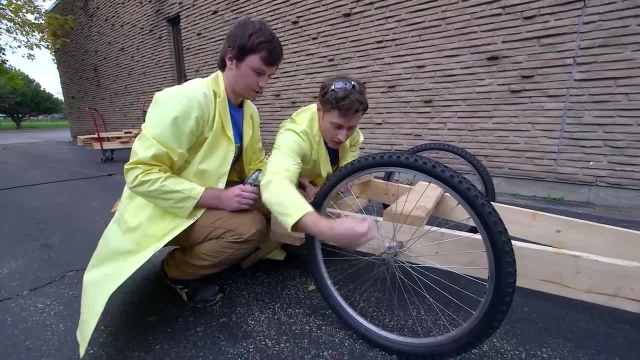 Oh, I see. So you put the drill right here at the end, That's right, and it'll spin the wheel, That's right. Oh, That's the idea anyway, And once we get it up to speed- hopefully a lot faster than before- give it a kick. 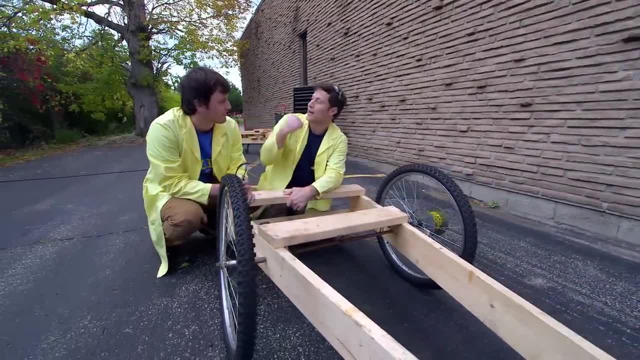 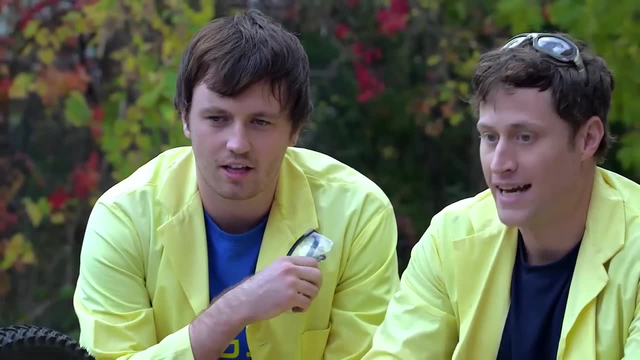 it should go a lot farther. Okay, great, So that's way better than me running all the way back with the rope. I think so. All right, Now here's the real question: Should we just go for it and have someone ride it when we do it with the drill? 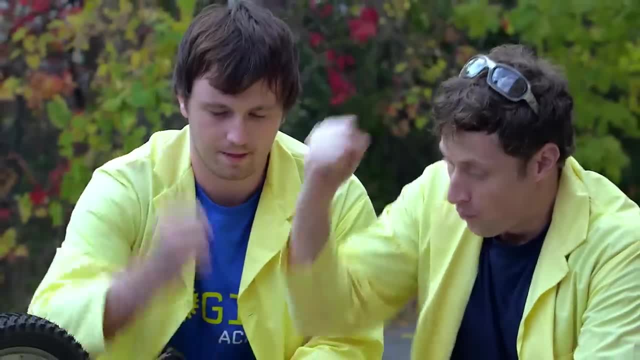 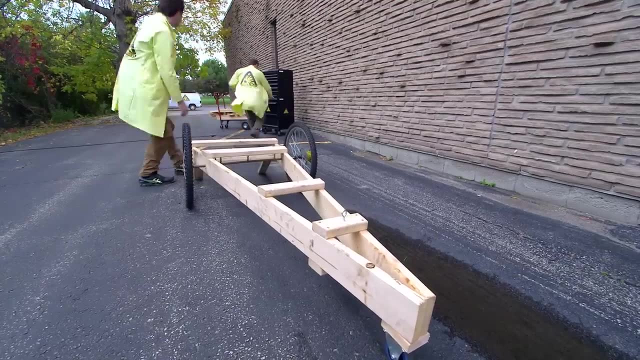 Well, who gets to ride it? Oh, rock paper scissors. Okay, Let's go One, two, three. Oh Yes, All right, I will get a drill. Okay, What kind of bit do we need? 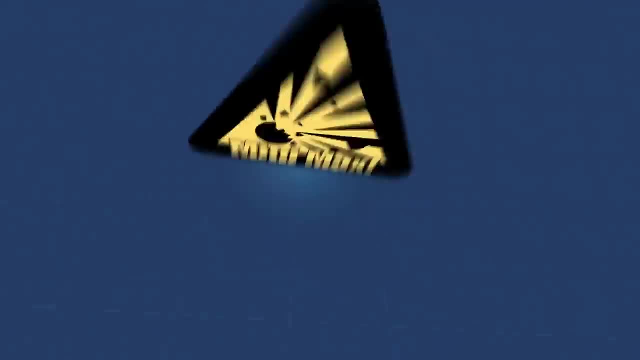 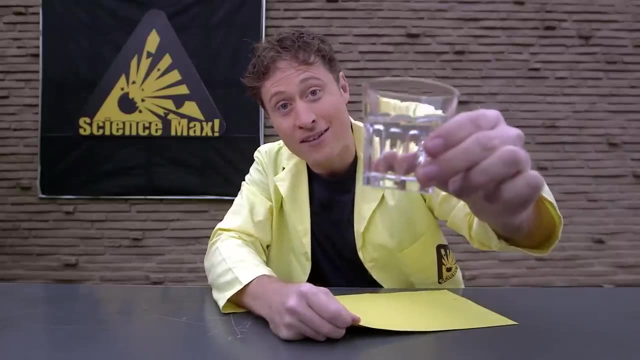 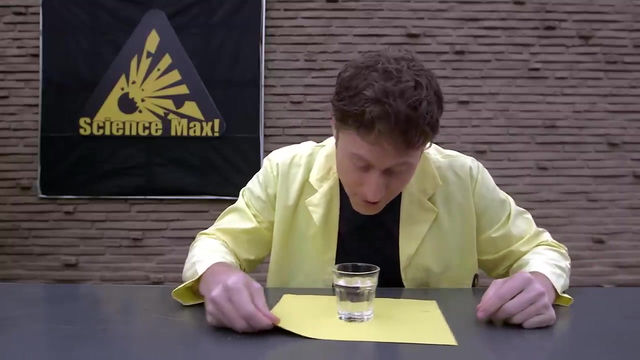 Hex bit. Okay, Let's go. Here's a fun experiment you can try. If you have something heavy like this glass of water and you put it on a piece of paper, you can experiment with inertia. If you move the paper slowly, the glass moves with the paper because the friction between 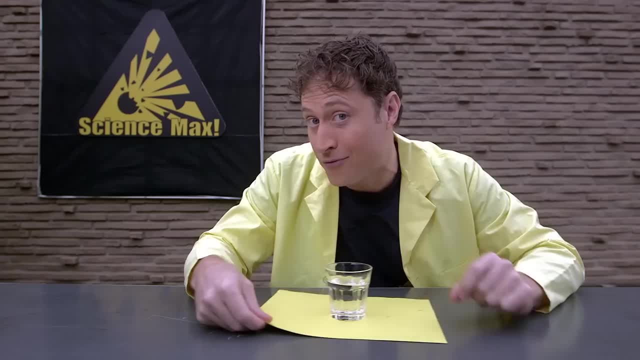 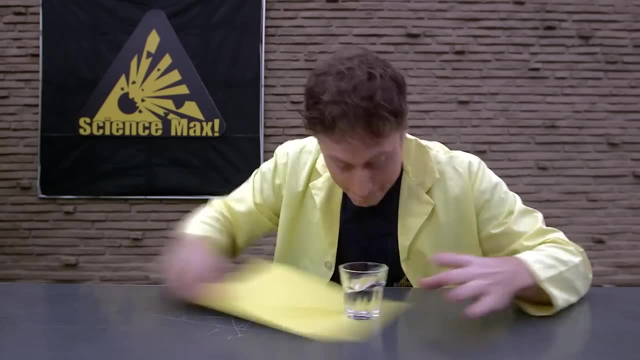 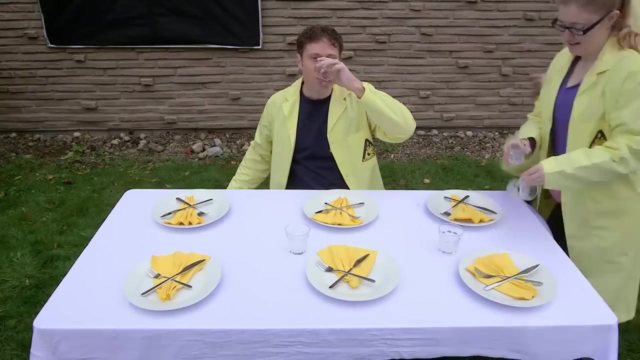 the paper and the glass is enough to overcome the inertia of the glass. but if you move the paper quickly, the friction is not enough to overcome the inertia and the glass stays there. And now let's max it out. Okay, Let's do it. 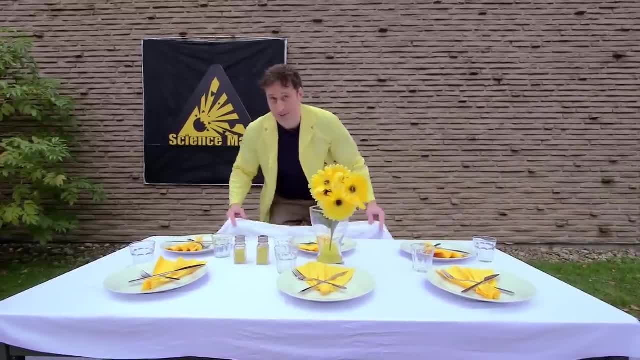 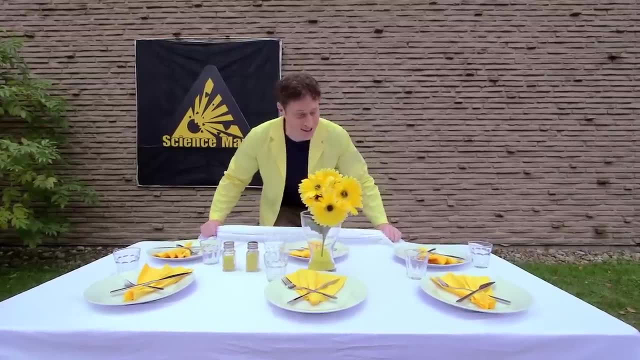 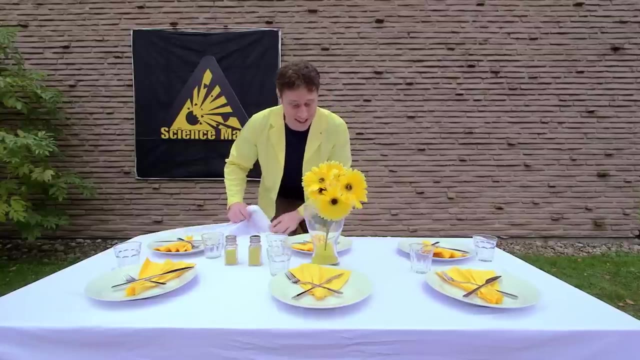 All right Now you might be tempted to try this at home, and you can, but please, for me, promise that you'll let an adult know you're about to do this and don't use breakable plates. Use plastic plates, because this will take a couple times of practicing before you get. 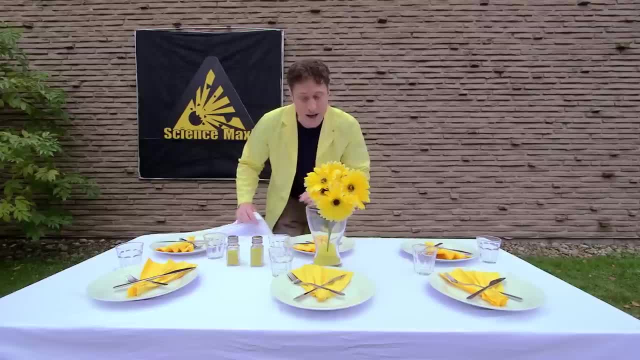 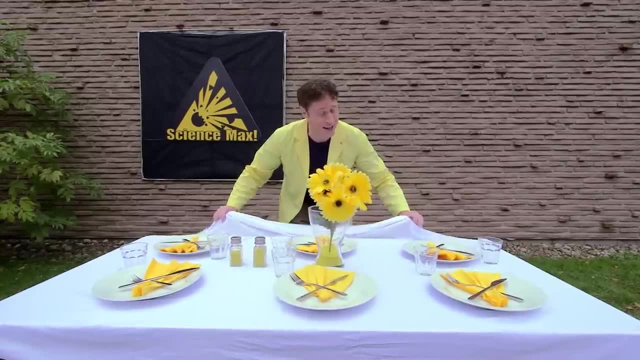 it right. Put something on the plastic plates, because the heavier they are, the better it will work. All right, Did I mention not to do this at home unless an adult knows you're doing it? I cannot stress that enough, Okay. 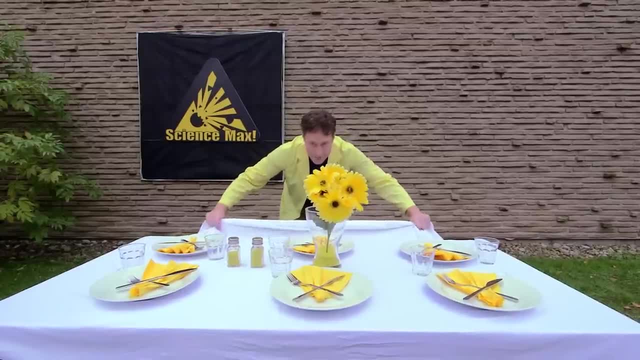 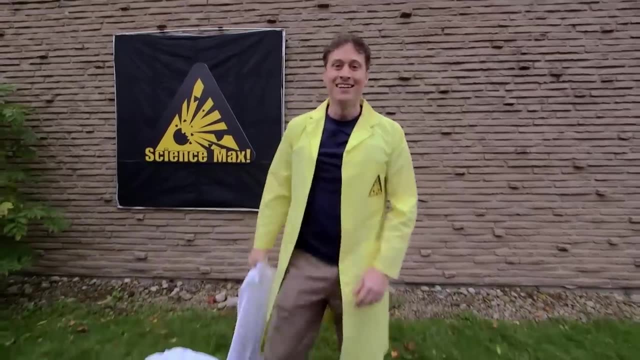 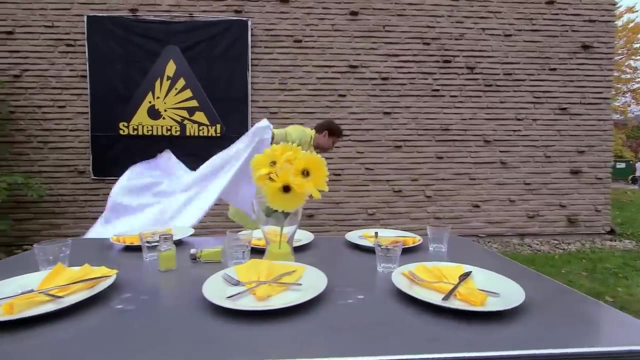 Deal. All right, Deal. Here we go, Ha-ha-ha, And there you go. Newton's first law. All right, Our dragster worked pretty well, but now we're going to try sitting on it and seeing if the 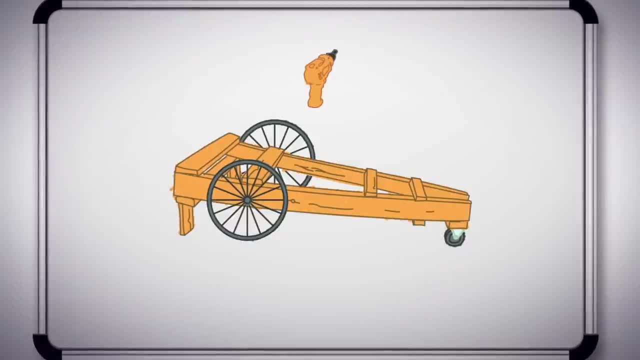 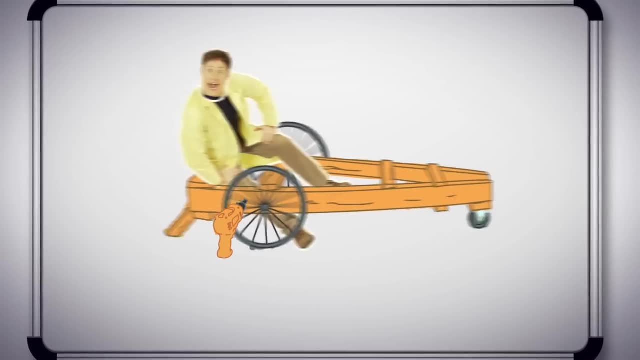 inertia of the wheels is enough to accelerate the dragster and the human rider, Because we're going to need a lot more inertia. we're going to make the wheels spin even faster using a drill. All right, Power tools. Yeah, Power tools. 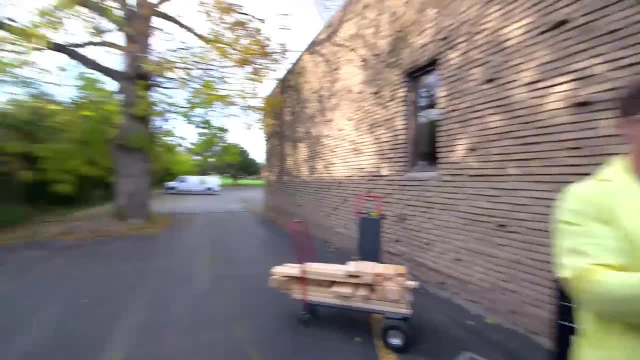 Woo-hoo-hoo-hoo-hoo. Yeah, Ha-ha-ha, All right, All right, Here we go. Ha-ha-ha, Ha-ha-ha, Ha-ha-ha, Ha-ha-ha. 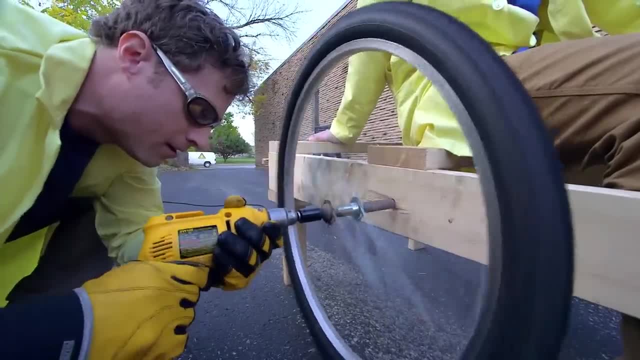 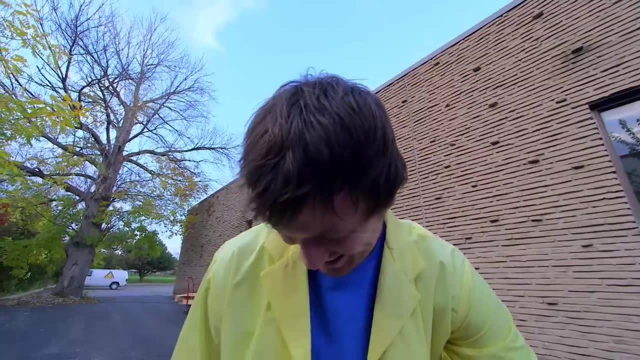 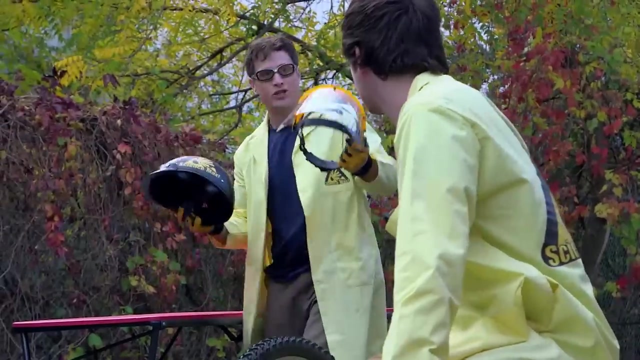 Sorry, When I attach the drill to the wheel, it works really well. Yep, That is really going to work. All right, Let's do it for real. So what do you want? Helmet or blast shield? Blast shield, Blast shield. 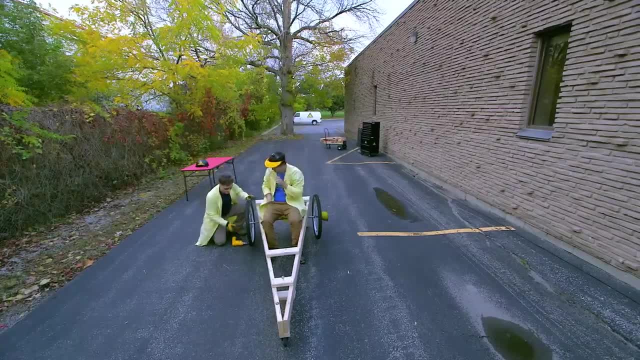 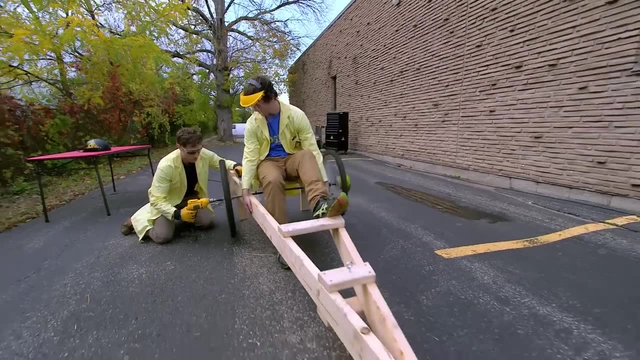 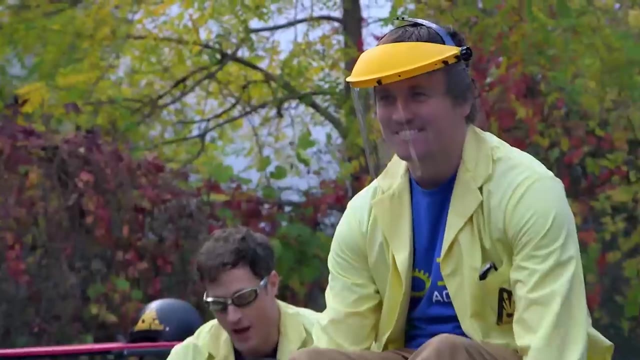 All right, There you go, You ready. Go. All right, Here we go, There you go. Okay, Remember, the faster the wheels are spinning, the more inertia they will have. Ready, Ready And Ha-ha-ha-ha-ha-ha-ha. 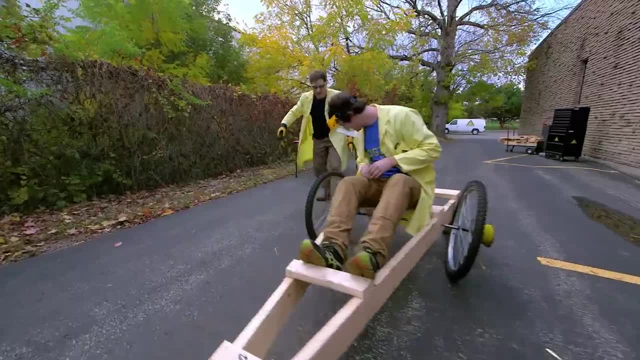 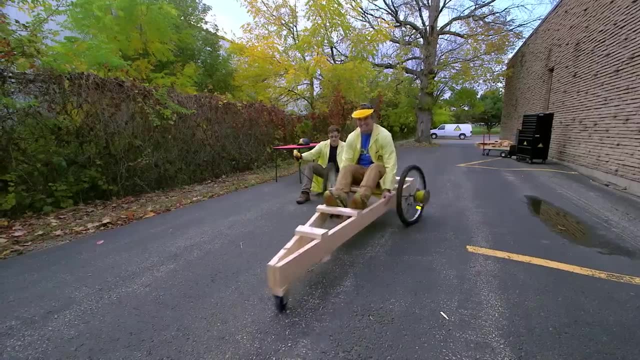 Well, What happened? Ha-ha, Uh, So you went. You went a foot One foot. So what happened? Uh, Uh, So you went. You went a foot One foot. So why didn't that work? uh, nearly as well as the last time we did it. 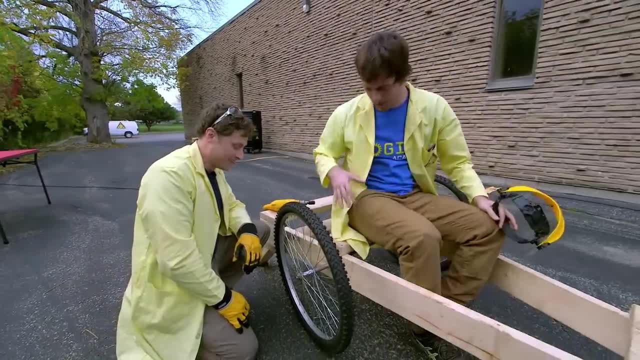 Well, I think my extra weight caused a bit of a problem. Yeah, So the inertia wasn't able to carry us forward, But the whole, The whole point of this is so that someone can ride the dragster. That's Because why? 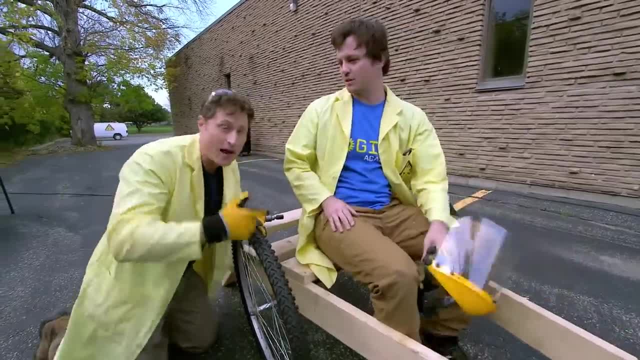 Why build it if we can't ride it? That's exactly right, I think. if we're going to have someone ride it, we need heavier wheels. Well, on the small one, we used plasticine. Yeah To. I don't know if that's what we can. 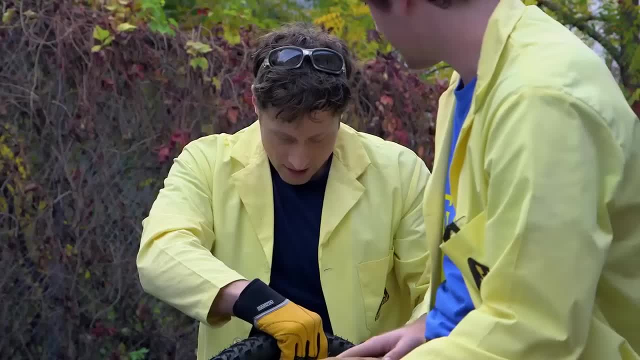 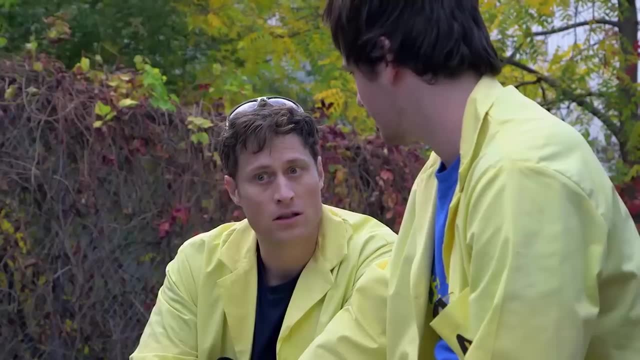 We should use. What if we used Car tires? Car tires, Well, how, What On this? No, I think we're going to have to build something bigger. Yeah, So we. Okay, So we build a whole new frame. 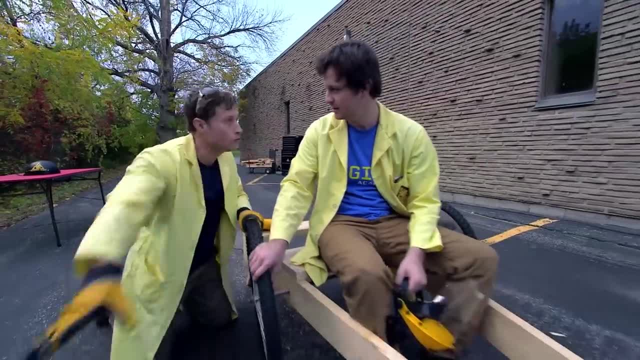 Yep, What if we got like the axle of, Like the back axle of a car or something That's a great idea, The back axle of a car, And then what We use- the drill? I don't think the drill is going to be enough. 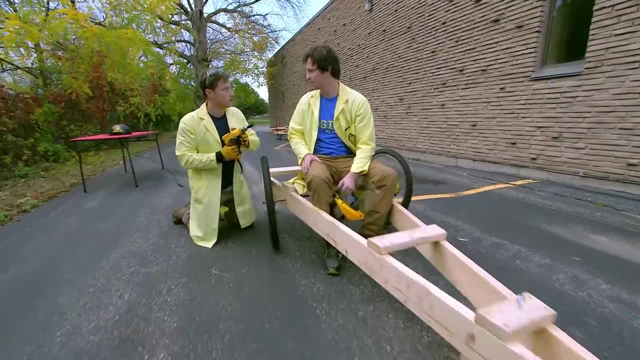 To move the Why? You don't think it's going to be enough to move the back axle of a car? Yeah, It's too Yeah, Too big. So what do we do? Well, what's good at moving the back axle of a car? 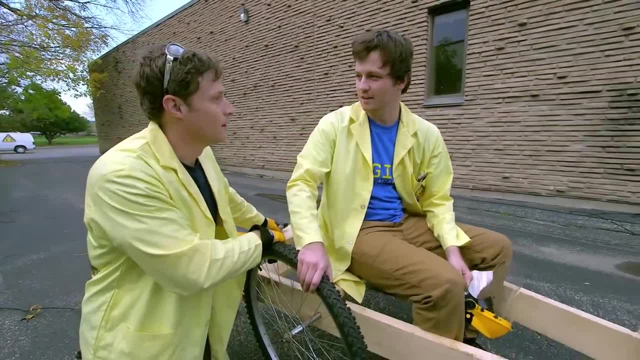 Well, I mean a car, But we would have to take it off the car, so We could use another car. We could use another, We could use. We could use another car, We could use another car. You'll have to explain how that works. 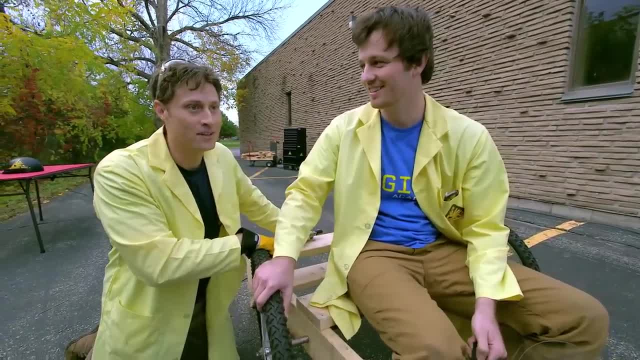 Okay, Let's go. Let's go get the stuff and you can tell me how we're going to use. So how do we use another car to make the first car go? Okay, I'm thinking we jack one car up, Yeah. 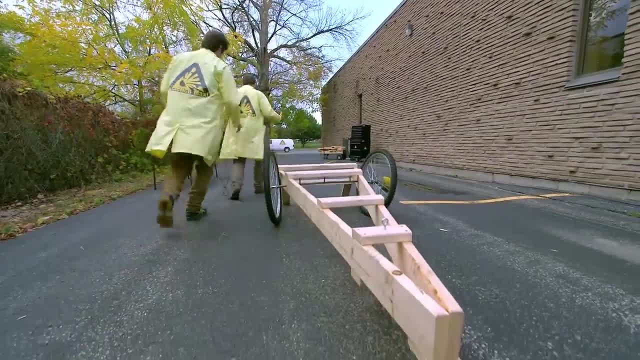 Back our big dragster Newton's Laws in 60 Seconds. Isaac Newton was a super genius, and among the many things he did was come up with three laws of motion that describe how everything works. The first one is the law of motion. 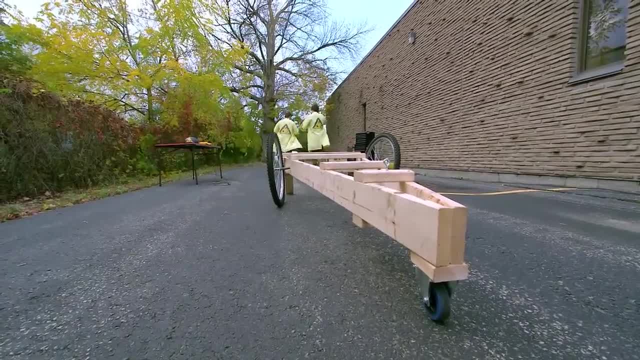 The second one is the law of motion. The third one is the law of motion. The fourth one is the law of motion. The fifth one is the law of motion. The sixth one is the law of motion. The sixth one is the law of motion. 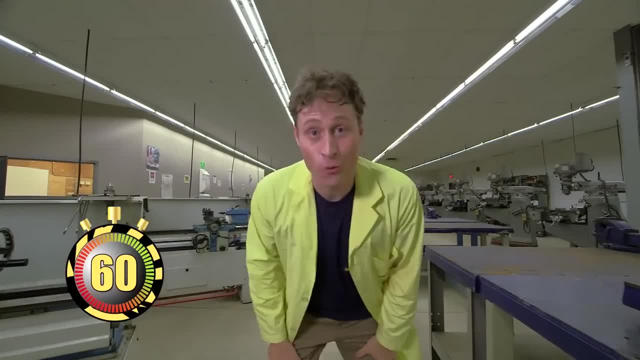 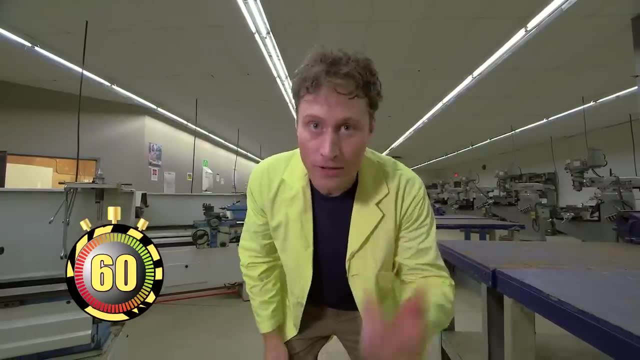 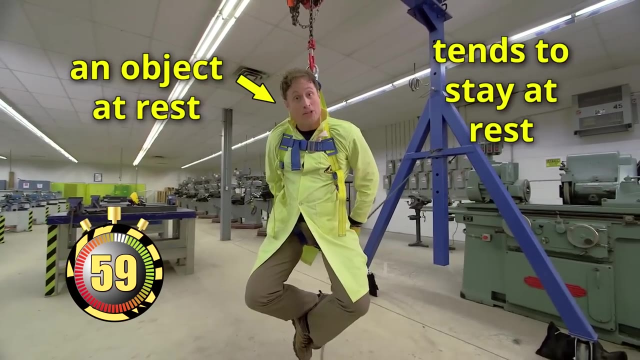 This has been Newton's Laws in 60 Seconds. Isaac Newton was a super genius, and among the many things he did was come up with three laws of motion that describe how everything moves or doesn't move. I will demonstrate using myself Newton's first law: an object at rest tends to stay at rest. 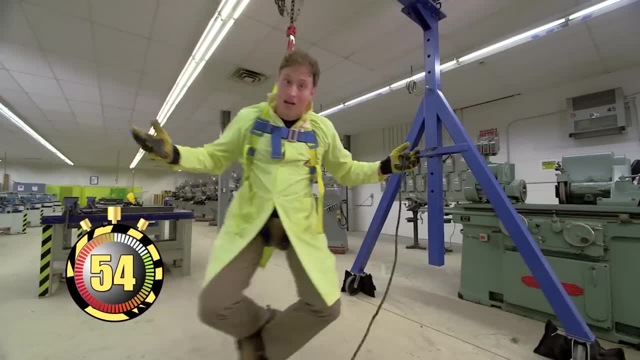 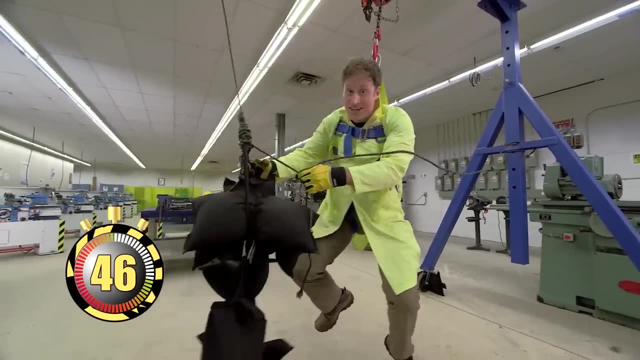 An object in motion tends to stay in motion. Newton's third law is: for every action there is an equal and opposite reaction. These sandbags weigh as much as I do, So when I push them forward, I go backward the same distance. 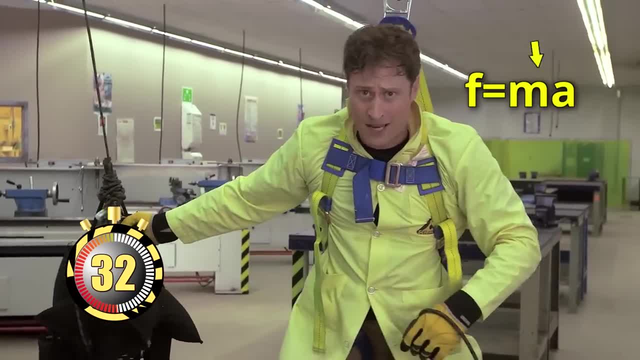 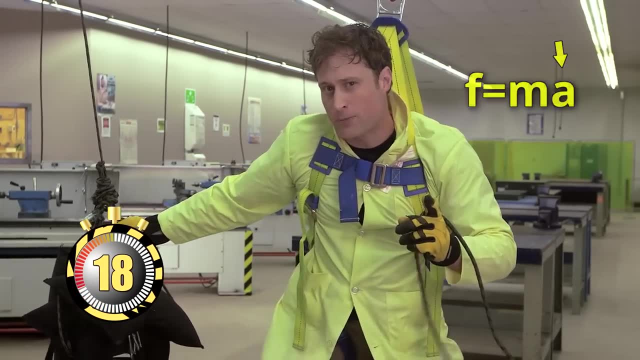 Now Newton's second law is: F equals ma, Force equals mass times. acceleration- How hard you push something is equal to its mass or its weight times its acceleration, or how much you change its speed. I know that one's a little bit more complicated. 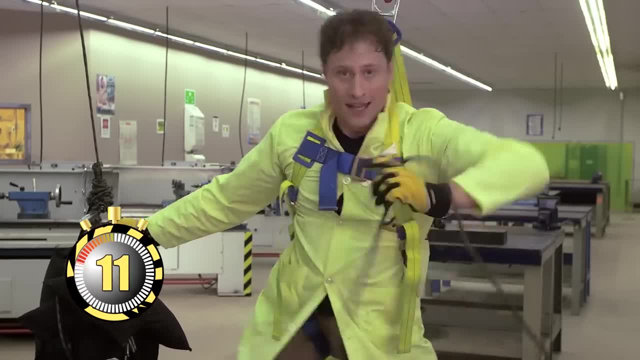 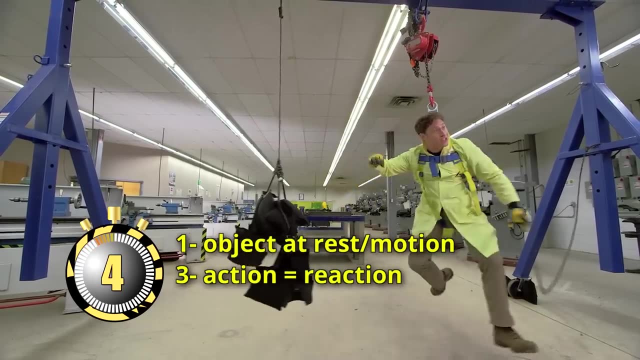 so we're gonna have a whole other segment describing that one coming up Meantime. let's recap. Newton's first law: object at rest tends to stay at rest. Object in motion tends to stay in motion. Newton's third law: for every action. 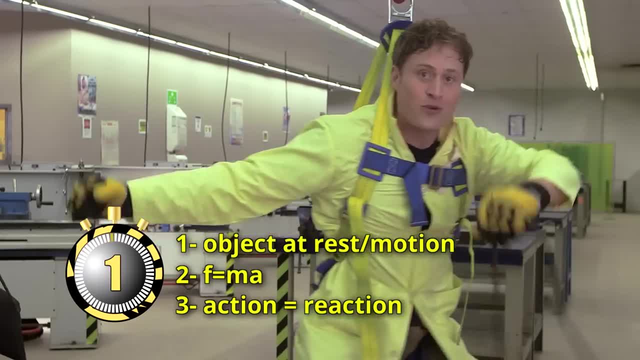 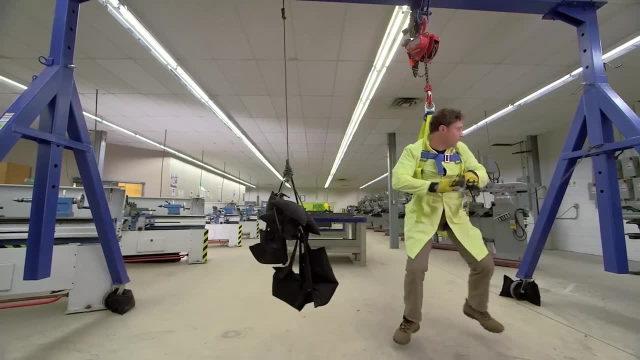 there's an equal and opposite reaction. Newton's second F, ma Newton's three laws of motion. Now, how do I, how do I get down? How do I, how do I get? oh wait, I know, I know. 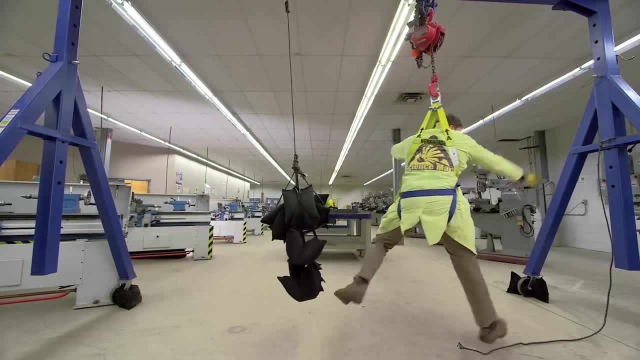 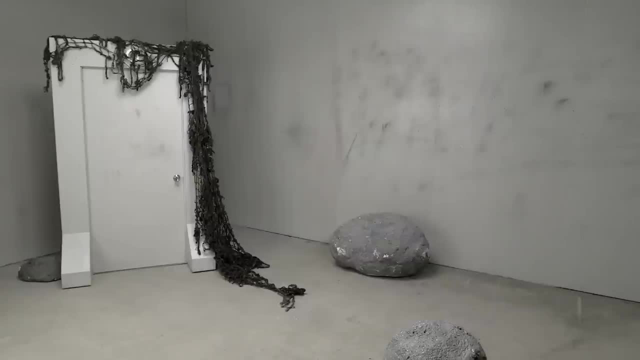 Oh no, that wasn't. that was not a good idea. That was. Now it's time for Science. So Simple a caveman could do it. This is a caveman. This is a door. It is a well, though. 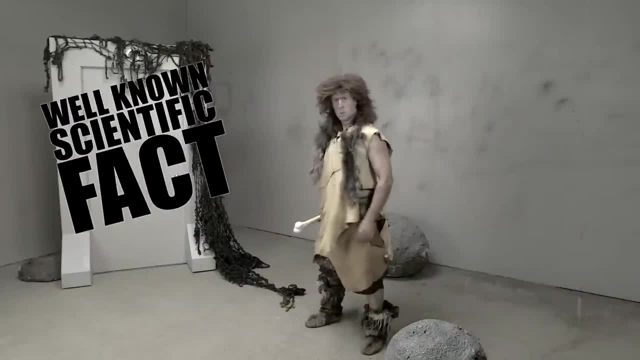 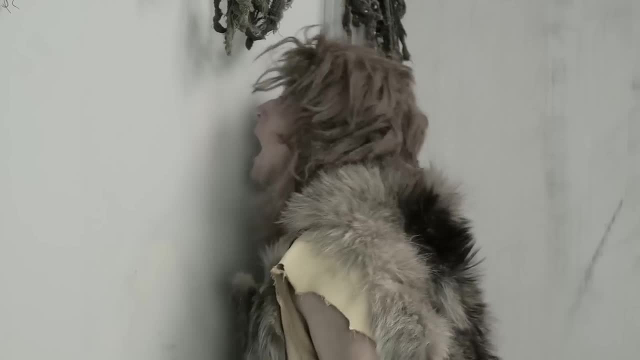 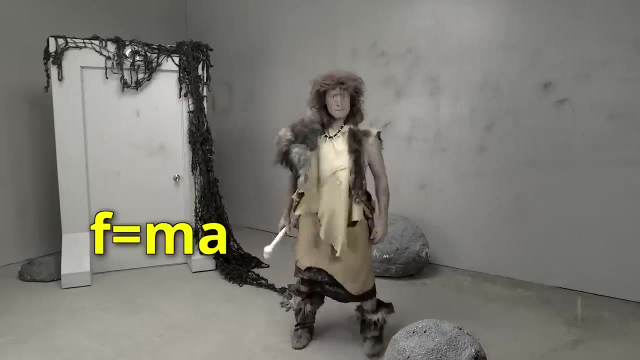 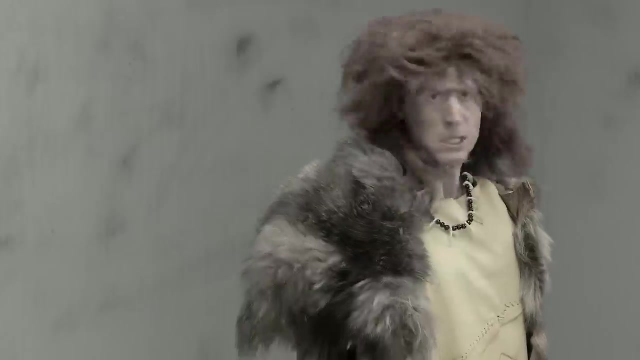 known scientific fact that cavemen do not know how to open doors. Huh, This is Newton's second law: Force equals mass times, acceleration, What Our caveman thinks he can open the door if he uses force, Ah yeah. Well, what if he was to walk, walk, walk, walk, walk, walk. 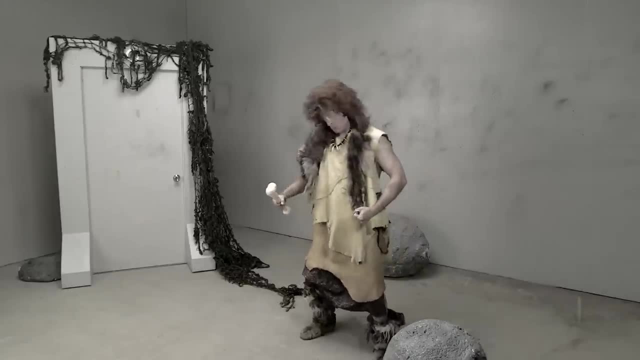 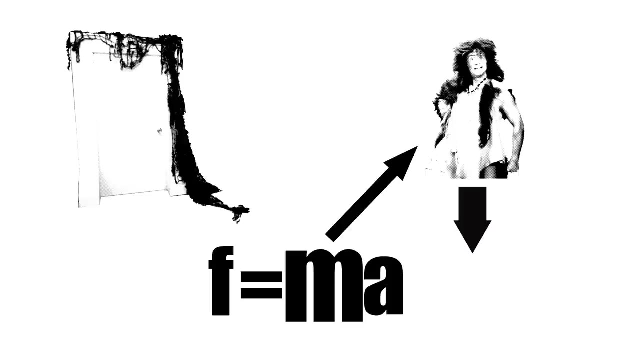 Well, what if he was to walk, walk, walk, walk, walk? Then he will walk briskly into the door. Then the force that he will hit the door with will be equal to his mass, or how much he weighs, times his acceleration. 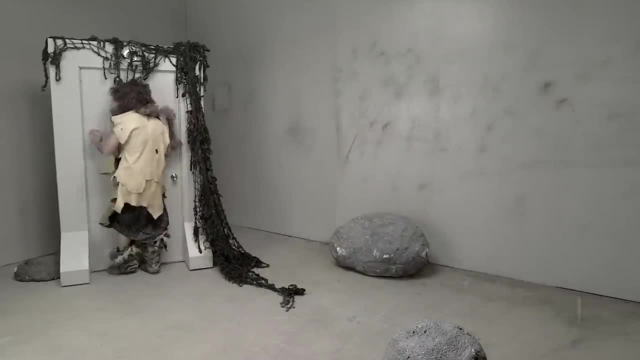 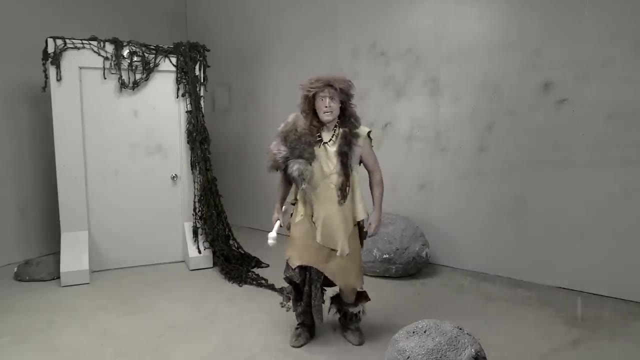 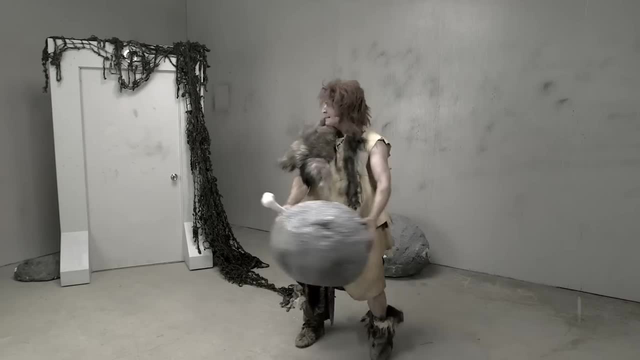 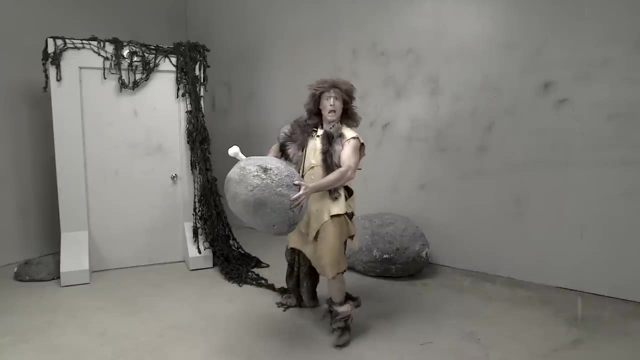 Increase the acceleration, or both. A rock, that's perfect. If the caveman holds the rock, he has a greater mass. Now we just need to increase the acceleration, which means going faster. Let's try running. Go on A little further, that's good. 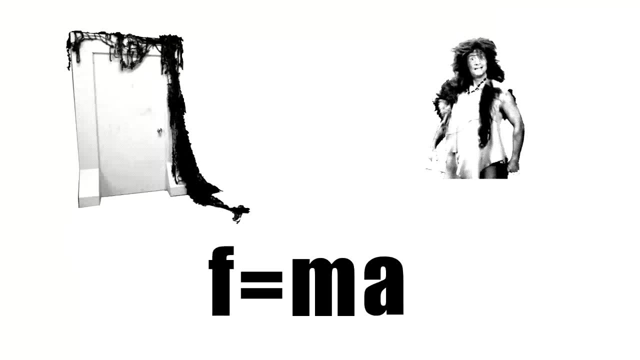 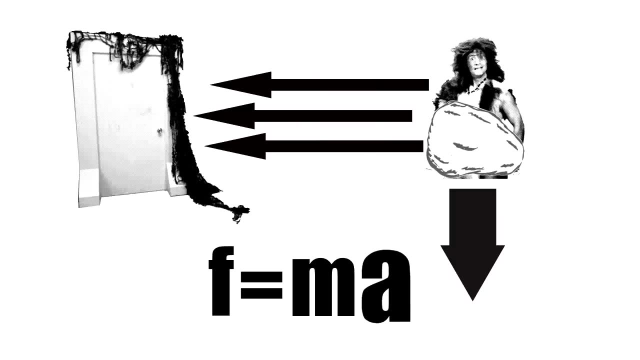 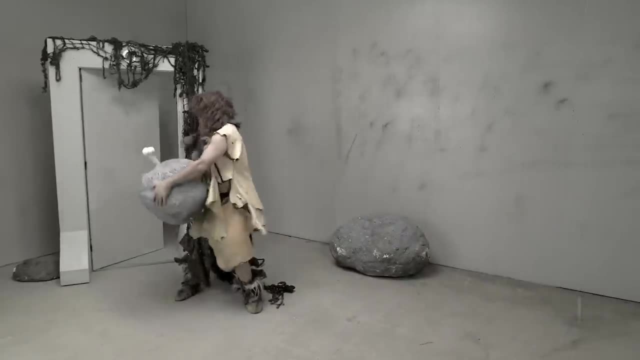 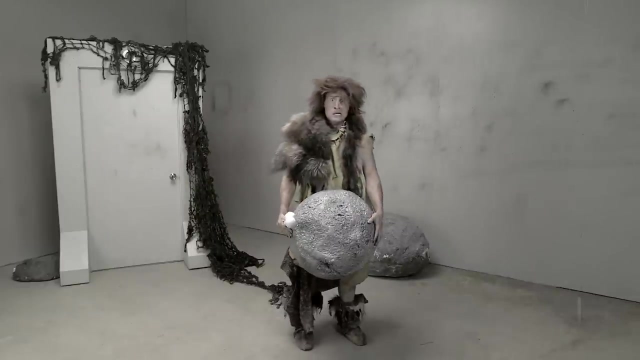 Now the caveman is going to run at the door. To get more force, we've increased the mass to a caveman plus a rock, And we've increased the acceleration to go from running speed to zero. And there you have it. That's how Newton's second law works. 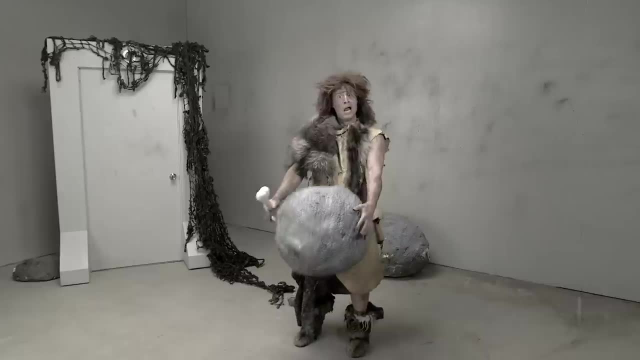 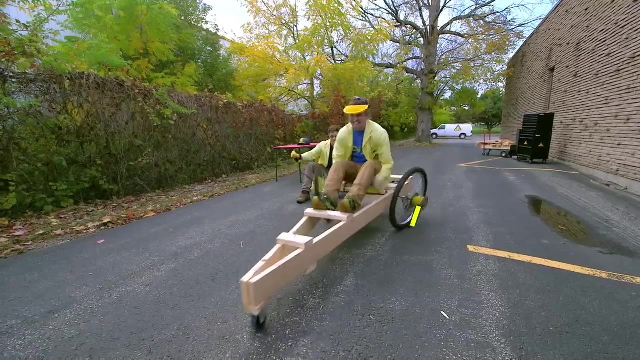 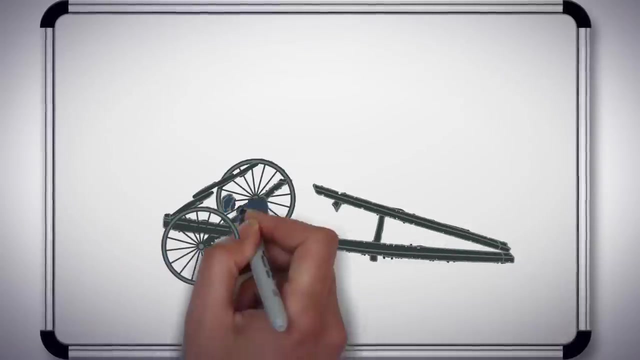 Join us next time for how doorknobs work. What Our inertia-powered dragster just wasn't maxed out enough. So Chris and I built a second dragster, the Dragster Mark II. This one is a welded metal frame. 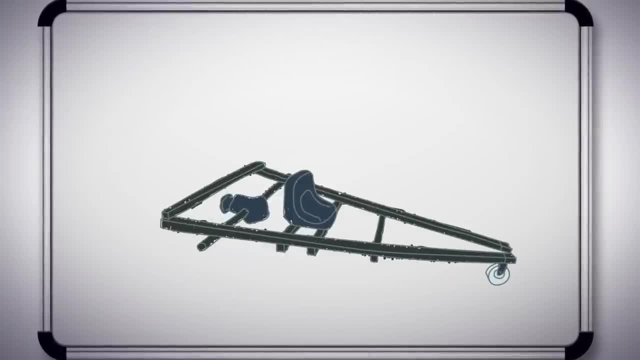 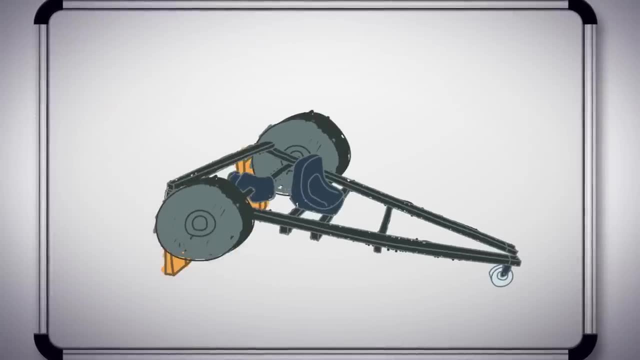 and instead of bike tires we're using car tires, because they're much heavier than bike tires And to get the tires spinning fast enough, we're going to use a car. That's right. we jack up an actual car and have the tires touch each other. 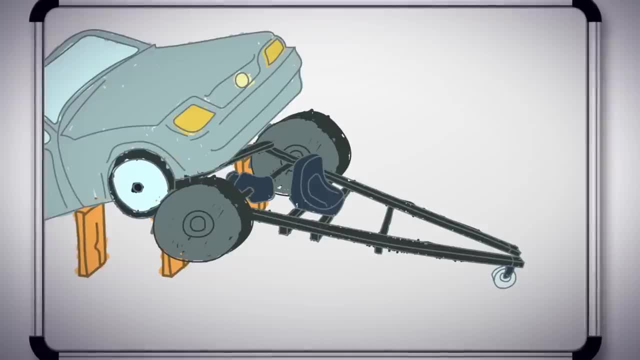 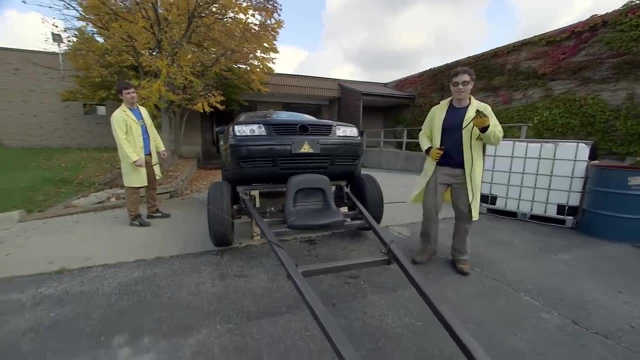 Then we can get those heavy tires to go up and down the track. We're going to get the tires spinning fast enough to get enough inertia to get me going from nothing. The Science Max build team pulled out all the stops on this one, Just like the smaller version. 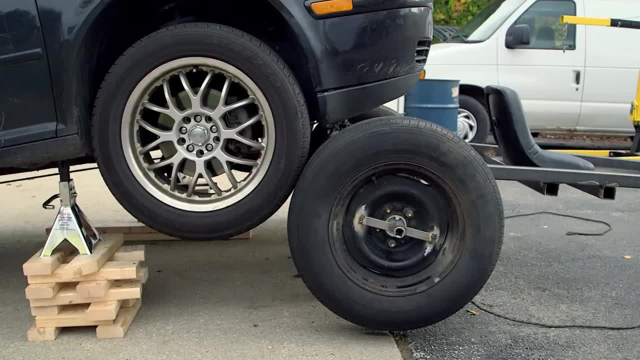 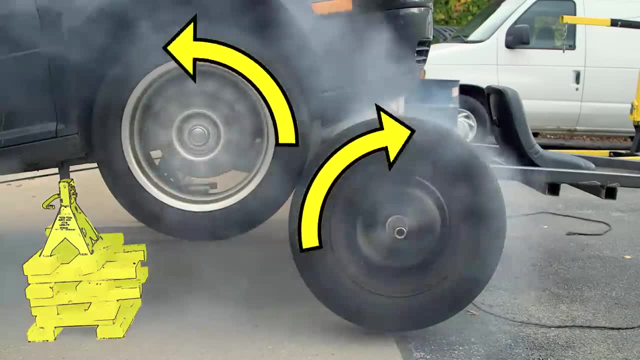 the dragster has to be up on jacks so the wheels don't touch the ground as they get spun up. The wheels of the dragster touch the wheels of this working car, which is also jacked up. That's how we're going to get them spinning fast enough. 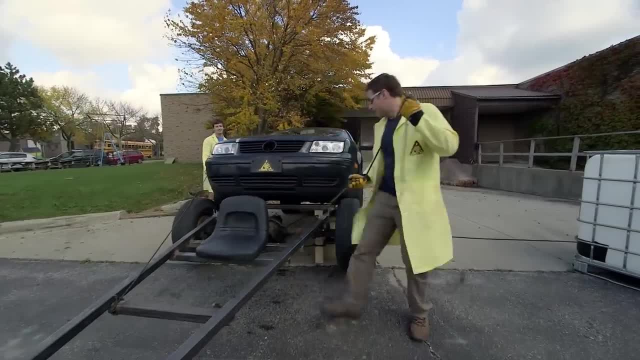 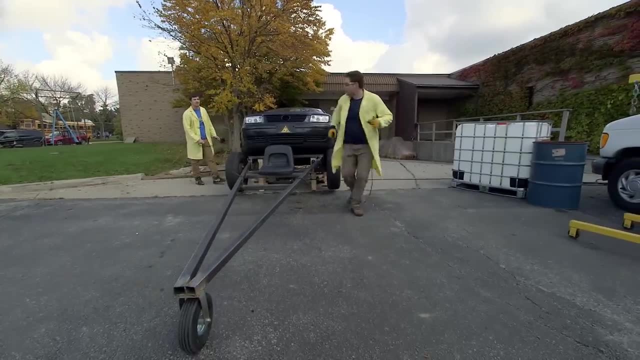 Chris is over there. He's got a rope, just like I'm going to have a rope. When we're ready, we're going to run forward and pull it off the jacks and our dragster will go. We hope right. 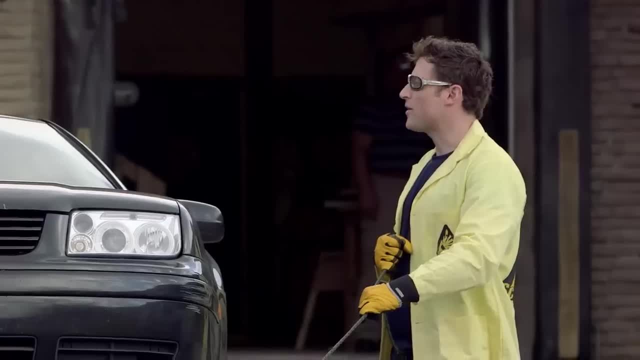 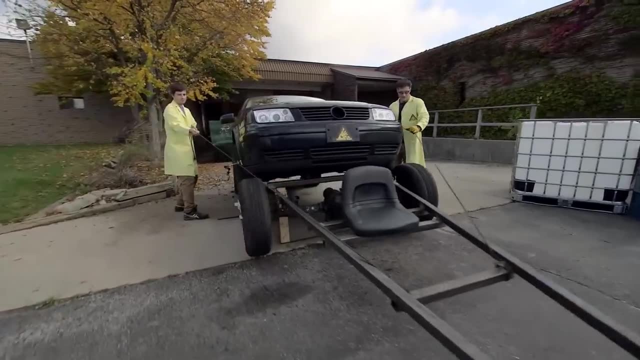 That's the plan, right? I think it's going to work. I think we should do it. Ready, Chris, Ready You ready, Paul Ready, Fire it up, Go, go, go, Faster, faster, faster. 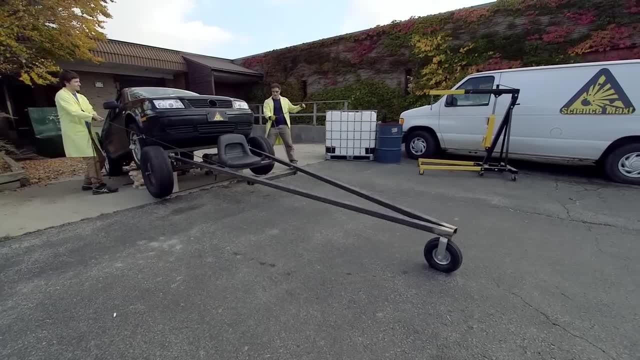 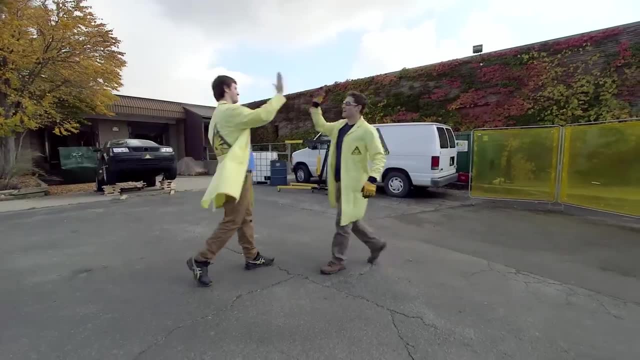 Faster, faster. After three right: One, two, three go. Nice, That's pretty good. Yeah, that worked. All right, I think. are we ready for me to be in it? I think so. All right, we're going to do it. 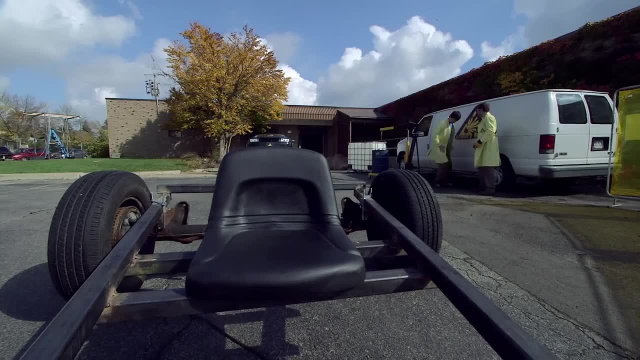 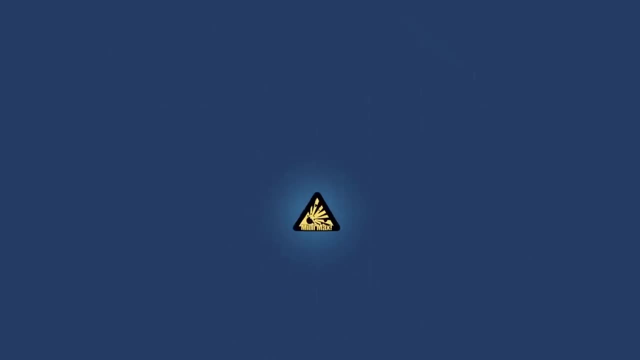 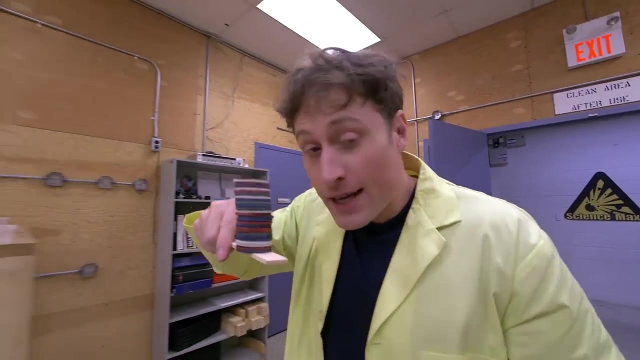 The helmet's in the max van. Do you have the keys for the max van? Keys for the max van? Here's another small experiment you can do with inertia. Take a stack of checkers Or Game pieces like I have here. 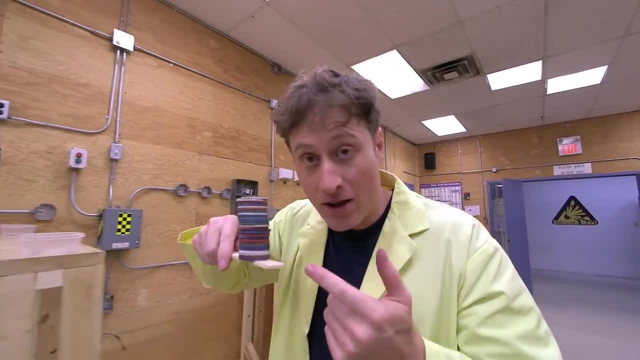 Oh, or coins- Coins work really well- And a ruler or something else that's flat. This is the kind of stick they give you at the hardware store to stir your paint with. Now you can knock checkers out of the middle of the stack. 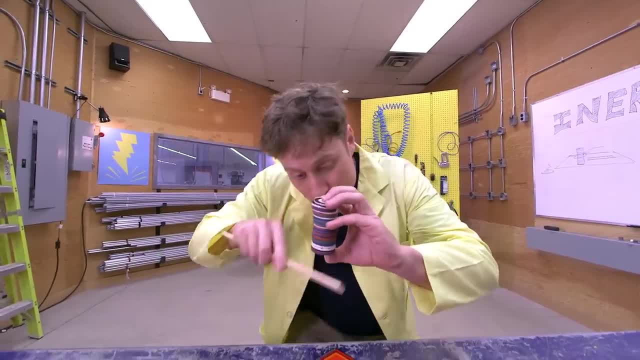 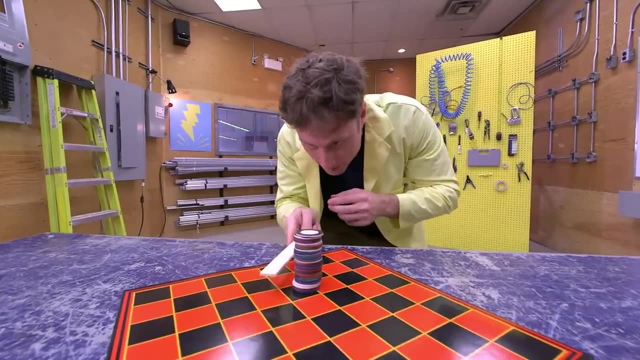 without the stack falling over. if you're very careful, You see the friction of the checkers leaving the middle of the stack won't be enough to overcome the inertia of the rest of the checkers. Ready, Now let's max it out. 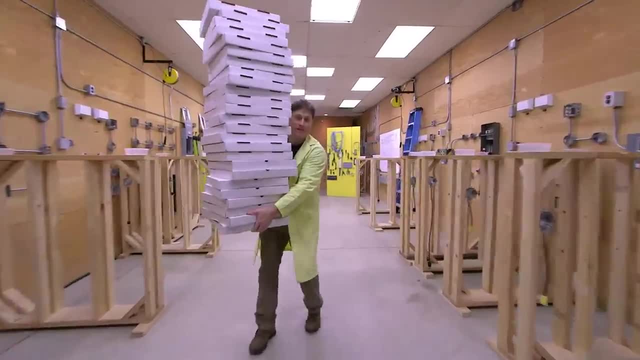 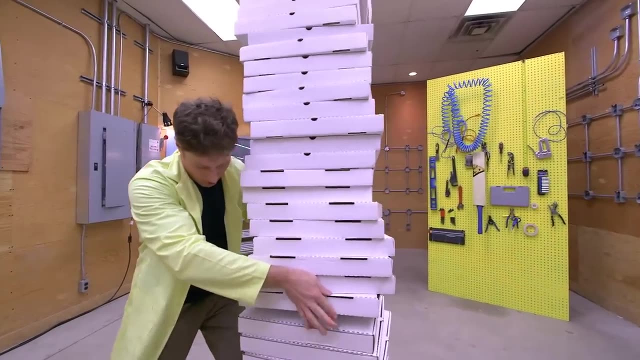 Oh, I have these pizza boxes and they should work the same way. You see, you get a stack And, don't worry, I've already eaten all the pizza And I put them on there like that, And now I need a ruler. 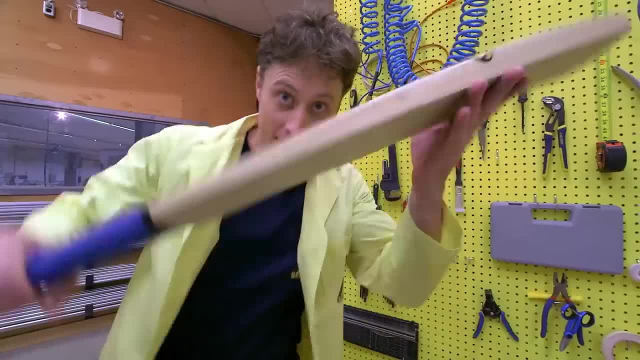 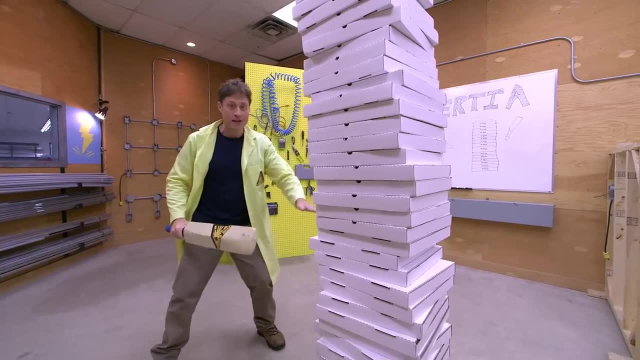 And what I've got is this cricket bat. You see it's got a nice flat edge, just like the ruler. Now, if this works right, I can hit it hard enough to knock out just one or two pizza boxes, and the rest of the stack should stay. 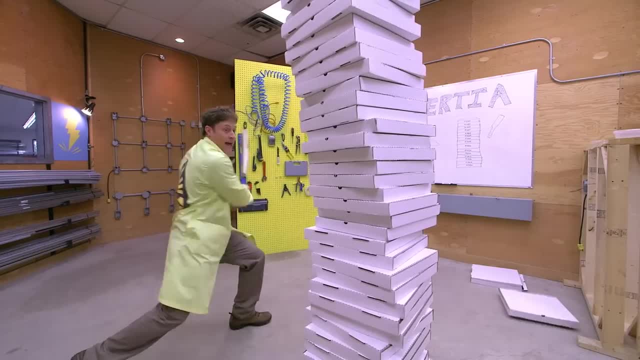 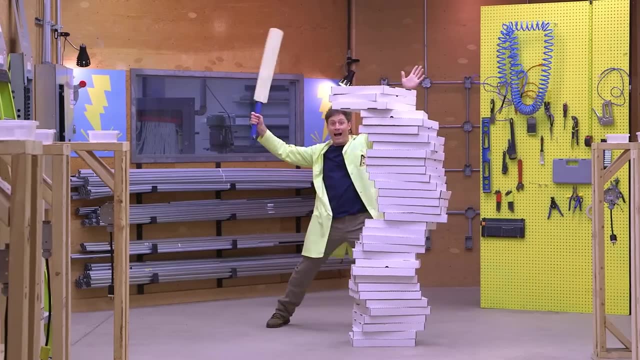 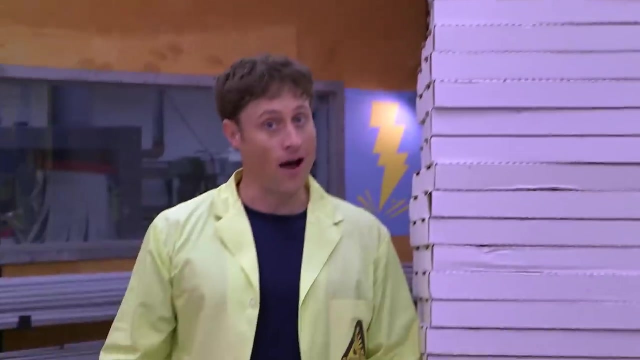 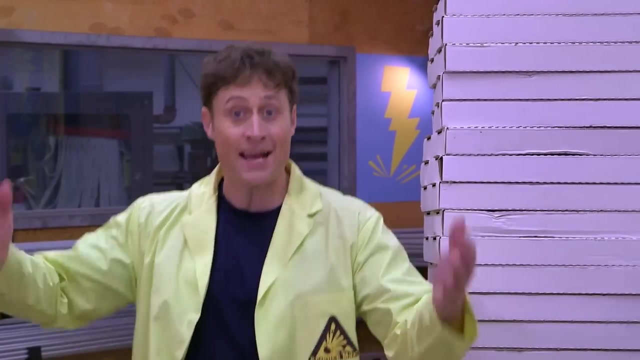 Here we go, Ready Go, Science, Awesome. And there you have it, Newton's first law: An object at rest tends to stay at rest And an object in motion tends to stay in motion. An object in motion tends to stay in motion. 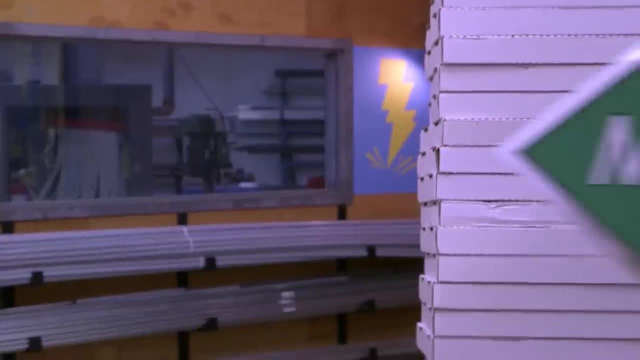 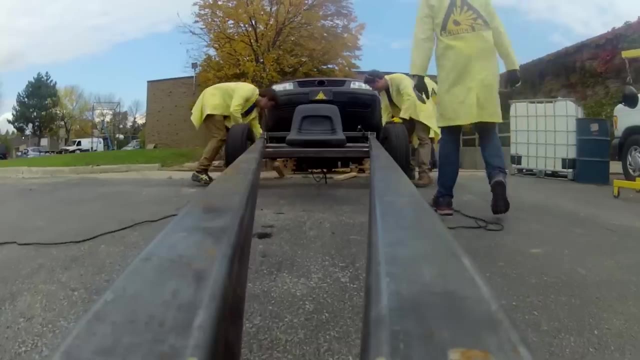 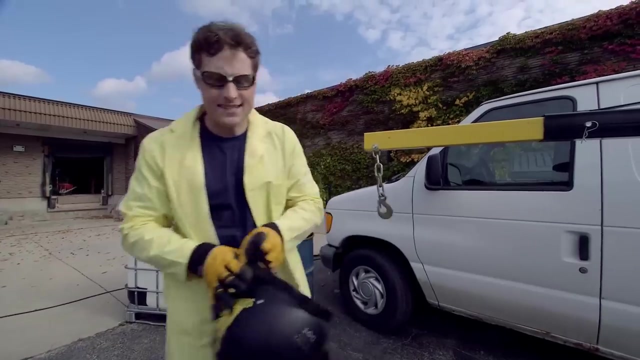 Usually there's a sign that kind of: Well, our inertia-powered dragster worked really well And now it's time for the final step: me riding it to glory. Now I know it probably doesn't need saying: but don't try this at home. 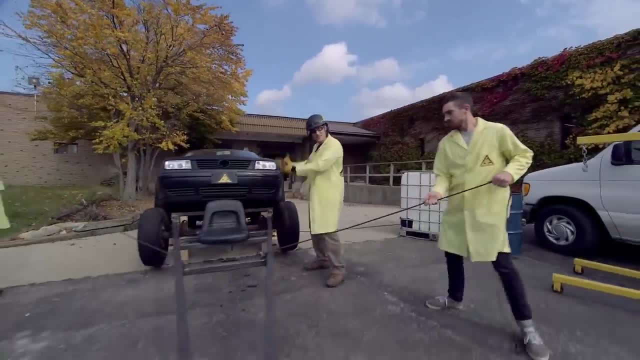 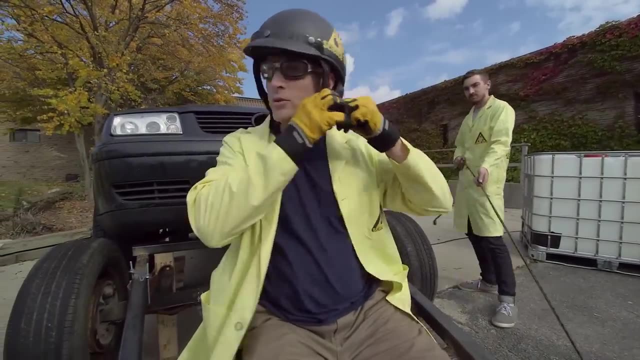 Not that I think you really can try this at home, because this is kind of involved, But I figured I should probably tell you guys, just in case you were tempted to try it at home. We know what we're doing. We know what we're doing, right, Chris? 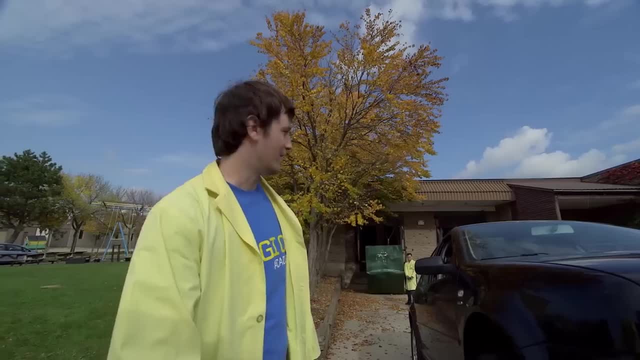 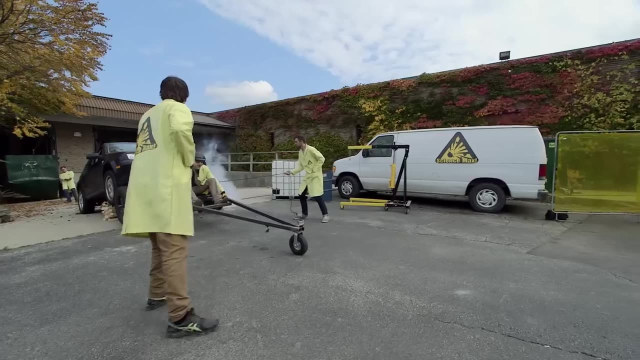 Yes, Yes, Yes, We know what we're doing. All right, Fire it up, Keep it going. Keep it going All the way, Whoa, All the way. Three, two, one, Go, Woo Yeah. 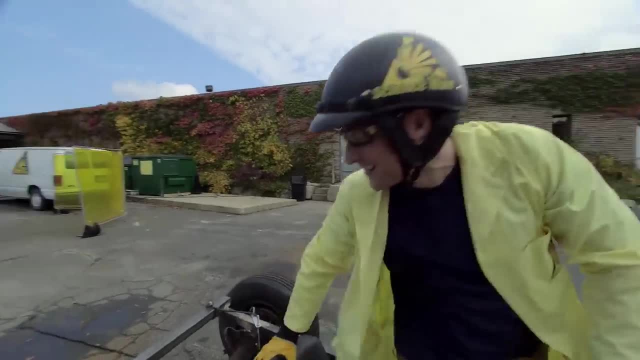 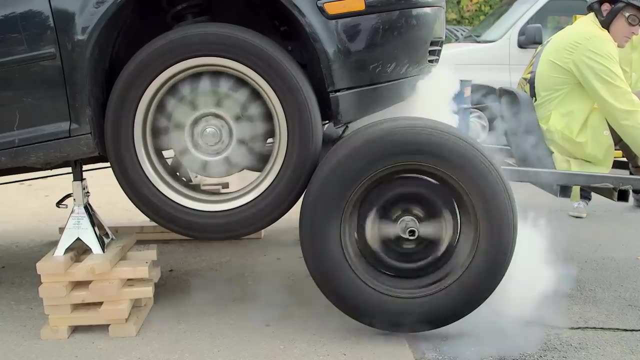 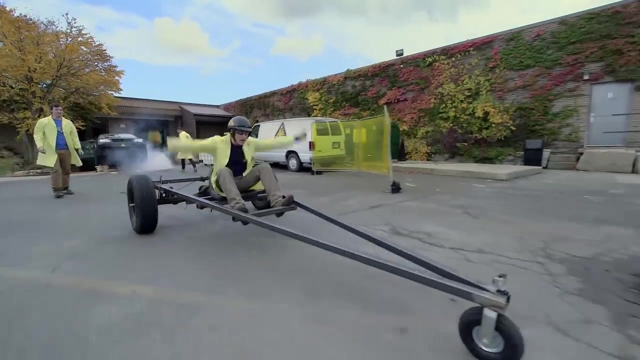 Yeah, Woo, How's that for inertia? Wow, Look at that, That's amazing, Cool High fives. Yeah, Let's recap The weight of the tires as well as how fast they were going, provided enough inertia to accelerate me- and the weight of the dragster. 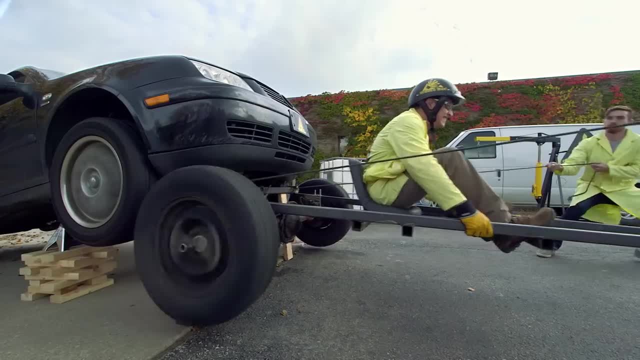 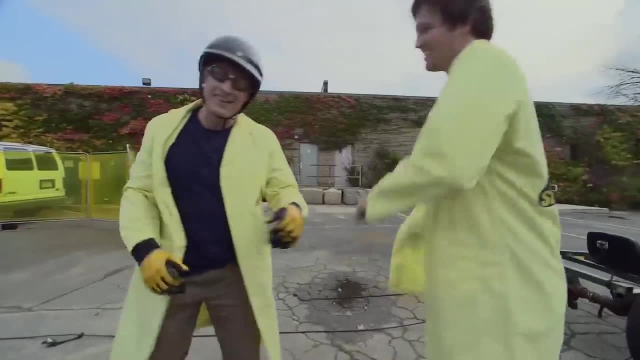 The objects in motion. the wheels wanted to stay in motion, so much they moved the dragster all by themselves: Inertia and Newton's first law of motion. Thank you for joining us on Science, Max. Let's go again, Your turn. 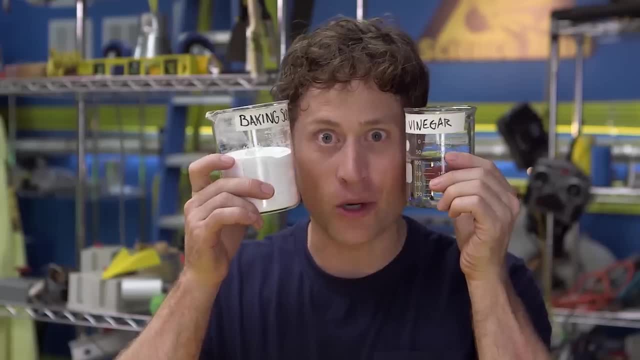 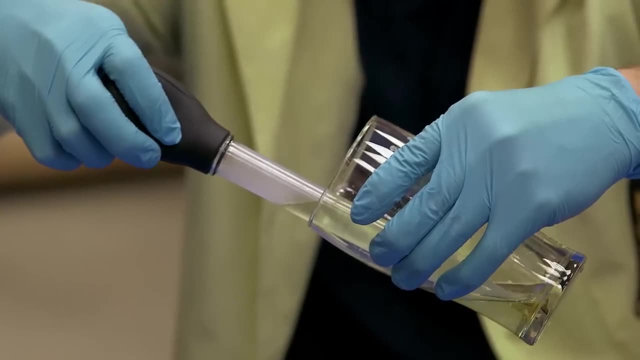 Yeah, my turn. Okay Woo. Today on Science Max, we're looking at Chemicals, Chemicals. Chemicals make up everything around us and we're finding out which ones you can mix together to make spectacular science. Whoa. 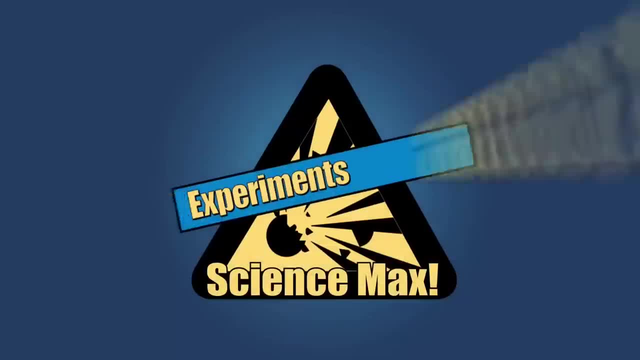 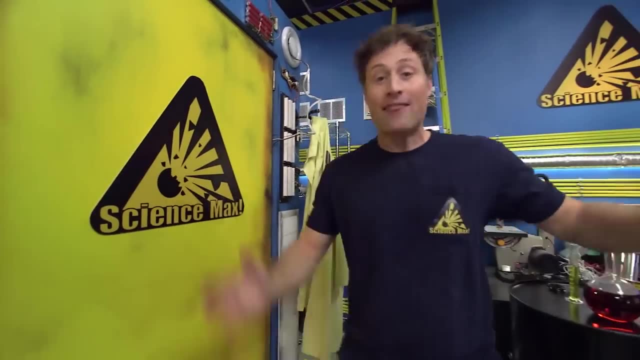 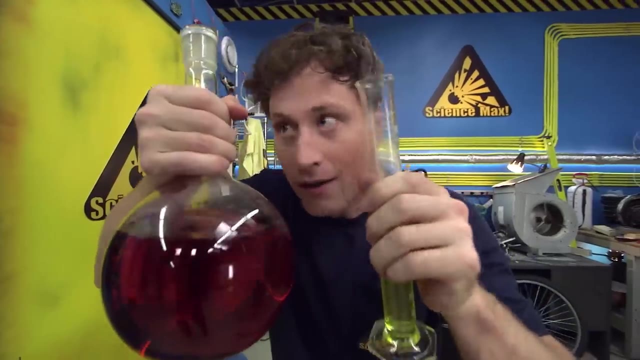 Woo, Cutest science ever Today on Science Max Experiments at Large. Greetings Science Maximites. My name is Phil McCordick and the name of the show is Science Max- Experiments at Large. Today we're taking a closer look at chemistry. 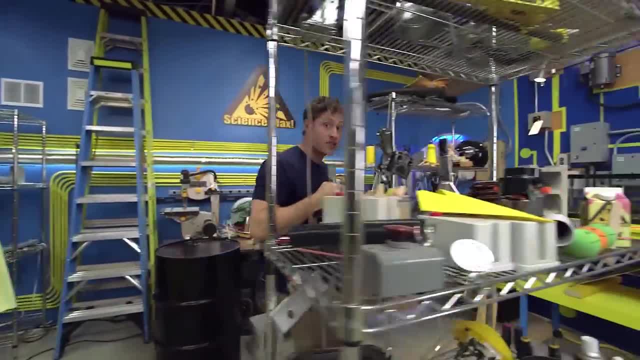 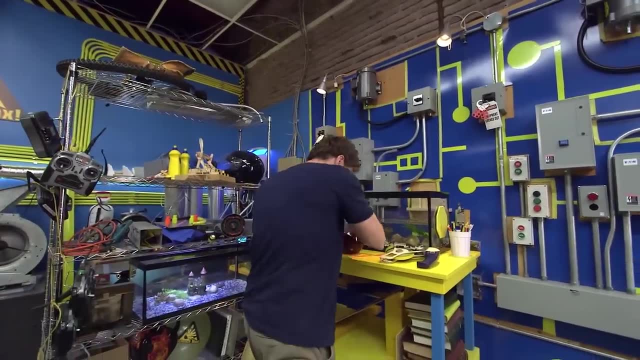 Ooh, Chemistry is the science of atoms and molecules, the things that make up all matter, and how they interact with each other. Take, for example, this glow stick. Actually, don't take it, because I kind of need it. 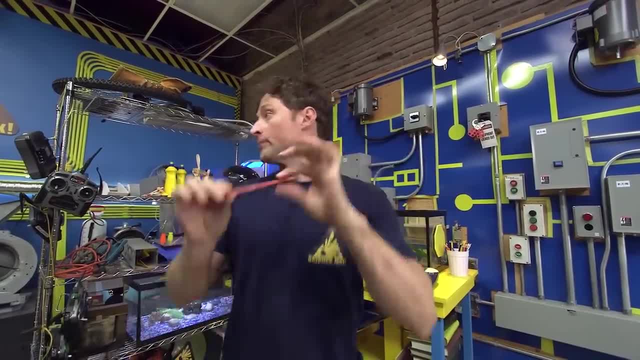 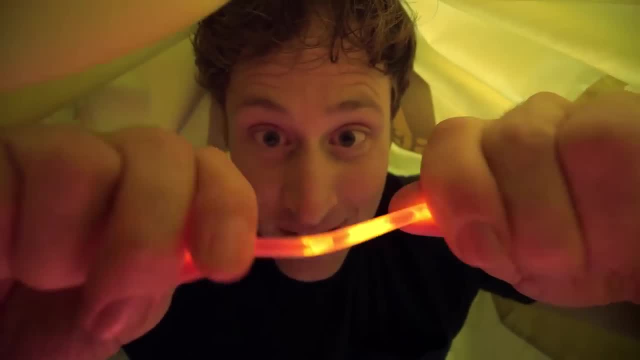 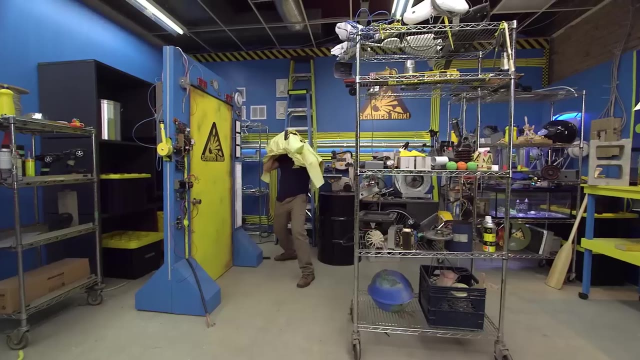 The glow stick doesn't glow until you- Um, The glow stick doesn't glow until you break the barrier and mix the two chemicals and they start to glow. Huh, Pretty cool, huh? Chemistry Now the chemical reaction we're looking at today. 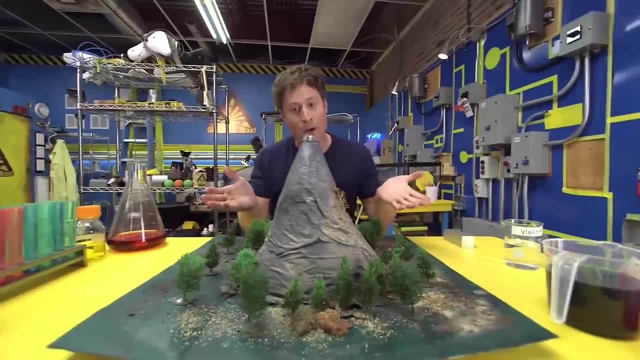 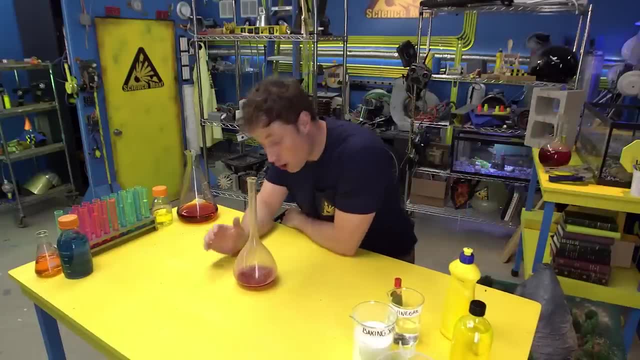 is the old vinegar and baking soda volcano, But this reaction doesn't have anything to do with volcanoes, It's chemistry. Now, this experiment is totally safe, but I do recommend you get an adult's permission before you do it, because it's very messy. 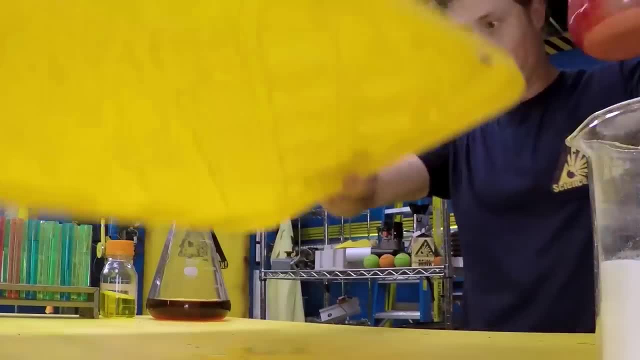 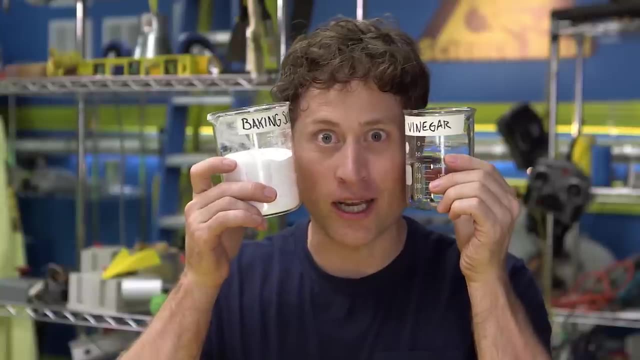 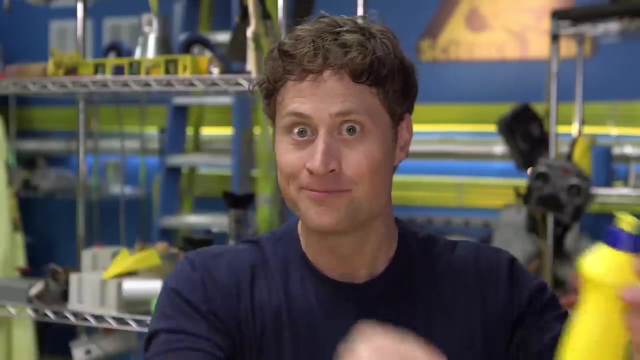 Uh, Uh Yeah. First you're gonna want baking soda and vinegar. These are your two main ingredients, But you'll also want dish soap and red food coloring if you want it to look a little bit more like lava. Now I like to mix the baking soda. 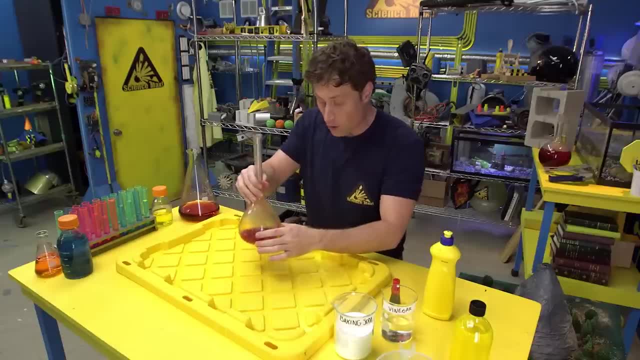 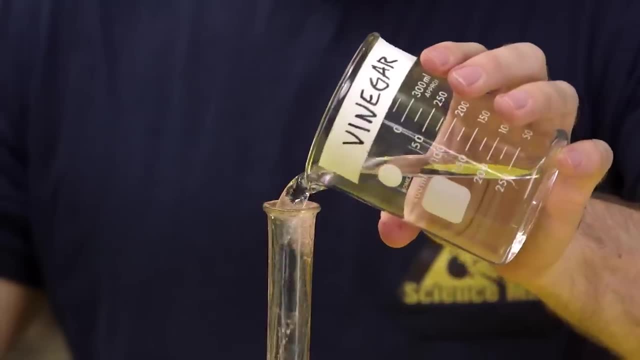 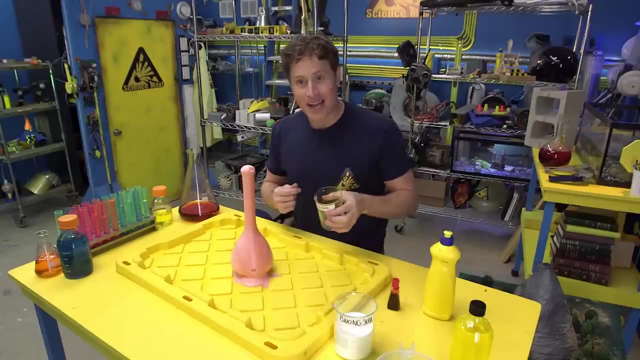 red food coloring and dish soap, together with a little warm water. so all you have to do is add the vinegar, And when you do this is what happens, And there you go- Chemical reaction. Now I know what you're thinking. 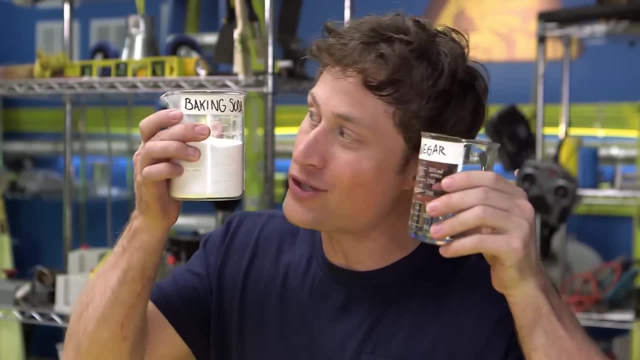 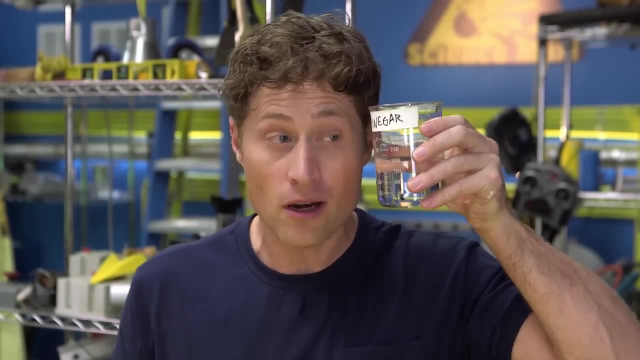 You're thinking, Phil, how much vinegar or baking soda do I use? Well, I'm not gonna tell you. This is where you can be Science Maximites. Try different amounts: More vinegar, more baking soda, More dish soap. 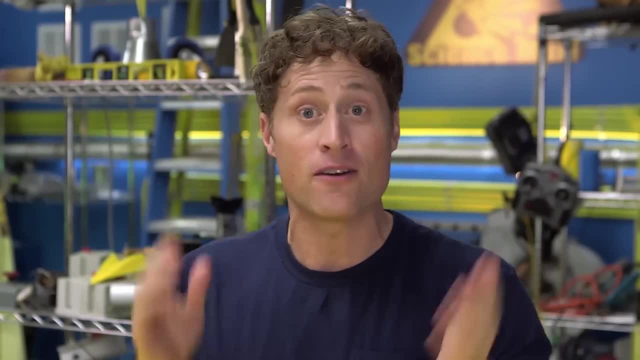 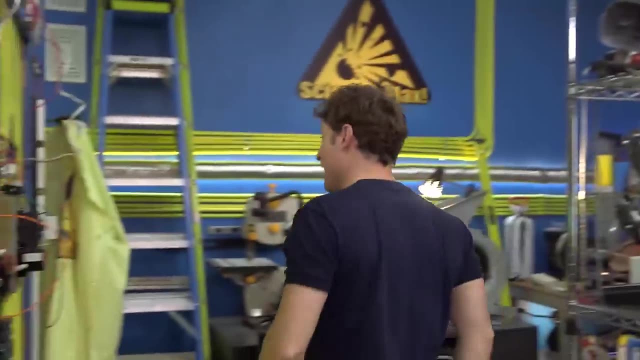 Who knows? Write down the amounts each time you use it and find out what amounts work best. That's called science And that's what we're gonna be looking at today: Chemistry in all its forms And, of course, because it is Science, Max. 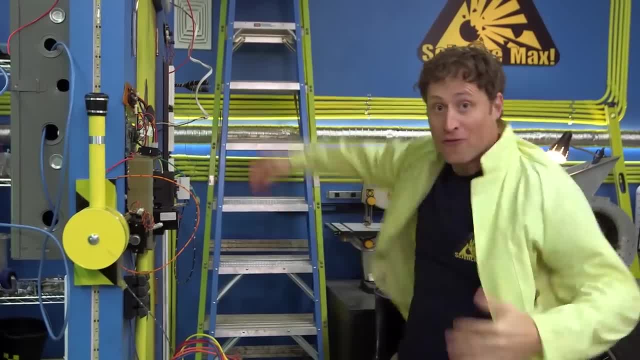 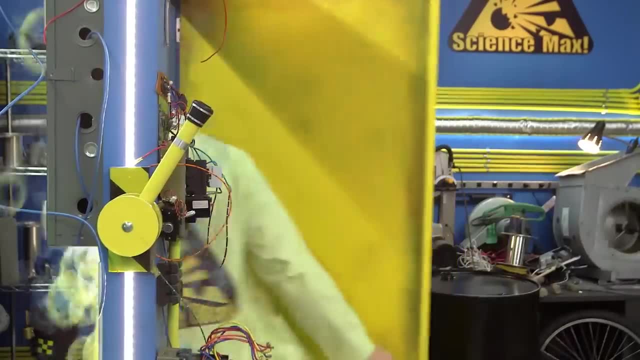 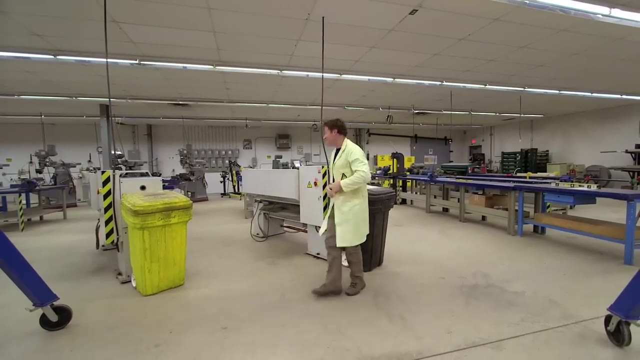 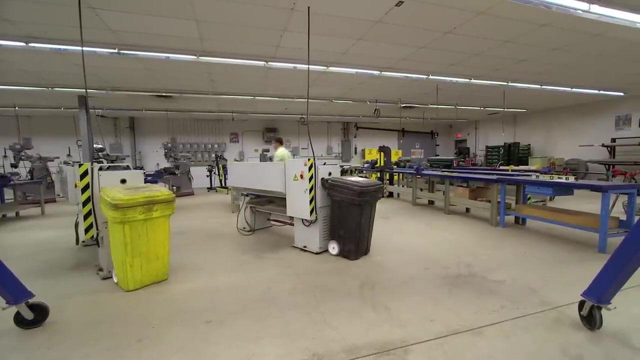 experiments at large. we're going to max out the vinegar and baking soda volcano. So I'm off to the Center for Skills Development and Training. Come on, Hey Talena, Hi Phil, How you doing Good? This is Talena. 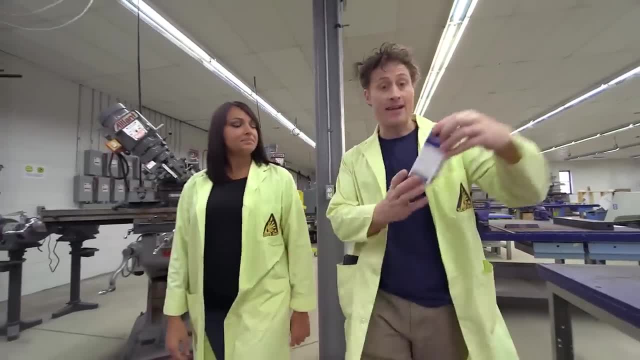 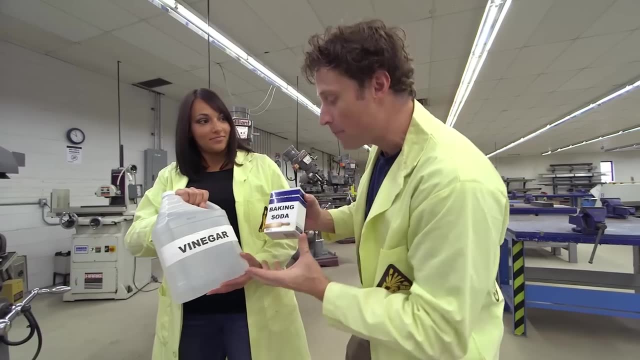 She's going for her PhD in chemistry from McMaster, right, Yep, Awesome. Which means you can help me max out the baking soda and vinegar. You grab that vinegar And vinegar volcano. So what happens when we mix these two chemicals? Well, vinegar is an acid and baking soda is a base. 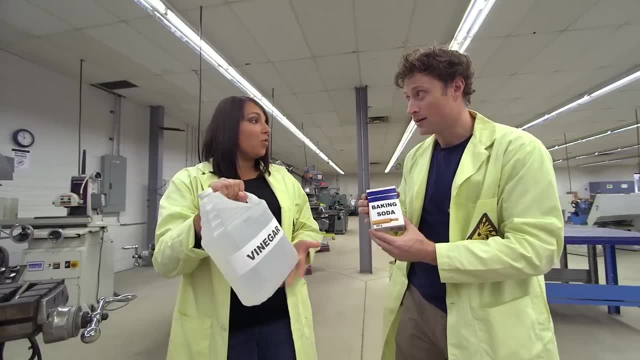 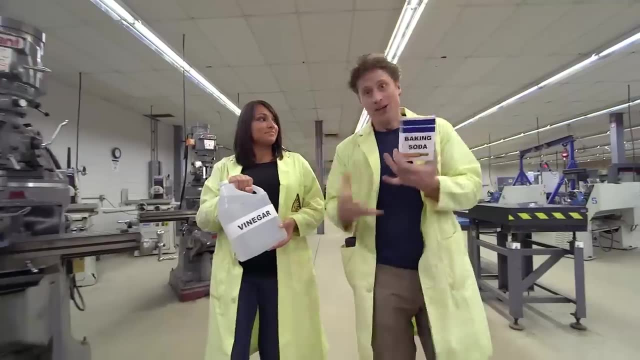 And when you mix them they neutralize each other to produce carbon dioxide and water as a byproduct. Hmm, So acids and bases are kind of like opposites, Yep, So I guess that makes sense. When you put them together, crazy stuff happens. 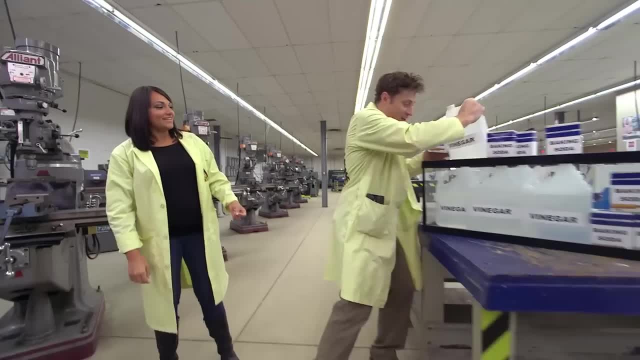 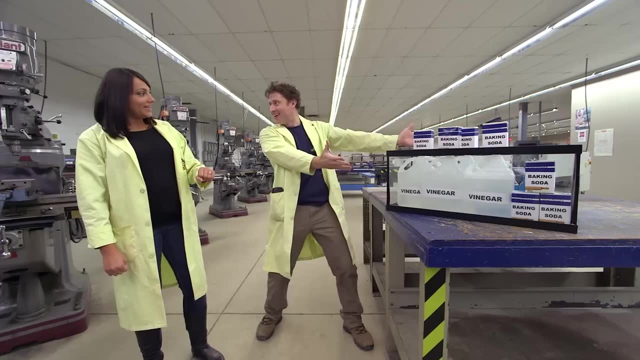 Yeah, I agree. Okay, so I want to use this much vinegar and this much baking soda. What's with the fish tank? The fish tank is where I want to mix it all together. What do you think? Awesome Maxed out. 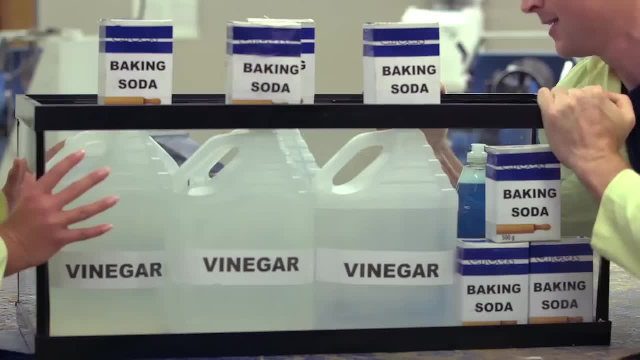 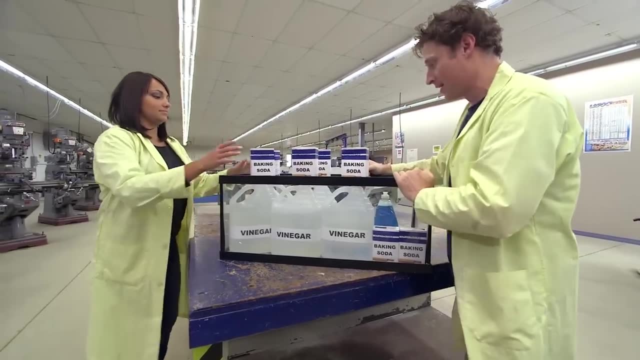 Okay, Let's move the fish tank somewhere where we won't make a huge mess. It's a little heavy with all that, Are we going to? No, we're going to have to take a couple trips. That's kind of heavy. 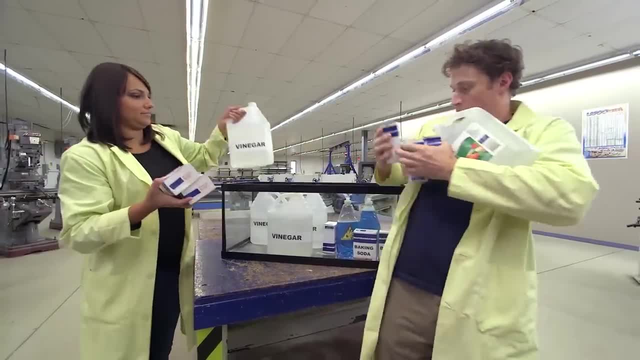 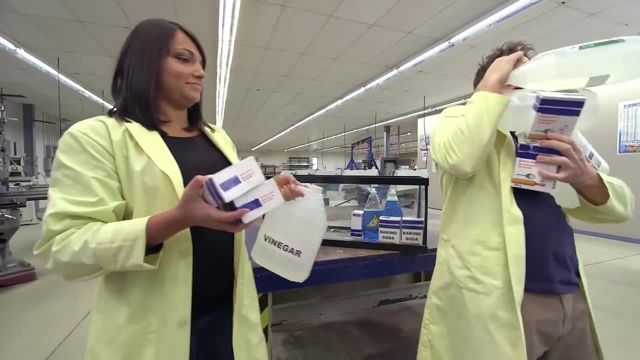 Okay, so we'll take this and that and then this and that. No, hold on One more. Okay, good, Okay, good. Yeah, I took too much. I took too much, Uh-oh, Uh-oh. 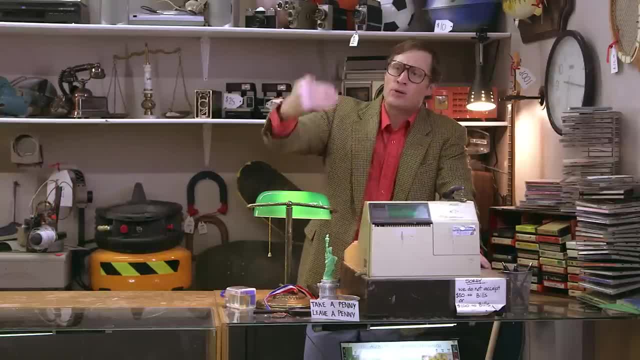 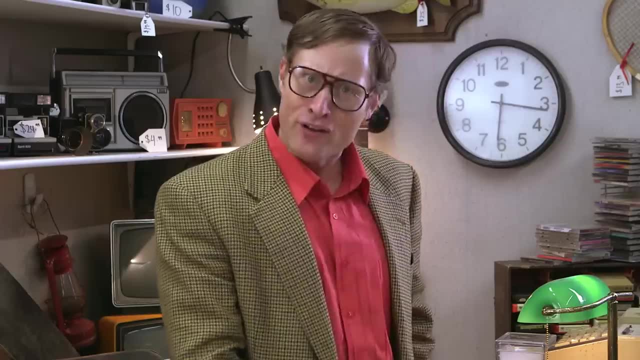 That's good, Ramona. Put it in the background. Put the sign in the background. Yeah, in the BG. I love the BG. Chemicals, Chemicals, Chemicals, Chemicals, Chemicals. What are chemicals? Are they things you have in a lab, in a jar? 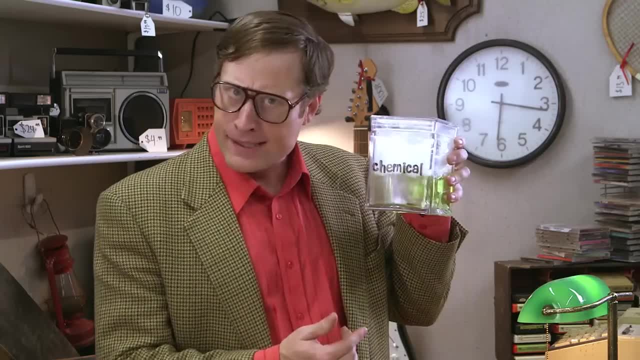 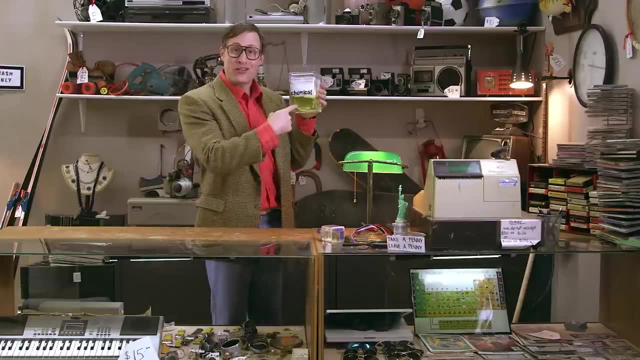 that say chemical on them. Well, yes, but if that's all you think chemicals are, then you need to know your chemicals. Turns out the stuff in the jar is a chemical, but the jar itself also made of chemicals. The table I'm putting it on made of chemicals. 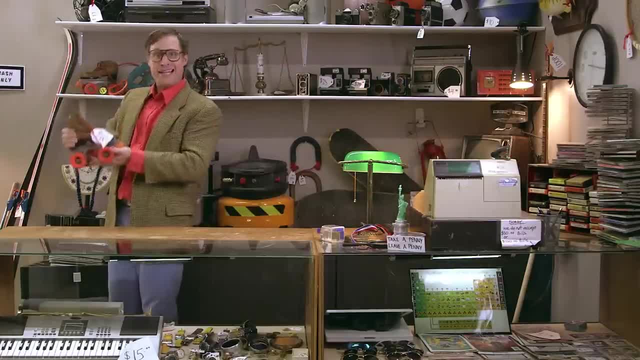 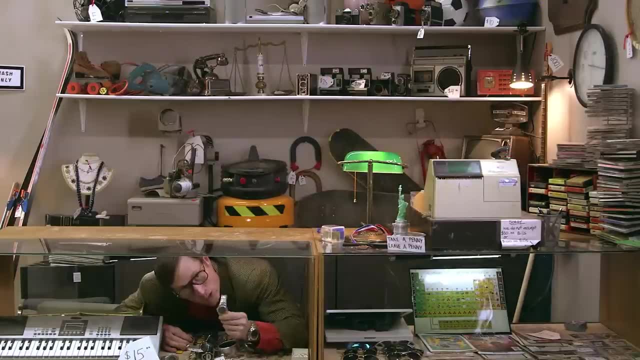 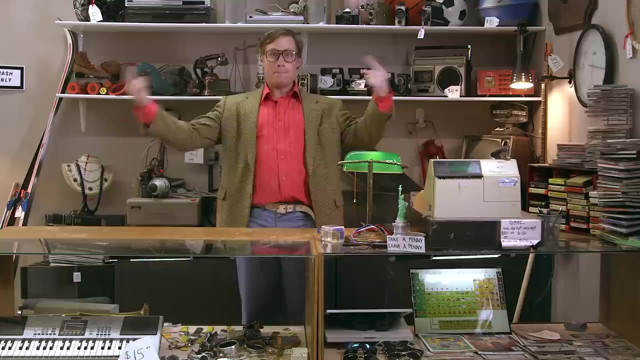 My lunch chemicals. Roller skate chemicals. My jacket chemicals. This guitar chemicals. My shoe chemicals. This watch chemicals. This fish chemicals. Chemicals, Chemicals, Chemicals, Chemicals, Chemicals, Chemicals. 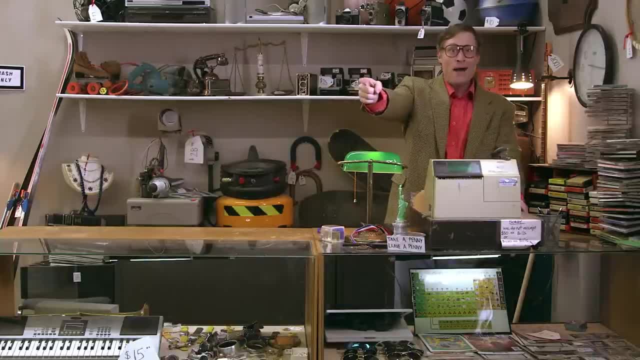 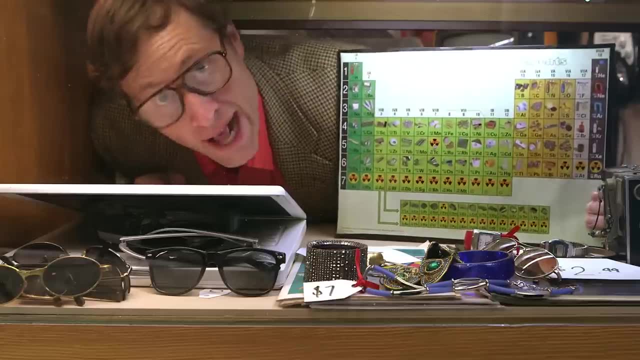 Me chemicals, You chemicals, Ramona chemicals. No, I said you're chemicals. Come on, never mind. This is it the periodic table of the elements. All matter in the universe is made up of these pure elements. 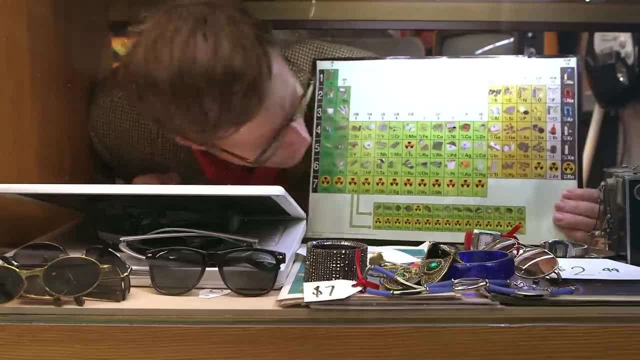 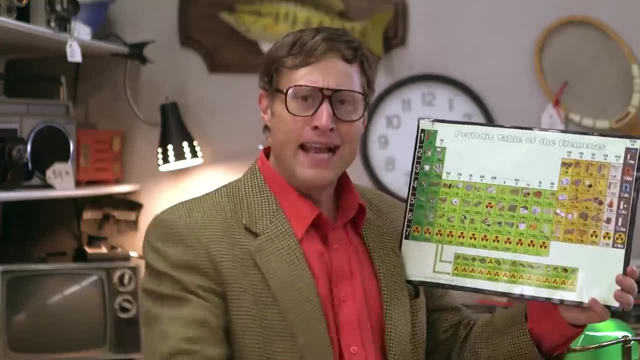 They go together in different ways to make up everything, All matter. Think of it like the name of a vegetable, Think of it like a plant, Think of it like building blocks. These little atoms are some of the elements on this periodic table. 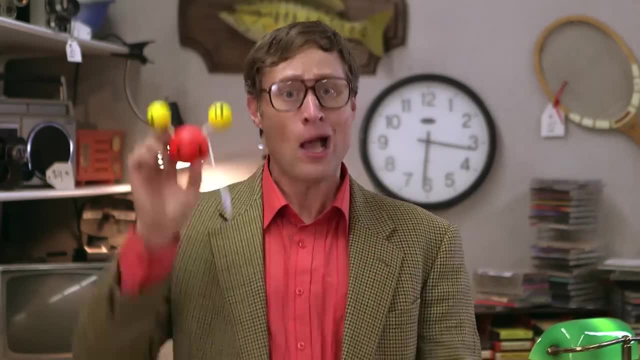 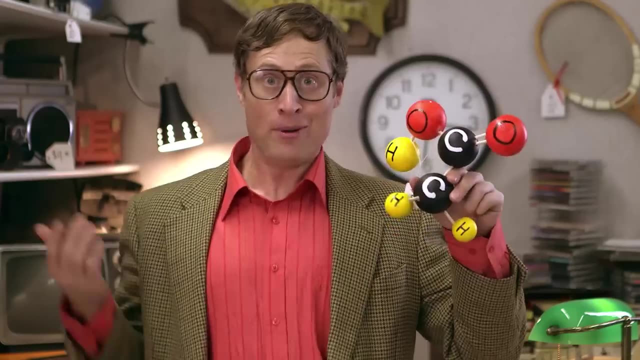 You got one oxygen, two hydrogen. Bam, You got a water molecule. One carbon, two oxygen. Hey, it's carbon dioxide. Two carbon, two oxygen, four hydrogen Skadoosh Vinegar. One sodium, one chlorine. 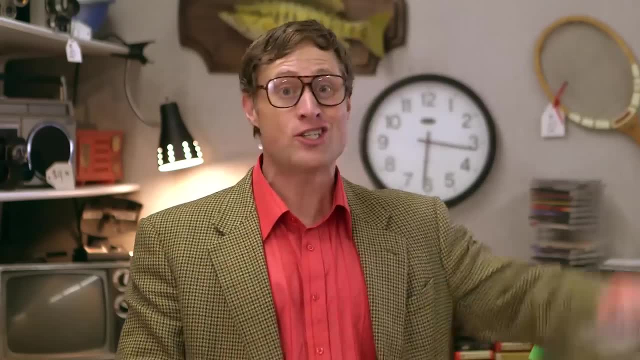 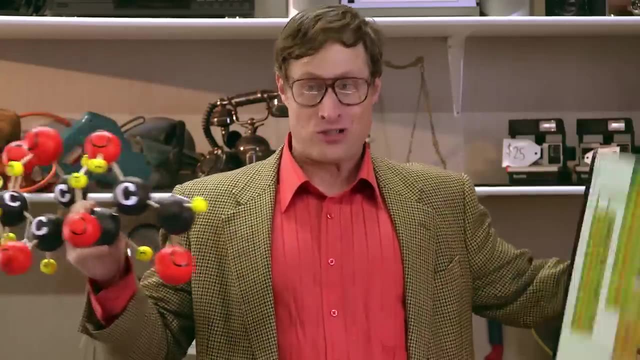 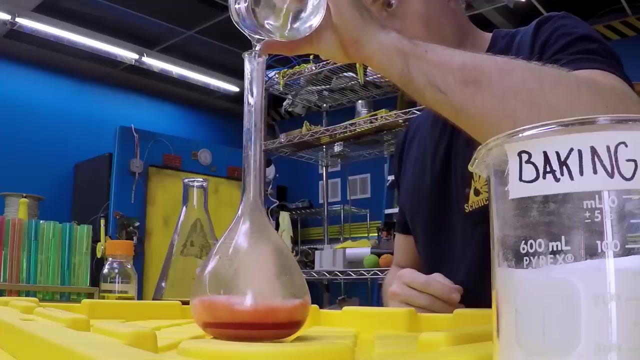 Hey, that's some. All matter in the universe is just the stuff on here combining into these. And now you know your chemicals: Mmm sugar. Let's take a closer look at what's going on when we mix vinegar and baking soda. 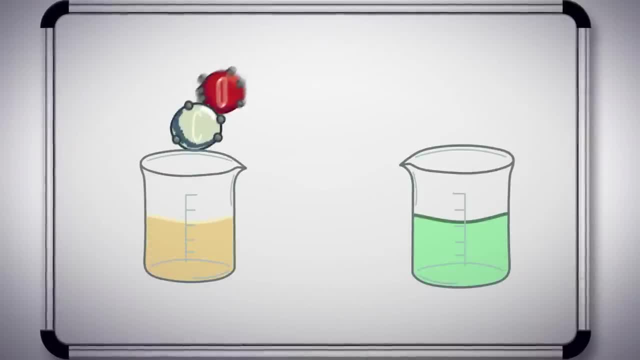 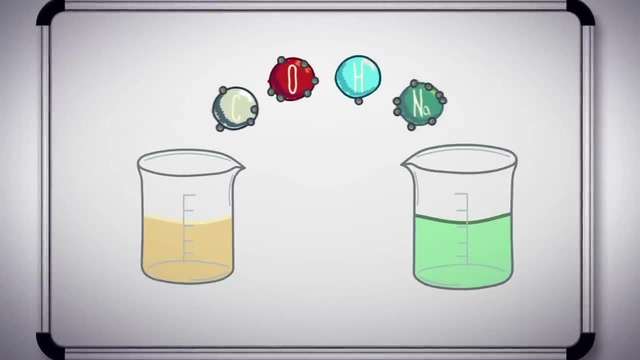 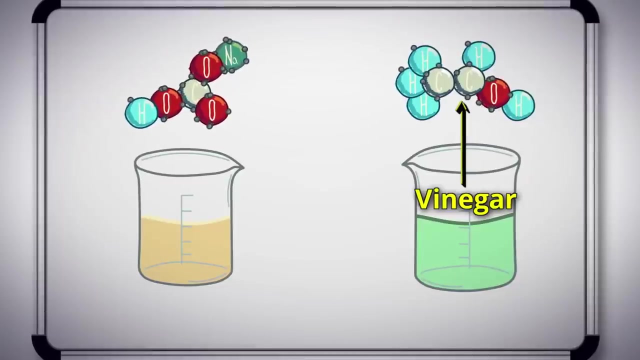 All chemicals are made of atoms. There's only four types in our reaction: Carbon, oxygen, hydrogen and sodium. When they go together like this, this is a molecule of vinegar or acetic acid, And this is a molecule of baking soda. 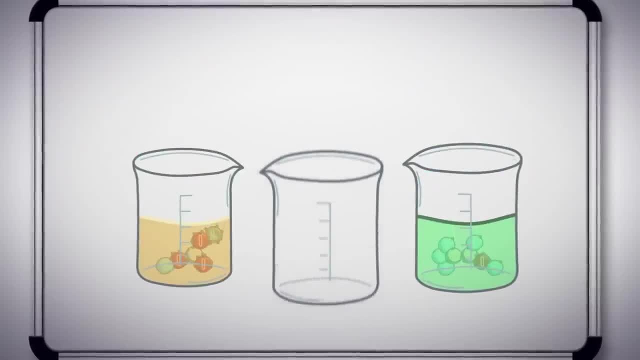 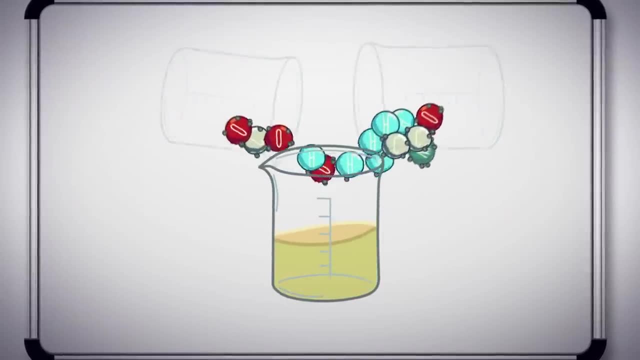 or sodium bicarbonate. When chemicals react, they switch atoms. That one goes there, this one goes over here, and then this one turns into this, and then what you end up with are new molecules. This one is called sodium acetate. 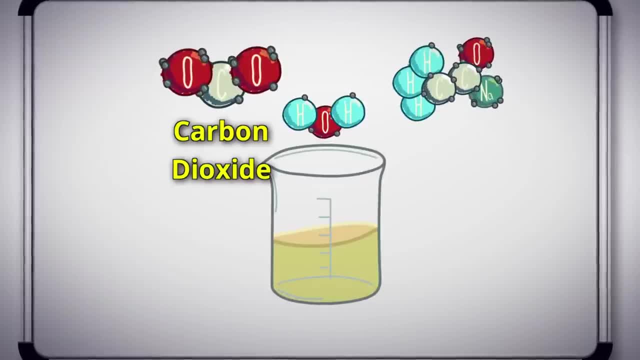 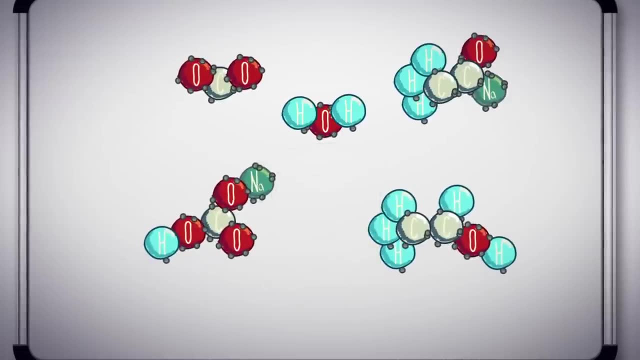 and this one is carbon dioxide gas, the gas you breathe out. And do you recognize this one Right? Water, H2O. Why all this happens gets complicated, but the sodium bicarbonate, the carbon dioxide and the sodium bicarbonate are connected. 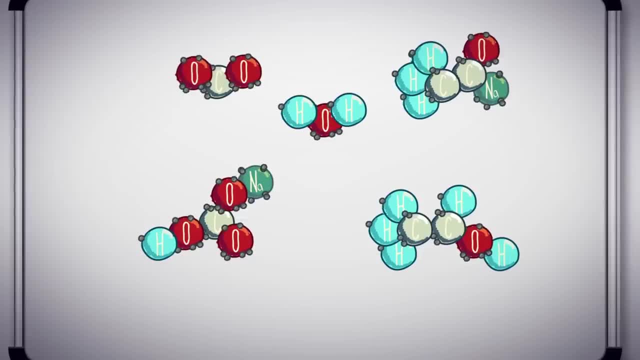 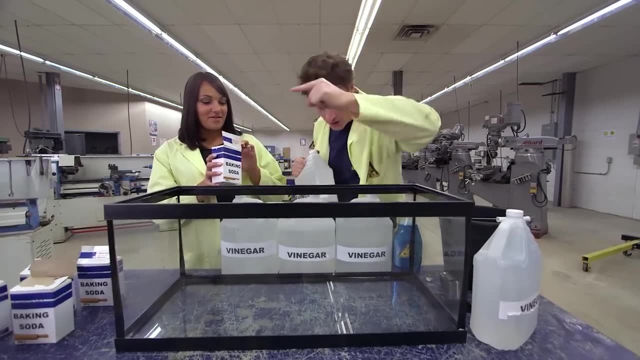 But the study of chemistry is all about how molecules are built and react with other molecules. All right, Talena, you ready? Yep, You're going to pour all your baking soda in the fish tank and I'm going to pour the vinegar into this bucket. 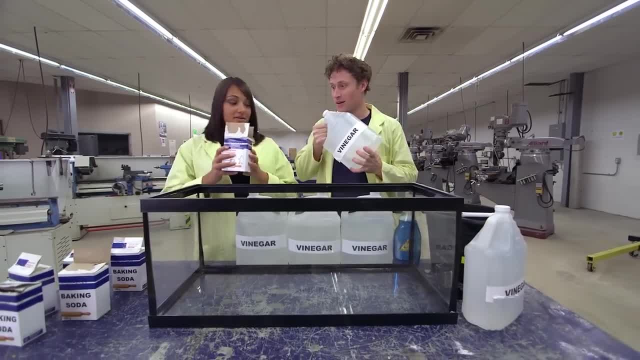 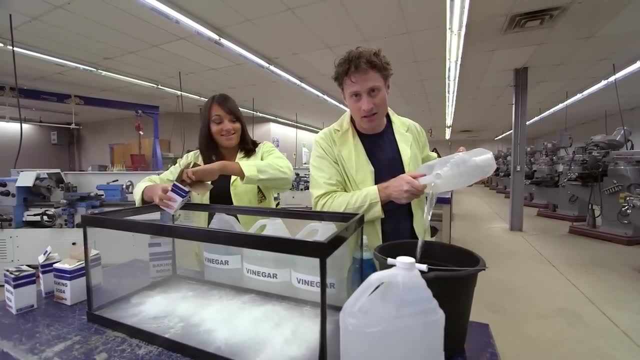 because you don't want to pour them together right away. Okay, you ready? Yep, Okay, go for it. When you're doing your PhD in chemistry, do you get to do stuff like this? Yeah, Really, I get reactions in the lab. 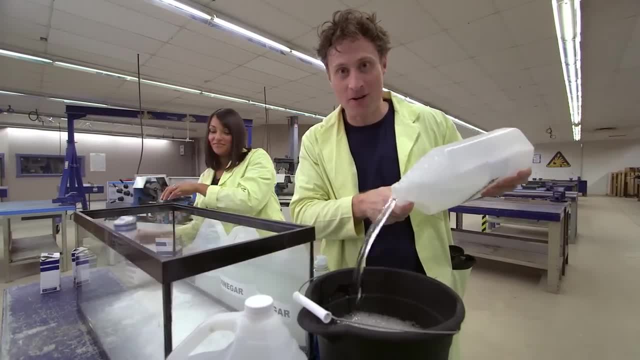 Oh, that's, I'm jealous. Have you ever done this much vinegar in baking soda in one time? I can't say I ever have. There you go. That's what I like to hear. I already put the soap in the bucket. 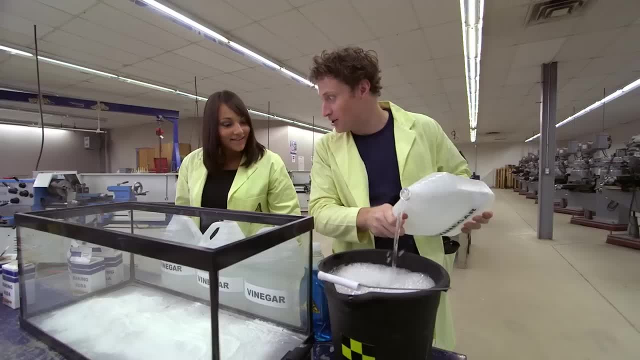 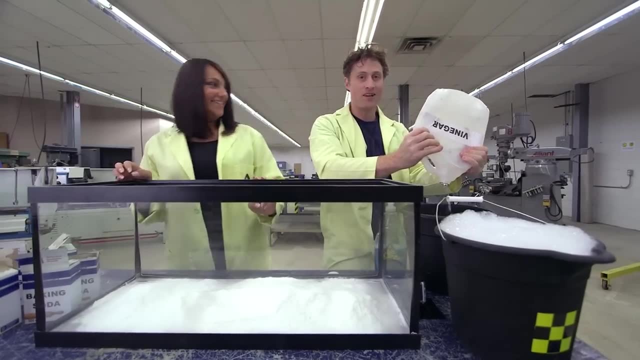 so it would mix with the vinegar when I poured it in. Are you done your baking soda already? I am. I'll pour faster, Oh faster. It smells vinegary, It smells vinegar. It makes me want french fries. Okay, Talena, you take this very full bucket. 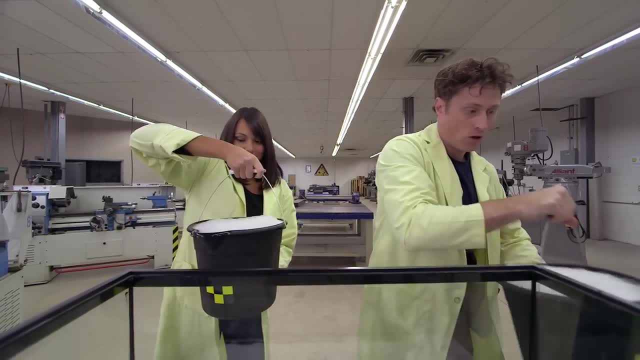 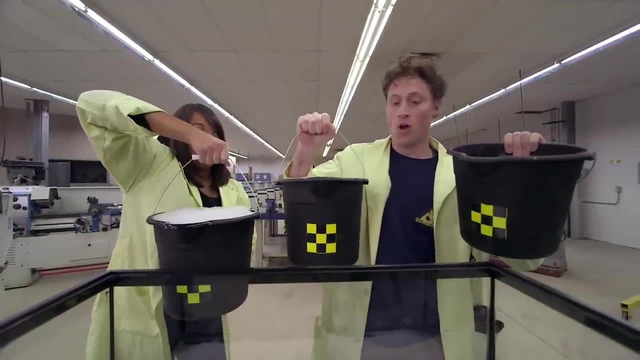 of vinegar and dish soap. Thank you, I'll take this one. Uh-oh, we still have our third bucket. Okay, I'm gonna. I'll do these both at the same time. Okay, Ready On the count of three? 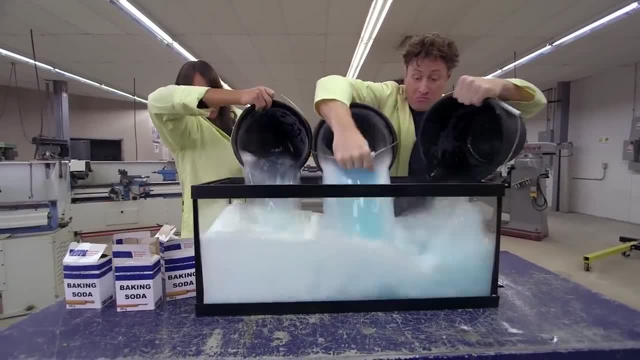 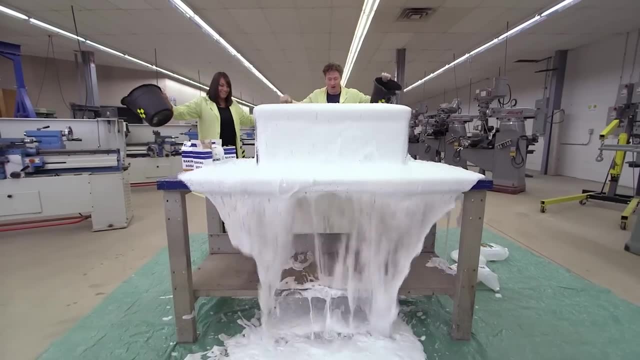 One, two, three, Whoa, Whoa, Whoa, Whoa, Whoa, Whoa. Okay, That's awesome. So the one thing it didn't do, it didn't shoot up in the air, though. 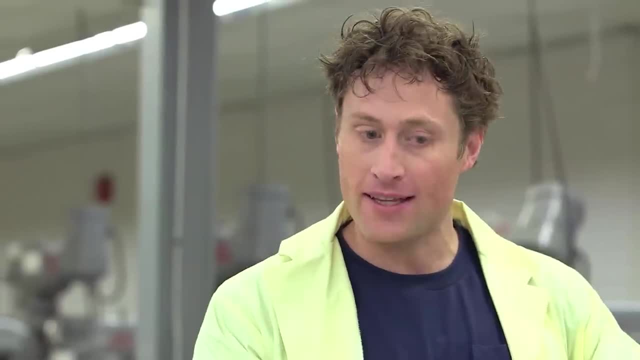 Yeah, it's because the top is quite open, so you would need to constrict it to the bottom of the bucket. Oh, okay, That's awesome. So the one thing it didn't do, it didn't shoot up in the air, though. 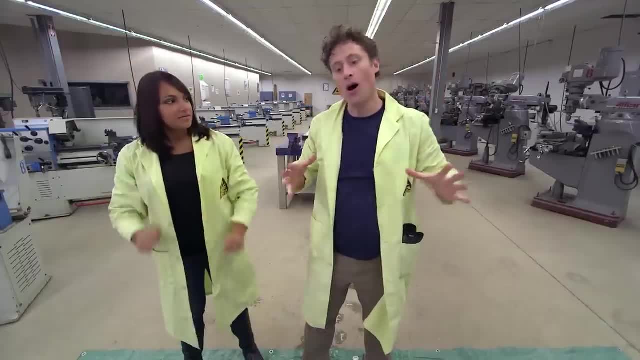 Yeah, it's because the top is quite open, so you would need to constrict it to get it to shoot up. Oh yeah, because we're using just sort of a square, a rectangular prism container. Mm-hmm, We should get something. 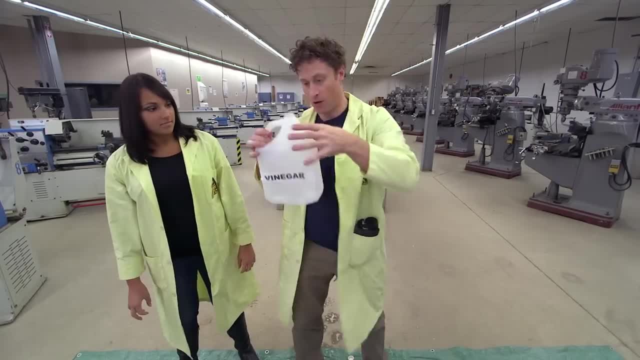 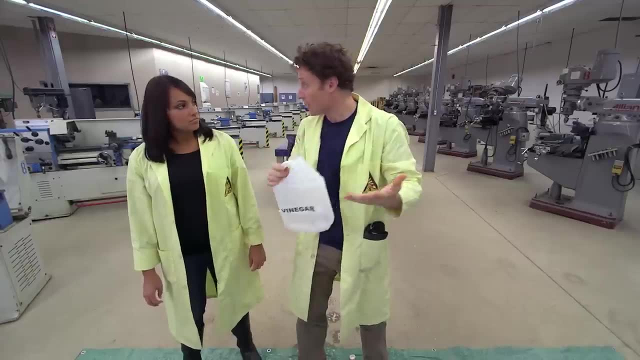 that's maybe something more like our vinegar bottle, right, Yeah, Because there's lots of space down here, but then it forces it into a tighter opening at the top there like a volcano. Yeah, And what else can we do to make it even more powerful? 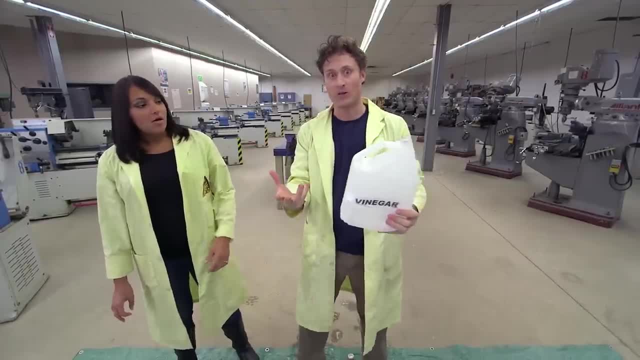 to max it out, Vinegar is only 5% acid. The rest is water, so you could try using 100%. So what kind of acid is vinegar? It's acetic acid. So what kind of acid is vinegar? 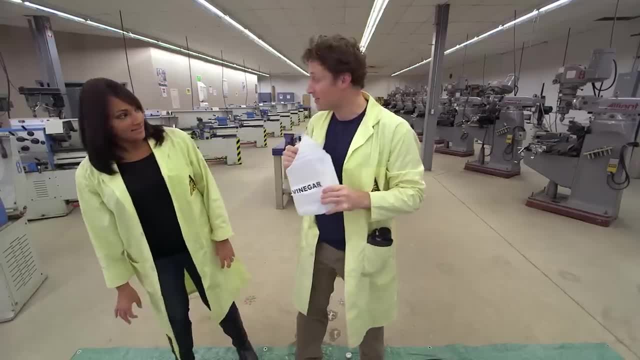 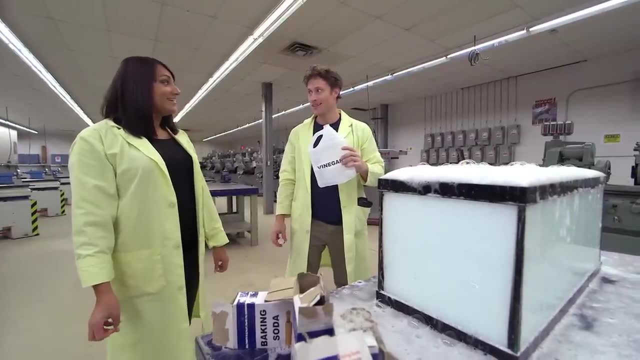 It's acetic acid. Okay, So vinegar is actually only 5% acetic acid, Yep and 95% water, So you can get 100% acetic acid. Yeah, Can you get 100% acetic acid. 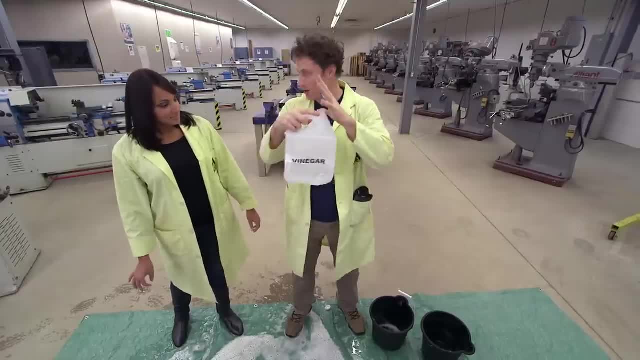 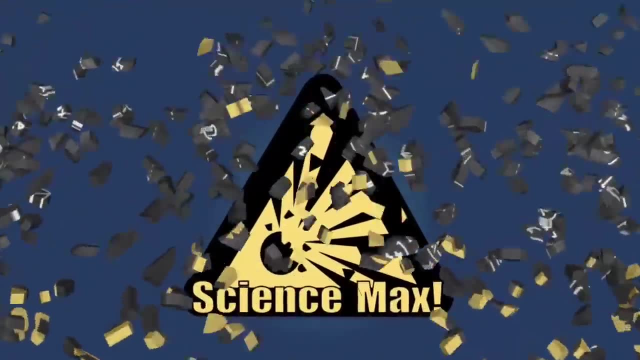 Yes, Awesome. Why don't we get a container that's sort of shaped like a funnel, like a volcano? Yep and 100% acetic acid and we'll do it again. Sounds good, All right, let's do it. 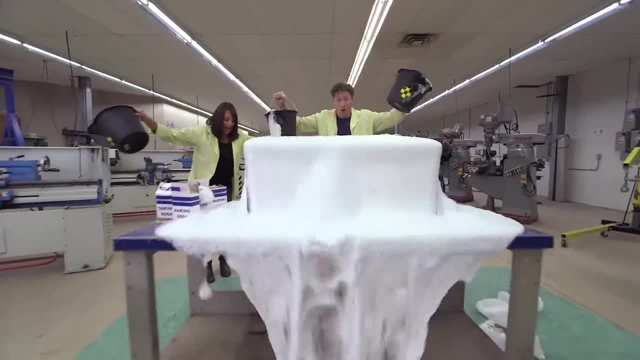 Our vinegar and baking soda reaction went pretty well, but now we're going to try it with a much stronger type of the same kind of acid you find in vinegar. Oh yeah, So vinegar and baking soda went pretty well, but now we're going. 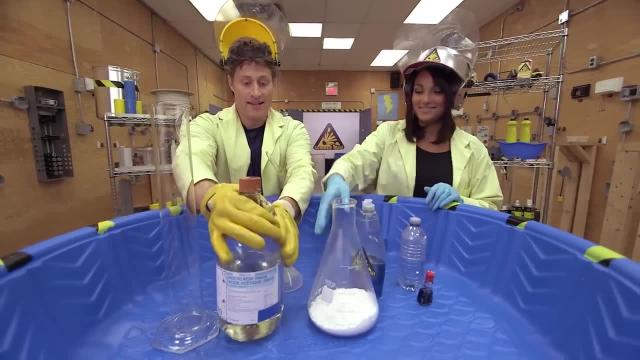 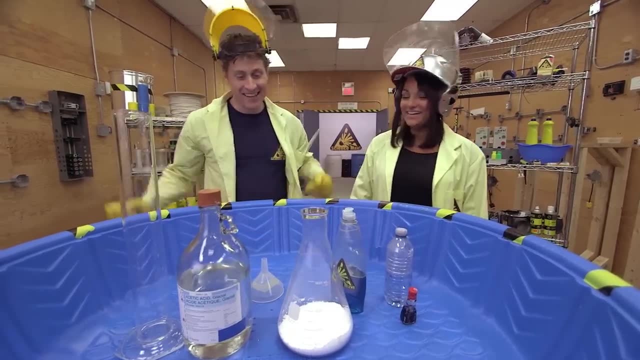 to be carefully putting this down And watch out for the baking soda. You never know when it'll get out. And well, I guess that's just baking soda. huh, Yeah, that's pretty safe. Yeah, okay, good. 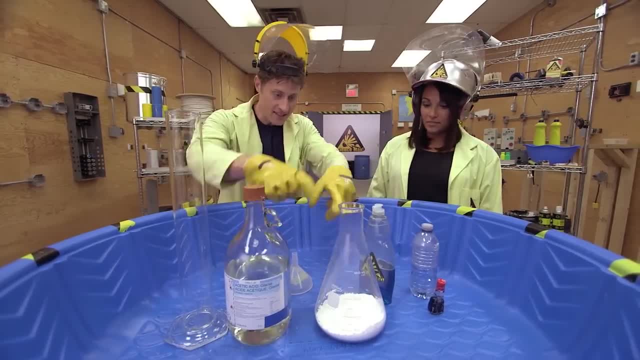 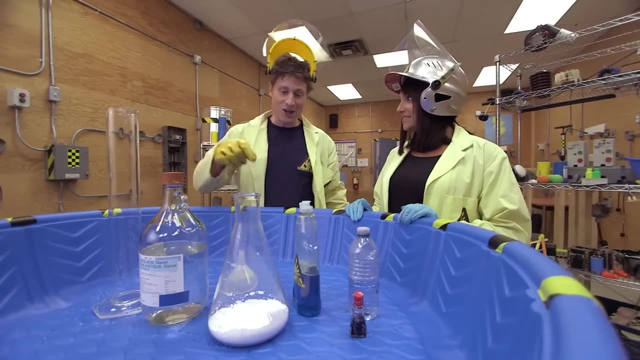 So this is baking soda vinegar. volcano version two. We have this differently shaped glass. What do you call this? again, That's an Erlenmeyer glass. Why is it called that? It's actually named after a scientist. Did he look like that? 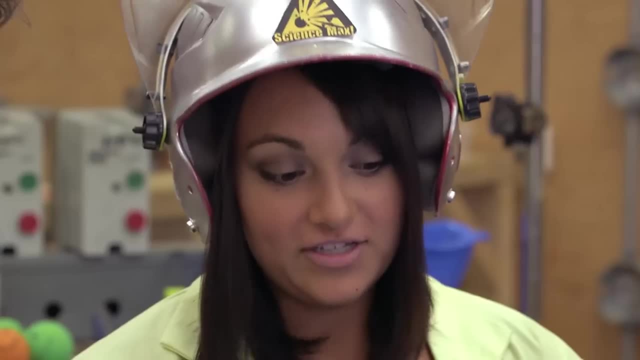 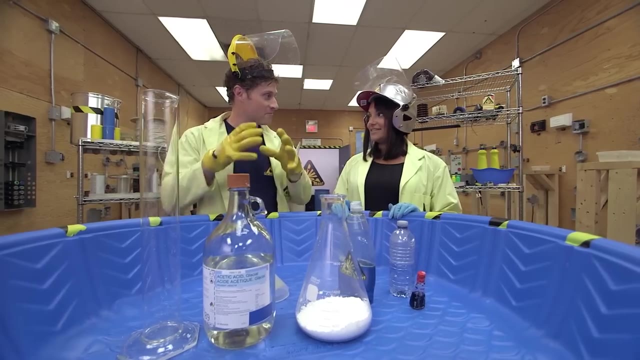 Was he sort of shaped like this? No, No, Was he just a good chemist, Good scientist, and I think he designed it. I want to have a glass named after you. You're a good chemist and design a glass. 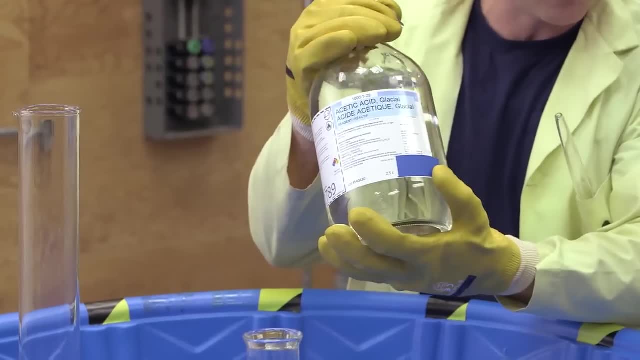 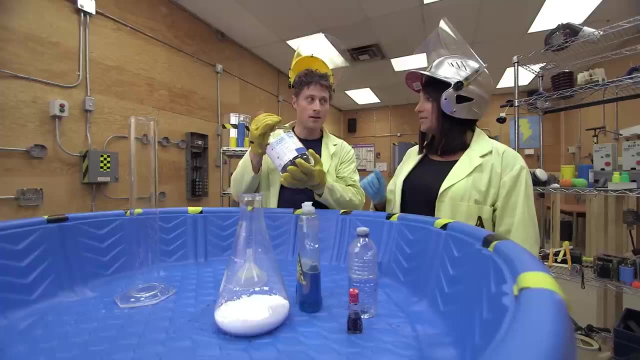 I want to make a fill beaker. So this is 100% acetic acid, Yep. And what's the difference between this and vinegar? Vinegar has 5% of this and 95% water, but this is 100%. 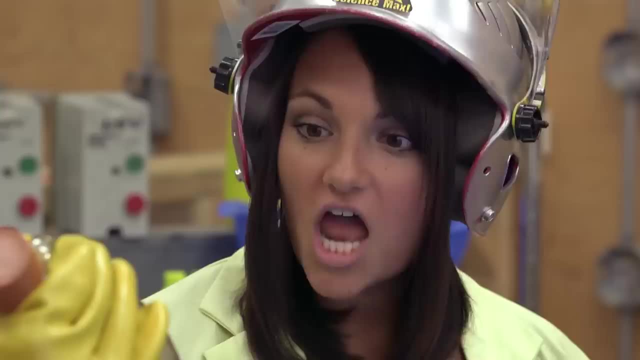 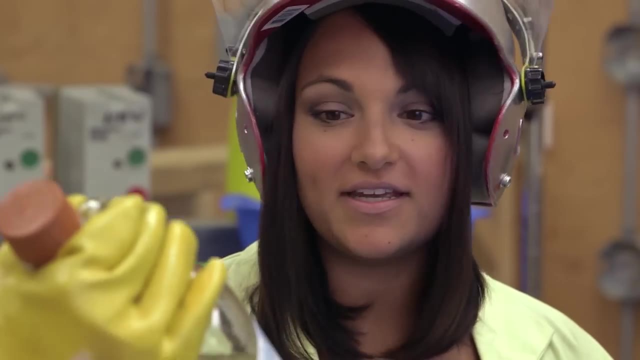 so it's much stronger, Much stronger. Can you put this on your french fries? No, I wouldn't be putting it on your french fries. No, As chemicals go, how dangerous is this? It's not too dangerous, but you definitely don't. 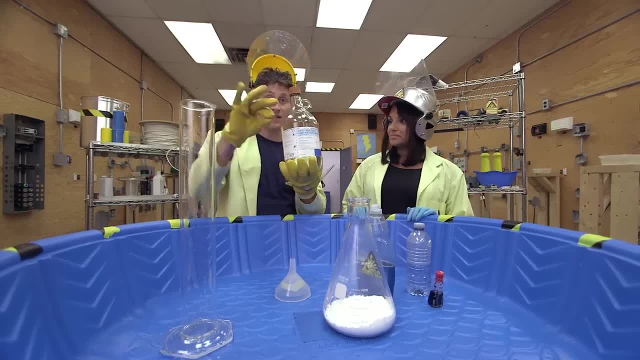 want to be breathing it in and you don't want to be eating it. You don't want to be wearing these fancy pants and gloves, So what I'm going to do is I'm going to pour the acetic acid in this. 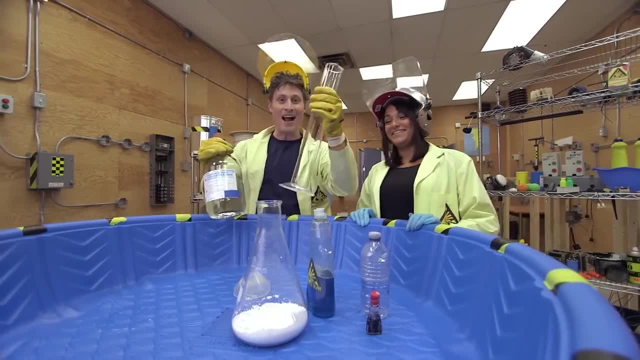 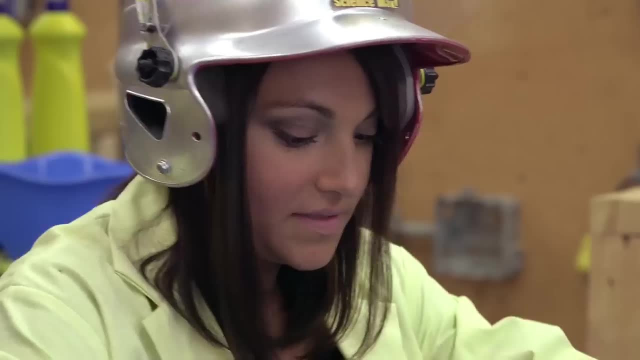 What's this called? That is a graduated cylinder, Because it finished school, So it graduated. Now you're going to mix water and food coloring and soap all together, Yep, And pour it into there. It'll help dissolve some of the baking soda. 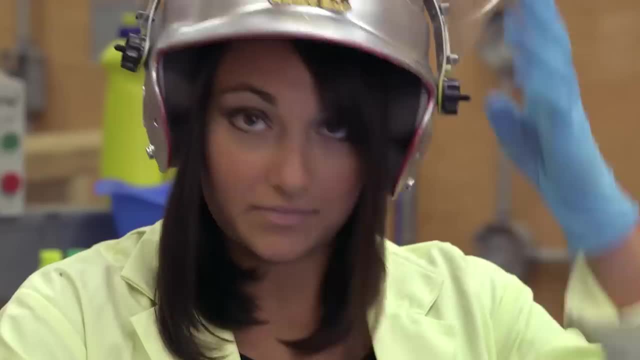 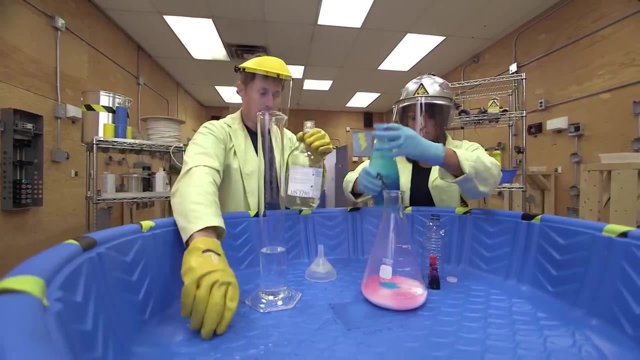 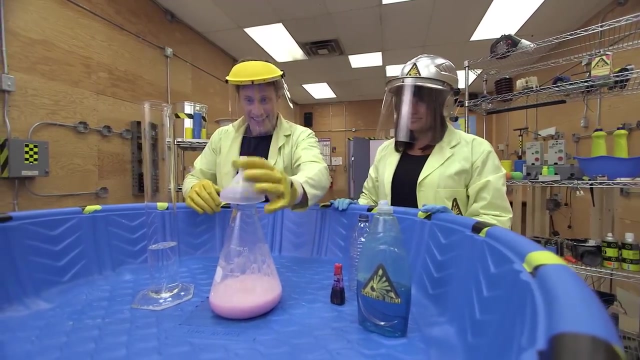 so hopefully it'll react better with the acid. Sounds good. Face protection: Oh, All right, that's good. And now, when we do it, I want to add the funnel at the end to like accentuate the concentration of. 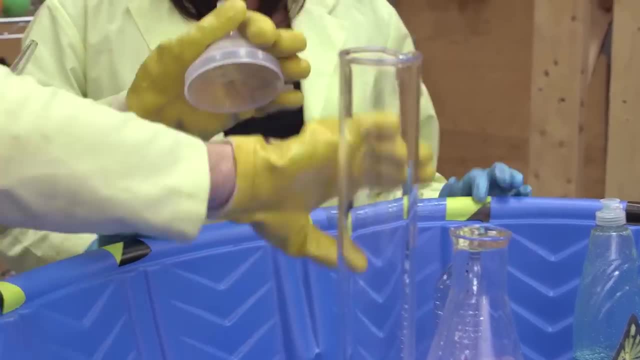 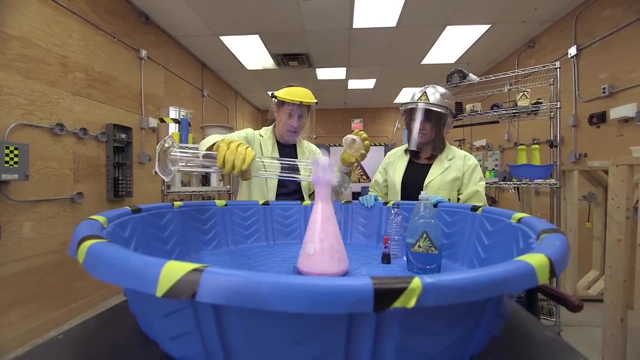 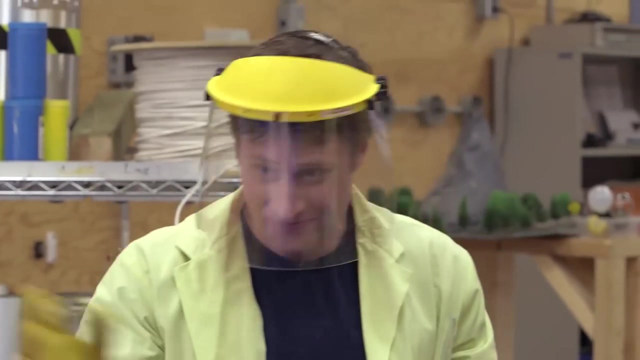 But I don't know if it's going to go so fast that I won't be able to get it in there, but we'll try it. We'll try it. Vinegar, baking soda- volcano version two. Whoo, Good thing you got the mask. 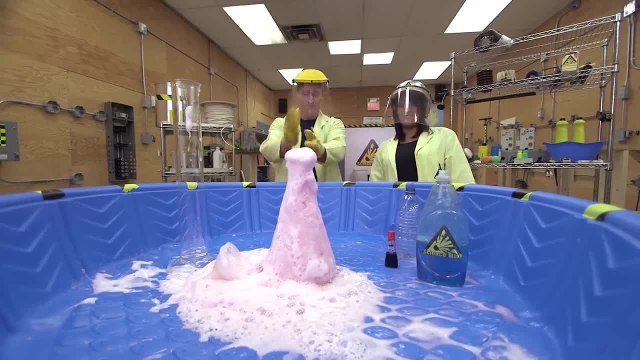 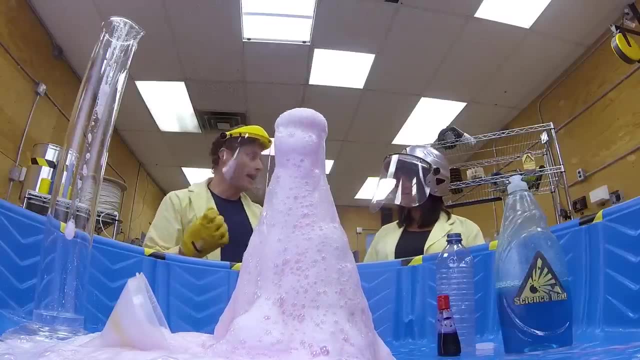 It smells a lot like vinegar. It's really strong. Oh, That was pretty good, But what can we do to make it even bigger? Well, you could try using a different chemical reaction. Ooh, okay, Like what? The decomposition? 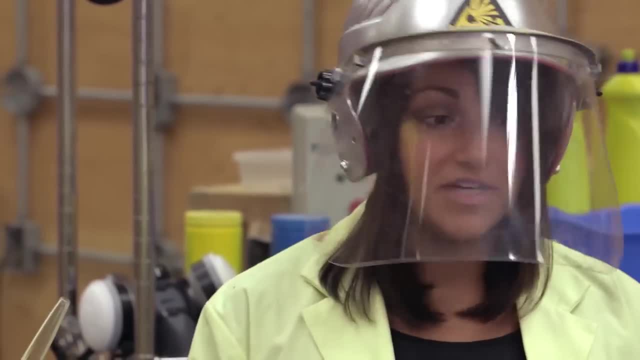 of hydrogen peroxide produces oxygen gas, and so that one's pretty vigorous if you use a catalyst. So we want something that makes a lot of gas, so that it makes a lot of bubbles when you put the soap in it. Yep, Great, let's do it. 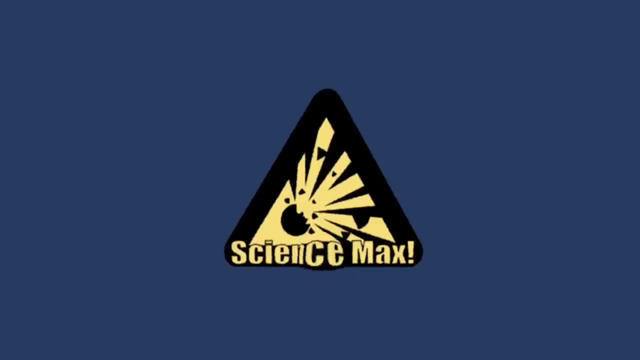 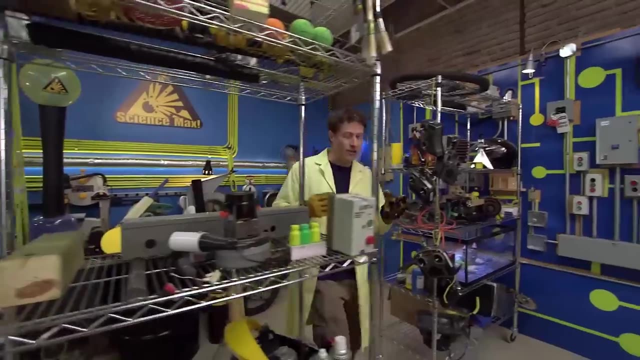 And the sooner you leave that smell, the better, I think, for my taste. Today we're combining two different chemicals to create a reaction. Sometimes chemicals can combine in a way that makes them very different from how they started out, For example. 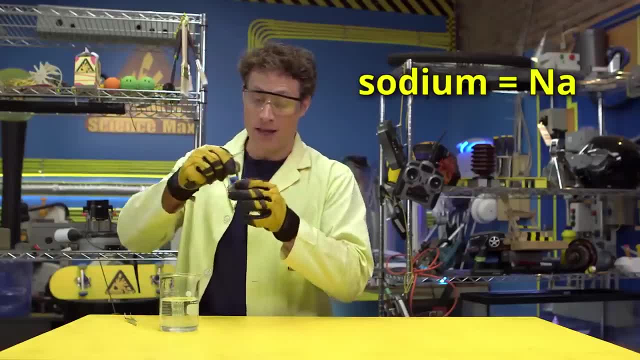 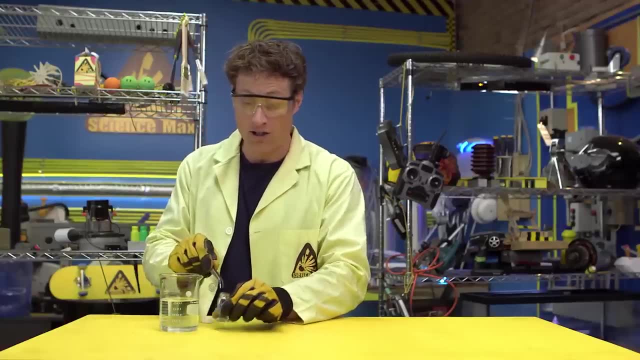 this is sodium or Na on the periodic table. Now the sodium tablets are in mineral oil because sodium reacts very strongly with water, even the water in the air or especially the water in my skin. Watch what happens when I drop a sodium tablet. 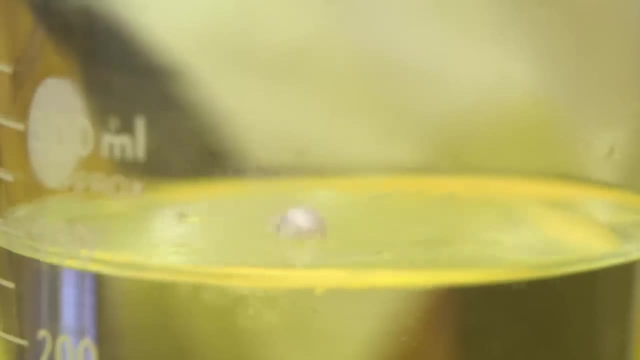 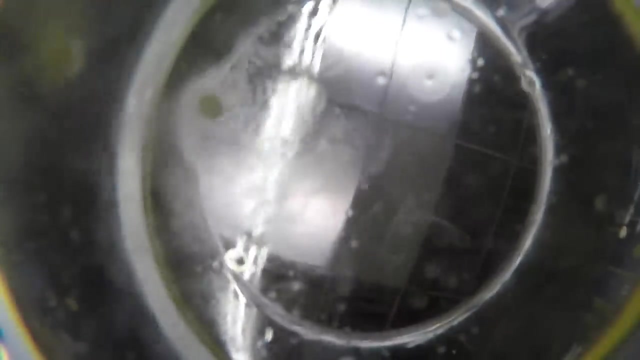 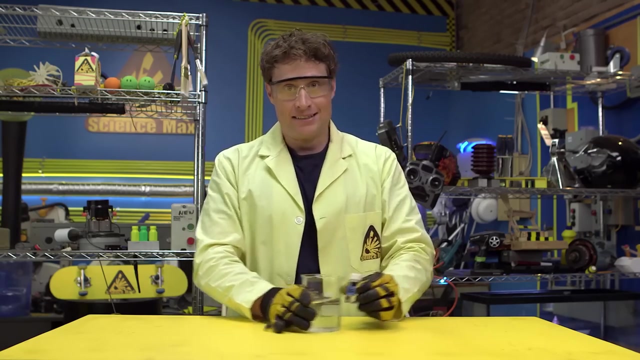 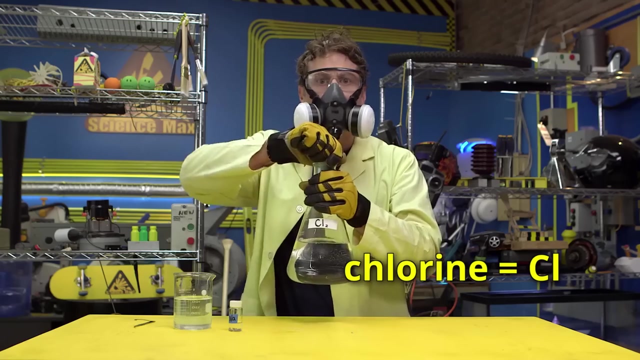 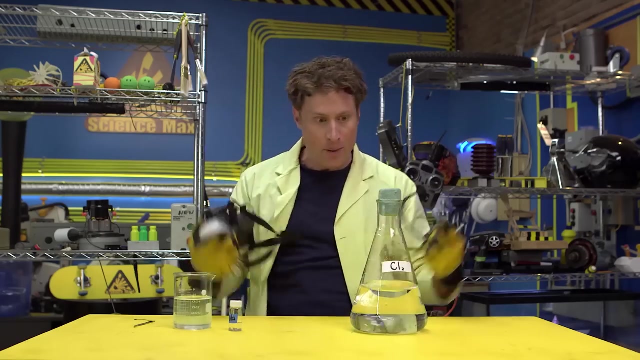 into this beaker of water, Very cool and very dangerous. And this is chlorine or Cl on the periodic table. Chlorine gas is very poisonous, So. So what happens if we combine these two deadly substances? Do we create some sort 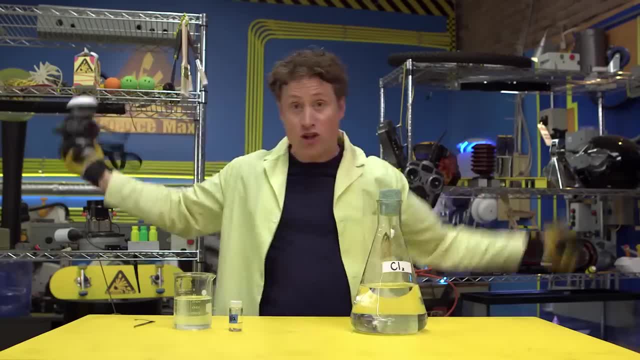 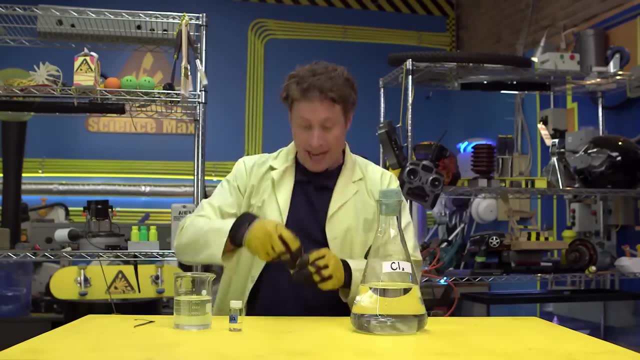 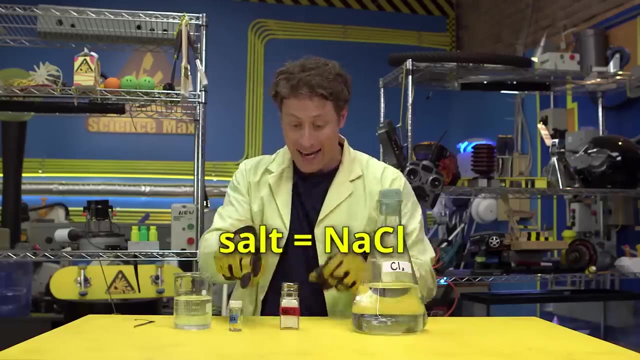 of super poison, something more deadly than anything else known to science, that causes fear and chaos in chemistry labs all over the land. No, We create salt, Good old normal table salt. These two substances combine to make NaCl salt, something completely. 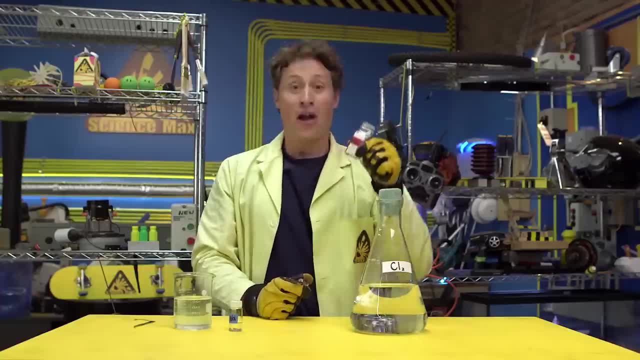 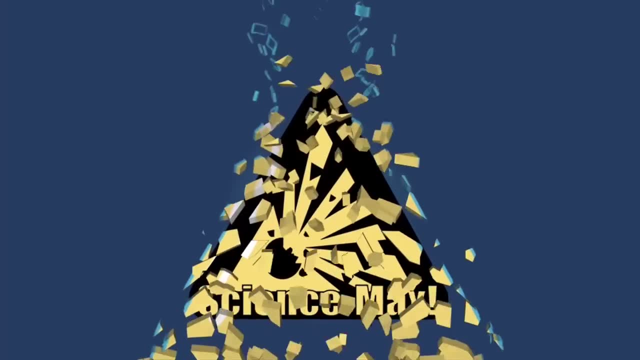 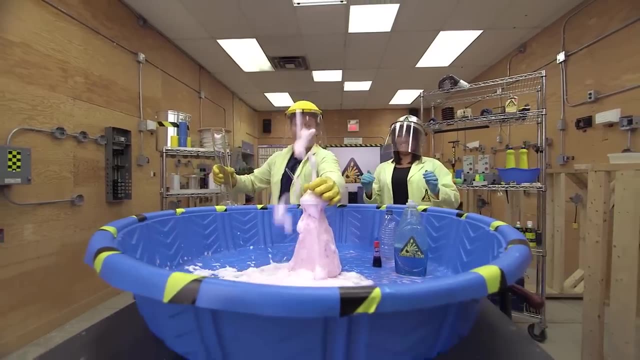 and totally safe Chemistry. Oh Oh, We've gone from vinegar and baking soda to 100% acetic acid in baking soda, and now we're doing the vinegar and baking soda volcano version three. No longer vinegar and baking soda, Nope. 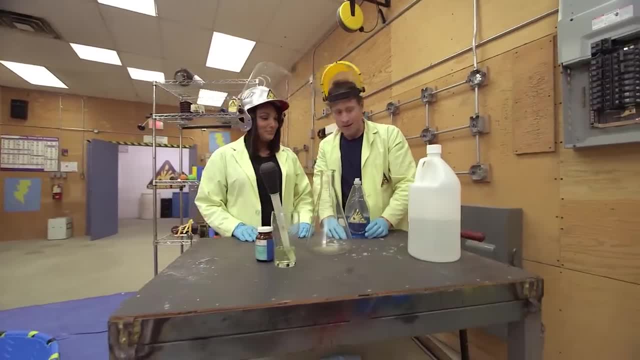 What are we using this time? So here we have some hydrogen peroxide. Oh, that's the stuff you use at home to put on a cut right. Yeah, but the stuff at home is only 3%. This one's 30.. 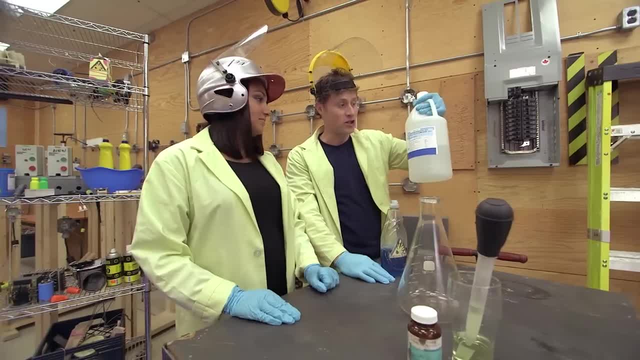 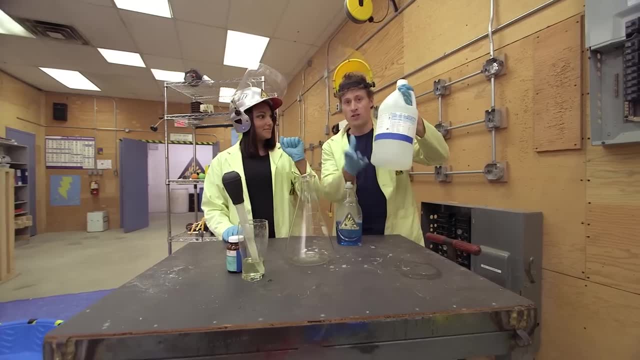 So much, much stronger, Much, Ten times stronger, Yes, And is this more dangerous? It's definitely corrosive, so it's definitely more dangerous. It's definitely corrosive, so wear your gloves. Corrosive means it could eat your skin. 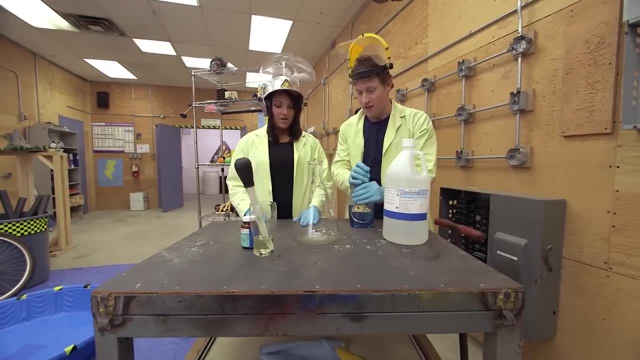 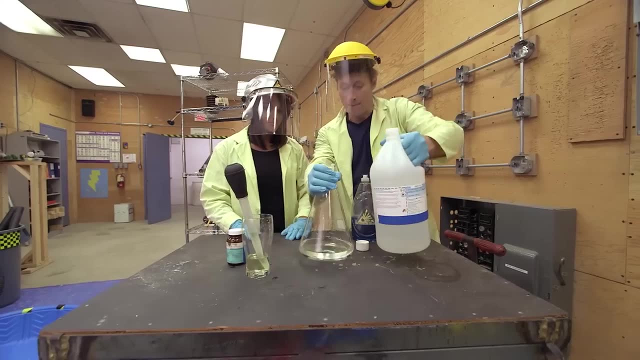 It can burn your skin a little bit, Which is why we are wearing gloves and blast shields. What's going to mix with this? So here we have some potassium iodide, which is a salt, and it's mixed in with some water. 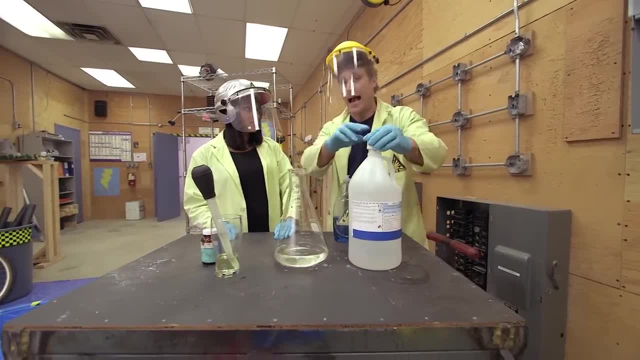 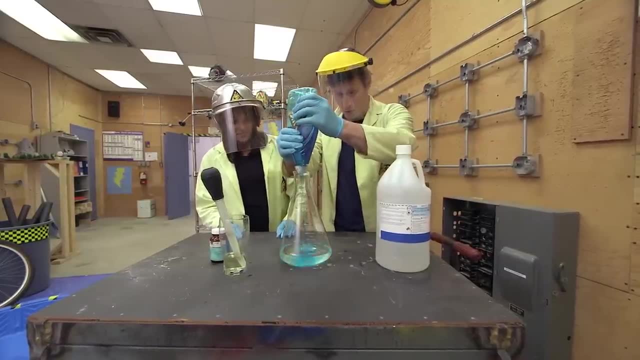 The most important part of this reaction is the fact that it creates gas, Oxygen gas, Which makes bubbles when you put in dish soap, right Yep? So one big squirt of dish soap like that, Mix it up And now we go over. 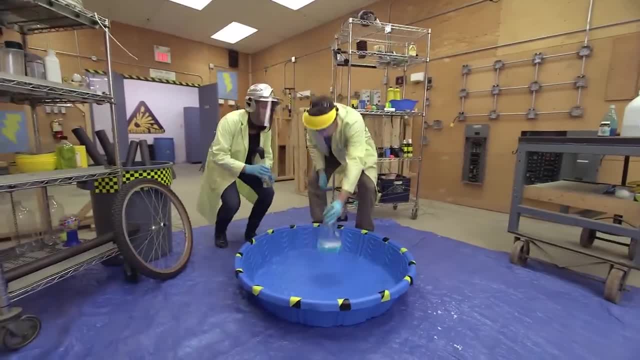 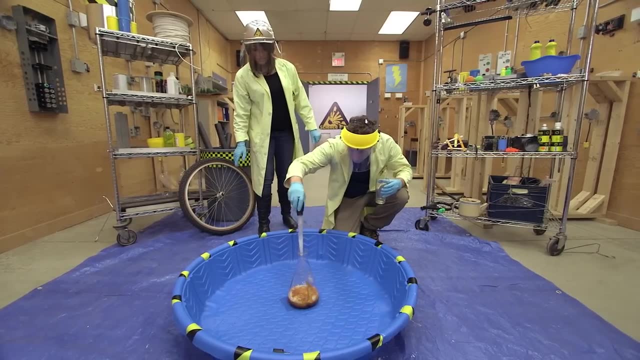 to the blast zone. That's plenty, All right. Now that's a reaction. It looks like there's steam coming off here. Why is that happening? Well, it is an exothermic reaction, so heat is being generated as the reaction proceeds. 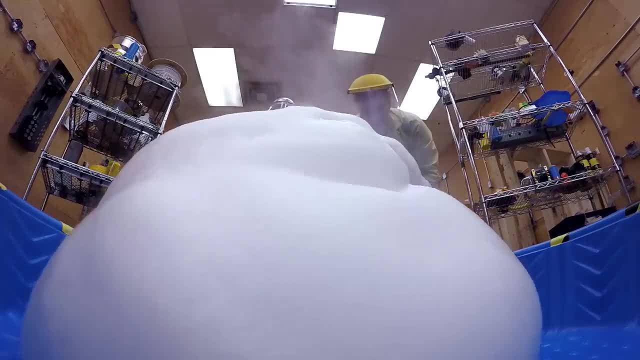 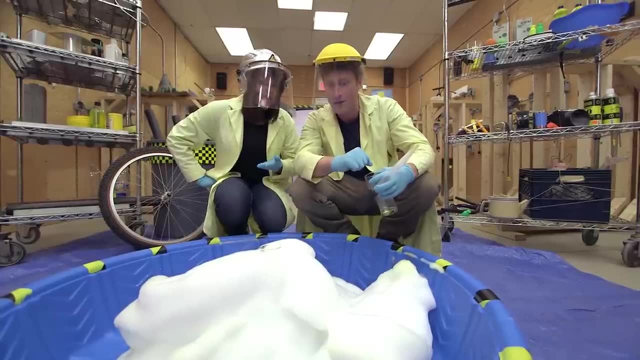 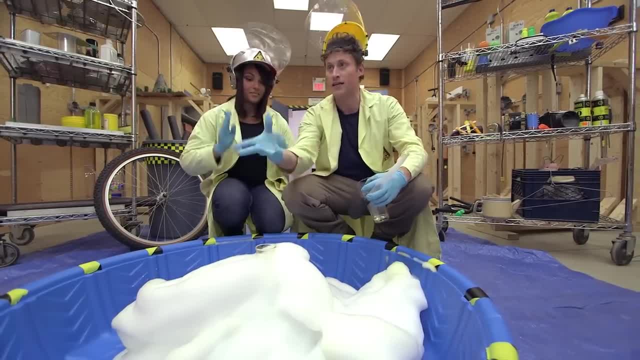 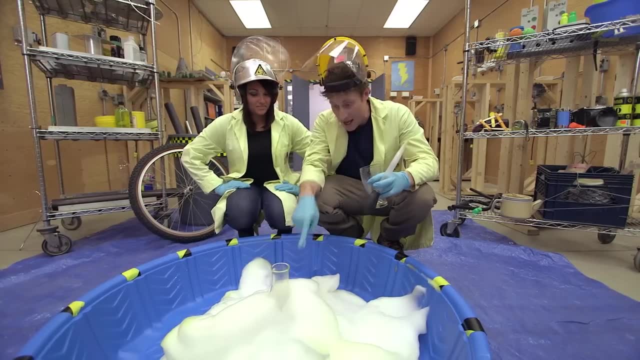 different. It's a little bit different. What's being released, What's the gas that's coming off here? So it's oxygen gas that's being produced. Oxygen, Ah. What we want to do is make this even bigger, but first, 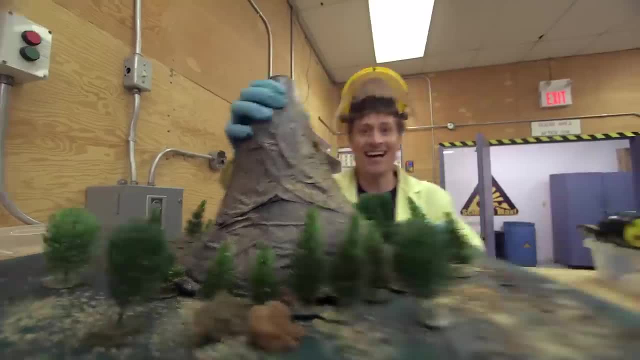 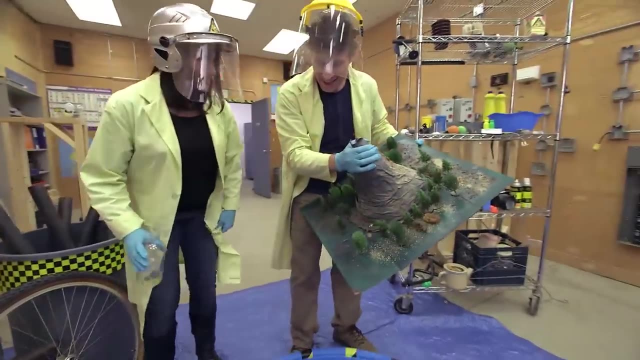 can we do it again? Sure, Because I have an idea. Hold on, I think we should repurpose our old volcano. What do you think Sounds like a good idea? Okay, So if we put it over here, All right. 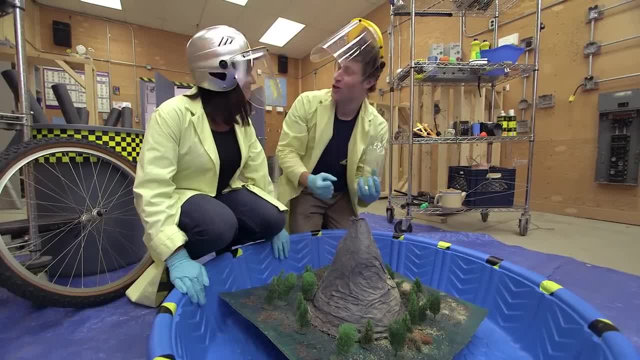 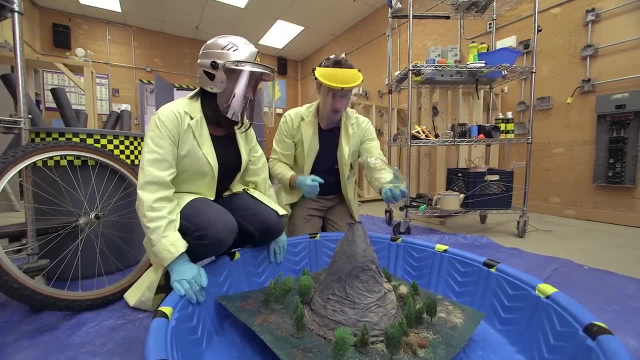 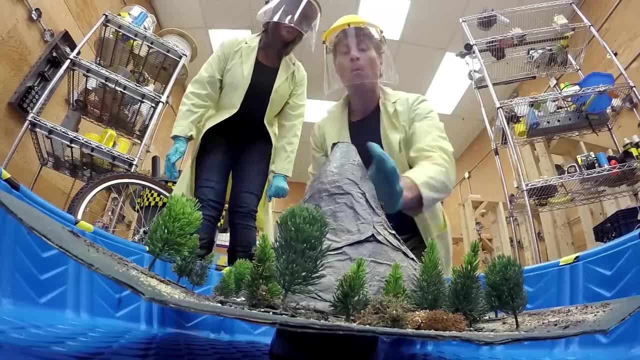 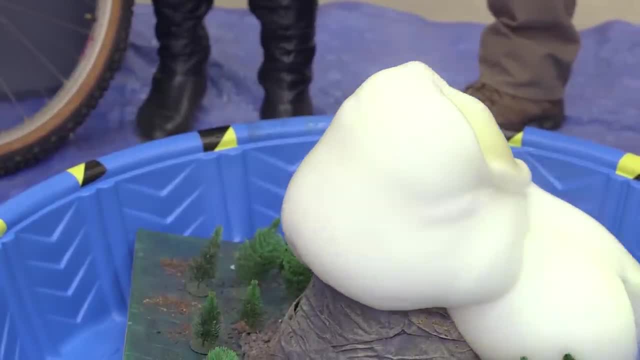 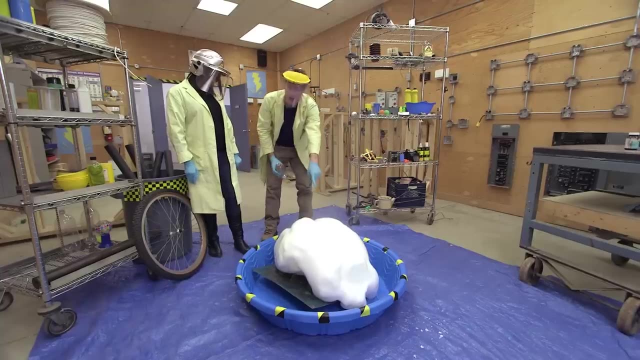 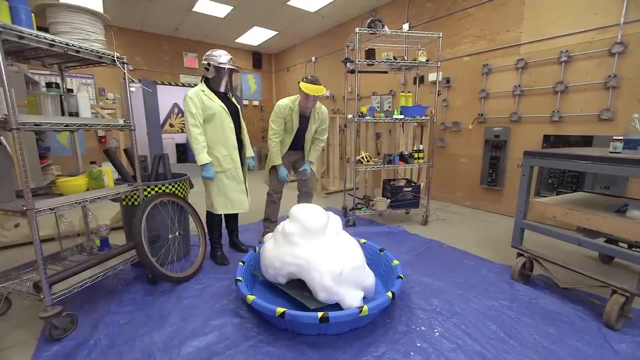 Here we go. Whoa, Look at that, Ha ha, ha, ha ha ha. Look at that. Now that is a big volcano eruption Just covered the town. That is completely yes. That town is going to be very clean because it's. 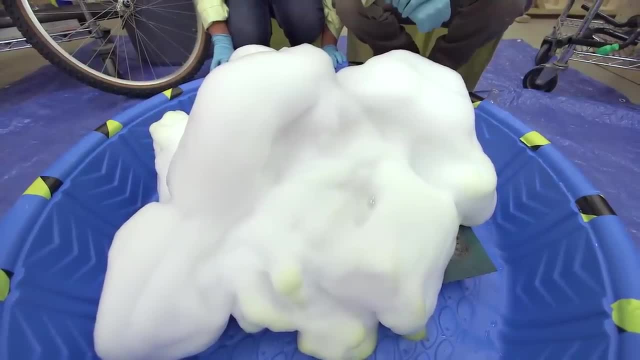 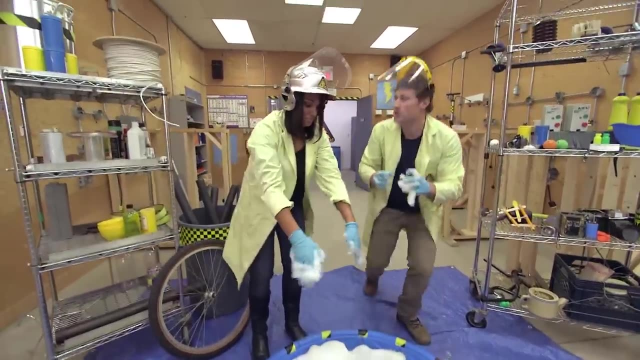 all soap bubbles. It's the cleanest volcano this side of Science, Maxaville. So I still think we can do this bigger, though, right, I agree. Oh, I know What if we use some sort of a tube, like maybe one of these, right? 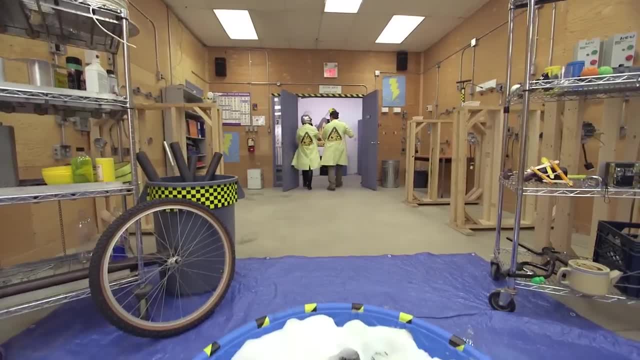 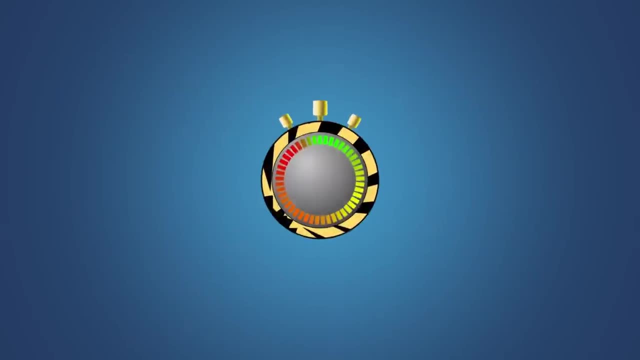 And then we attach it to like an air compressor. I think you'd get some height, Yeah, and we go aside The atom in 60 seconds. The atom is the smallest unit in a chemical element. Atoms are made of three parts. 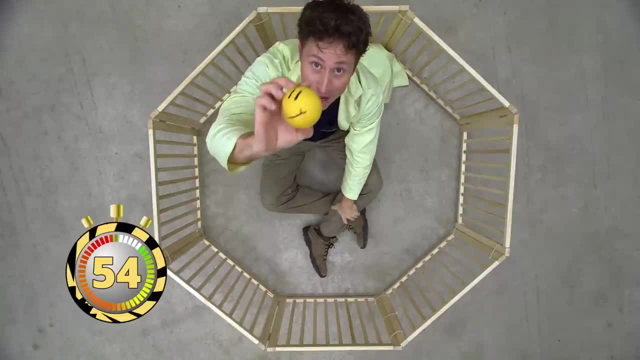 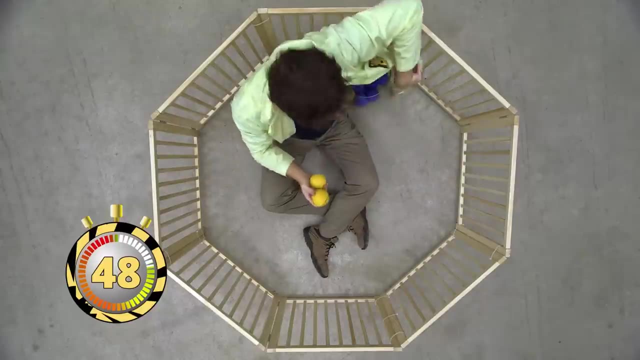 Part number one are these guys protons. They have a positive charge. The number of protons determines the element. One is hydrogen, two is helium, three is lithium, and so on. The protons sit in the middle here, which is called the nucleus. 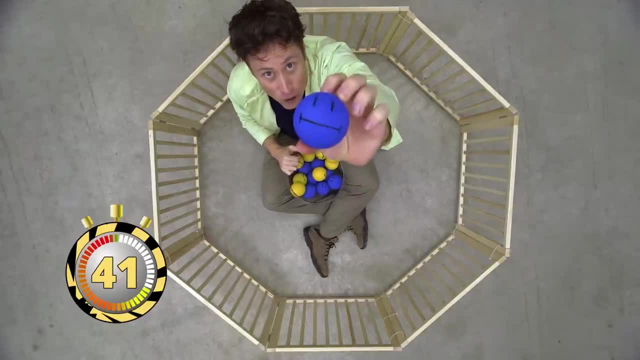 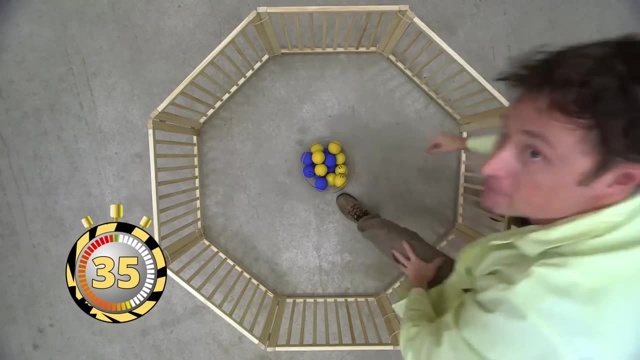 They sit in here with part number two, these guys. They're neutrons and they have a neutral charge. Now I've got eight protons and eight neutrons in this nucleus, making this an atom of oxygen Orbiting around the nucleus. are these tiny guys? 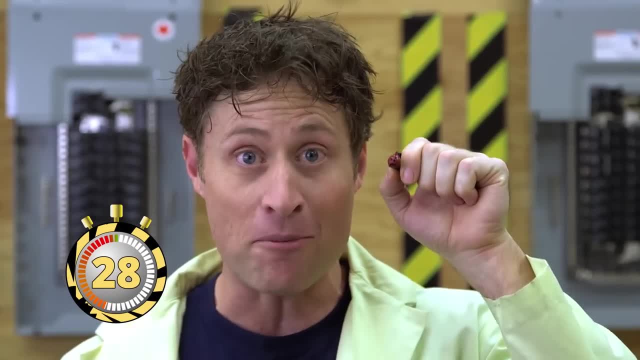 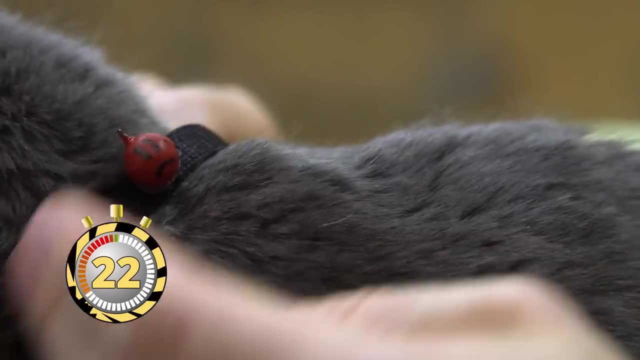 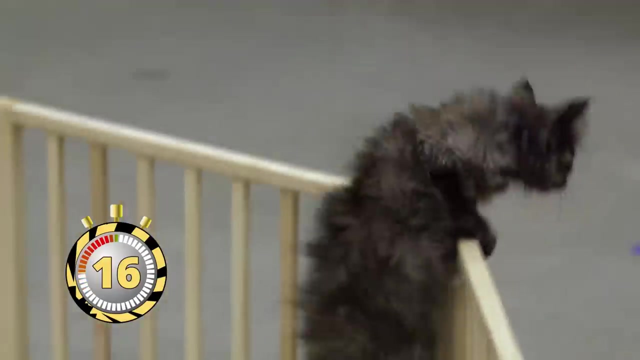 They're electrons and they have a negative charge. I will demonstrate using kittens. Kittens are perfect because, just like electrons, kittens are really small And, just like electrons, kittens move around randomly. You never know where they're going to be. 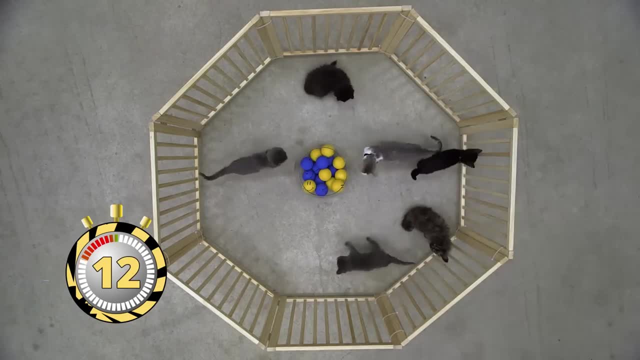 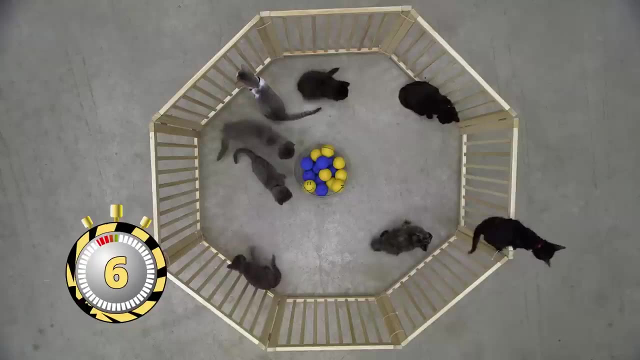 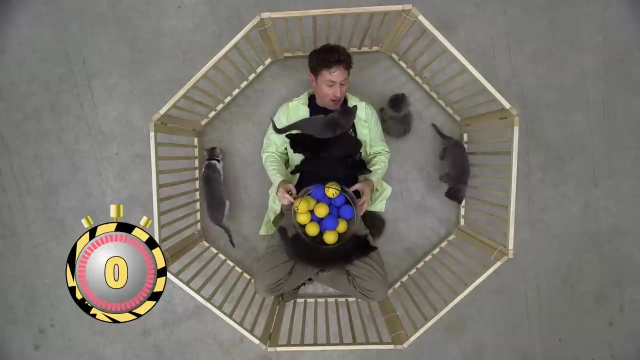 But an oxygen atom should have eight kittens or electrons somewhere inside. These kittens are constantly escaping, but guess what That happens with electrons too. There you go The atom: a nucleus of protons and neutrons surrounded by randomly moving electrons. 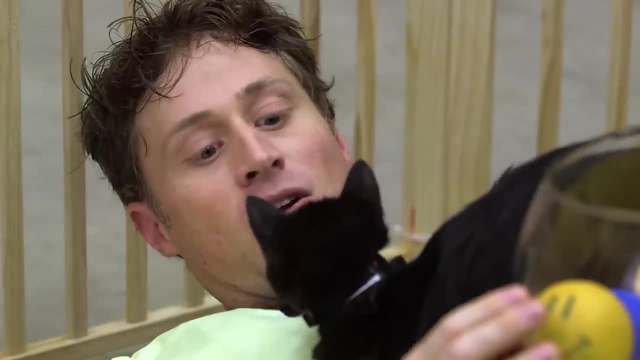 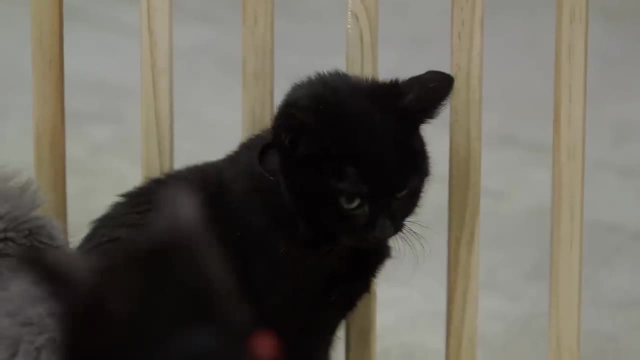 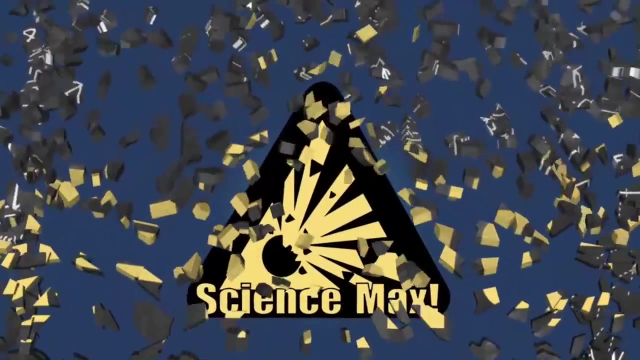 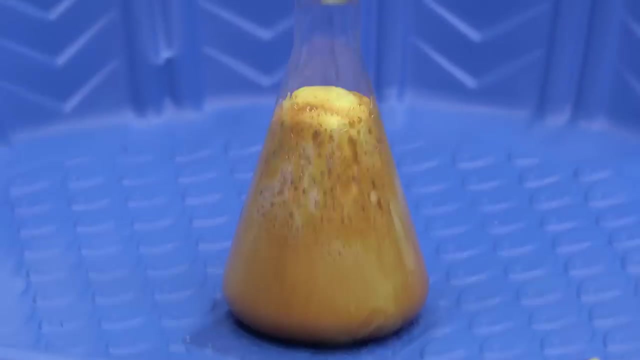 Cutest science ever. How do you guys feel, Did you learn something? Huh, Paws up. Who learned something? Hm Talena and I have made a bunch of chemical reactions, but in our quest to max things out, we've got a new plan. 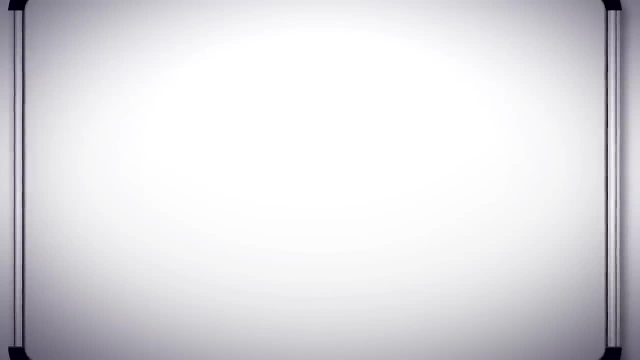 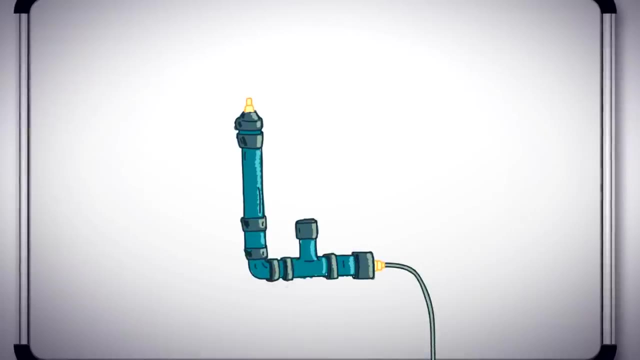 Whoa. Hydrogen peroxide and potassium iodide create gas. One way to max out the reaction is to contain the gas in something like a tube. We're going to put the hydrogen peroxide in the tube first, Then we're going to put in the potassium iodide in the top. 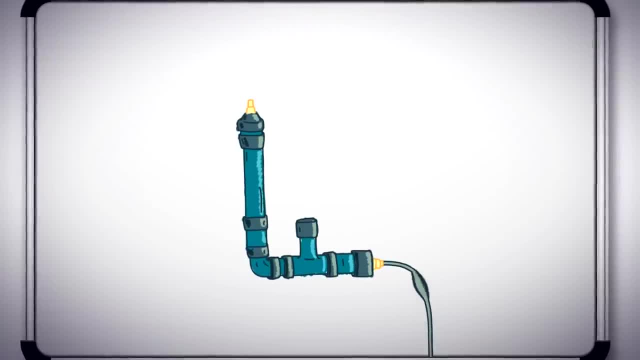 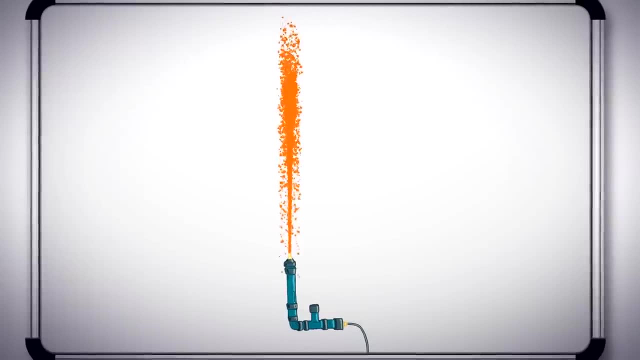 through a one-way valve. Then we're going to pressurize the container. When it finally reacts, it will shoot up through the valve and we'll see how high we can get our stream of bubbles to go. But be warned: capping anything and not letting it escape. 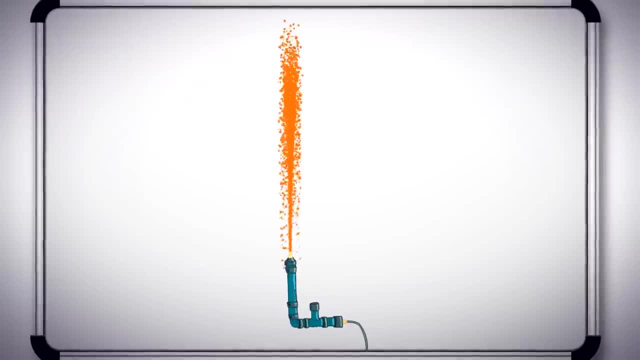 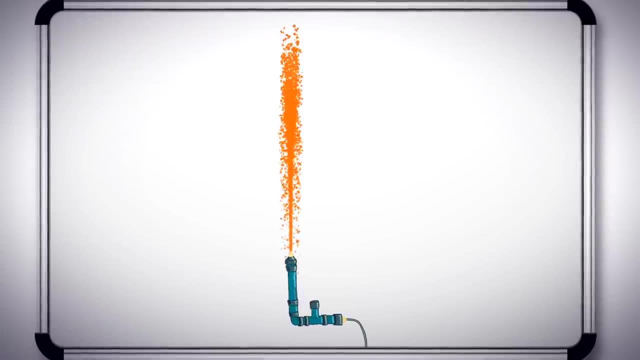 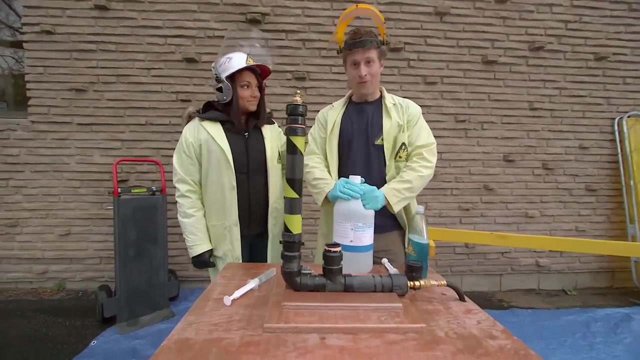 is never a good idea, So we've got a release valve to make sure things work out. This is one of those experiments that's definitely on the list of don't try this at home. Vinegar, baking soda, volcano version four, Hydrogen peroxide, potassium iodide. 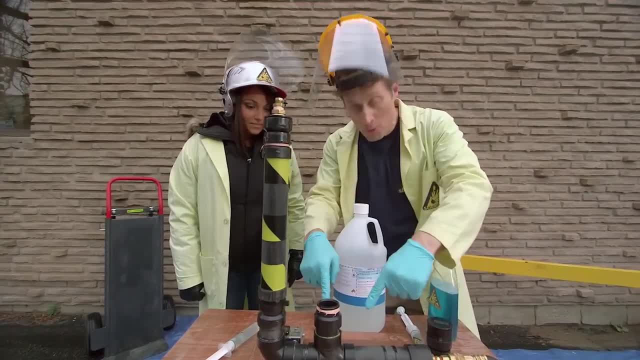 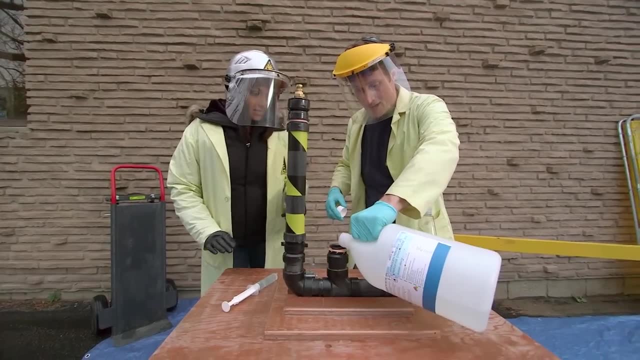 And what we're going to do this time is we're going to put it in this tube hydrogen peroxide. hydrogen peroxide goes in here And we've got. Talena, do you have the potassium iodide in syringes? 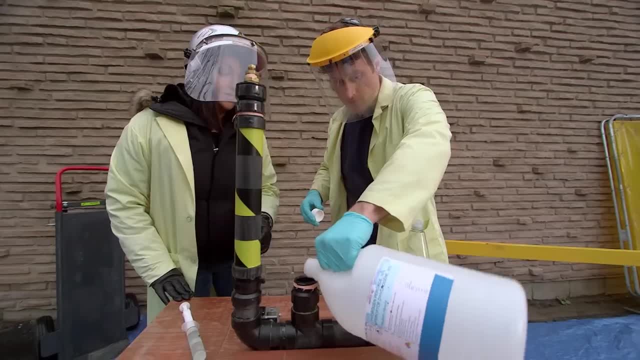 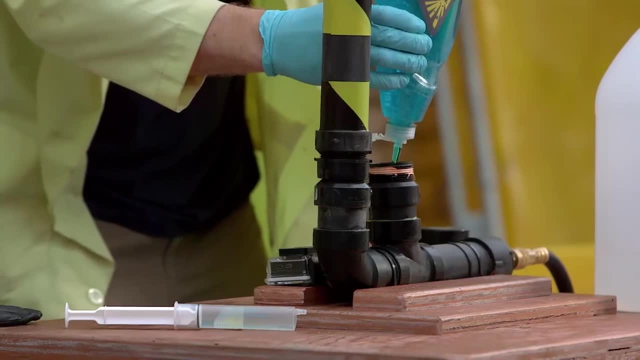 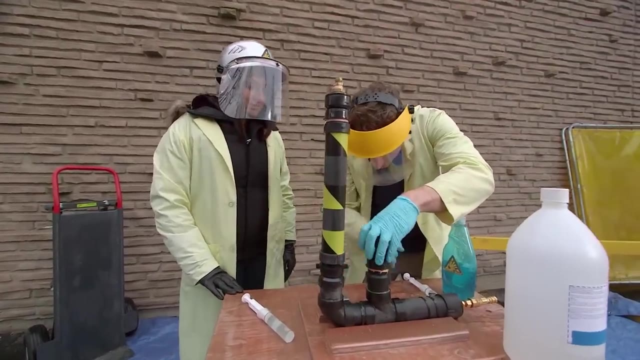 Yeah, two syringes full. Two syringes full, That's about there is good, And then soap, good amount of soap in there, And so what we're going to do is we're going to close this off and tighten it up. 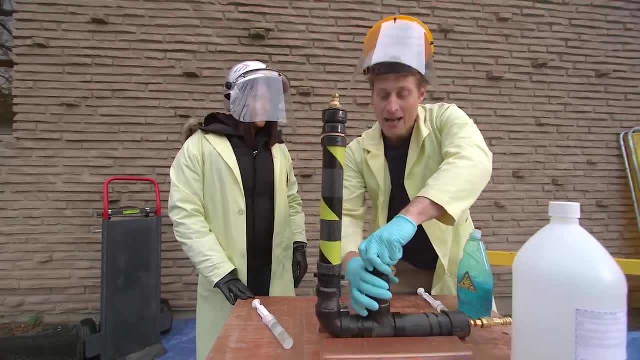 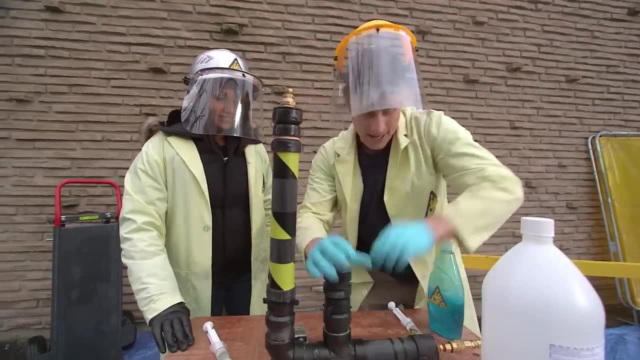 And then we're going to pressurize the whole system, And then we're going to add the potassium iodide And it's going to be spectacular, we hope. OK, that's on tight. This is all good putting this down here.